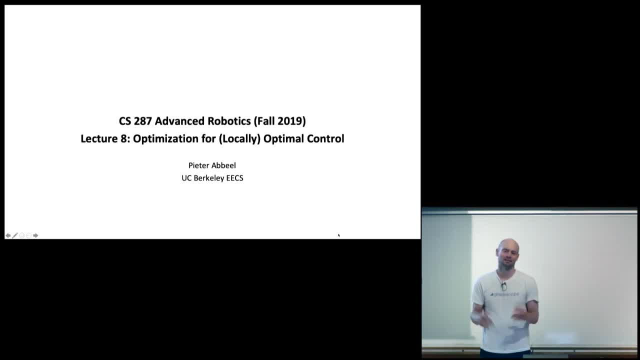 Tuesday: Igor is well. he's done the most advanced nonlinear optimization for optimal control of anybody in the world. So it's really exciting to have him come lecture here and share kind of his best expertise in the world about how this can be done, Kind of the highest end version. 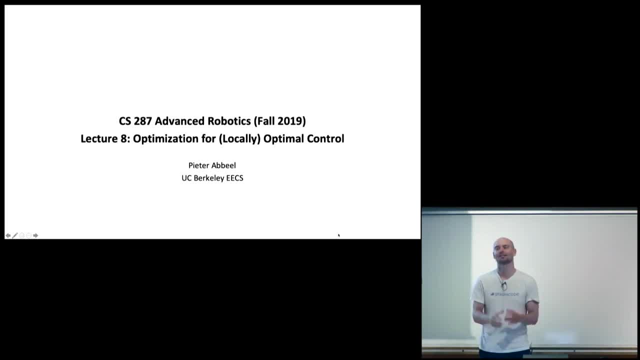 is something called contact invariant optimization, And that's one of the main things he'll cover on Tuesday. Let's see Any questions about logistics. Okay, Then let's get started. So I got a few things still to wrap up on constraint optimization. The first half of lecture will be on that. Let's 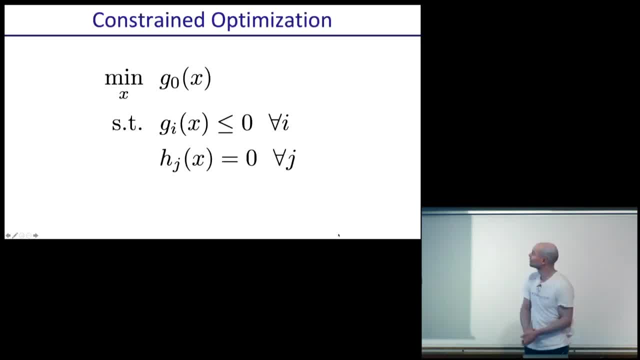 do a quick recap of what we looked at. Constraint optimization looked at this type of problem: Minimize some objective functions Subject to some functions being smaller than zero, which defines a region in the space where you're allowed to be, And then subject to some other functions equal to zero, which defines a very narrow. 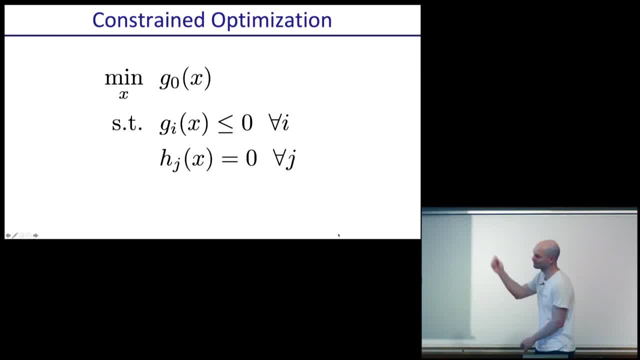 sliver of region in the space where you're allowed to be for each of those equations, Then the main formulation we saw was something called penalty formulation, And what it looked like is this. So let me get a pointer. So here's the original problem, And we knew already how to solve unconstrained optimization. 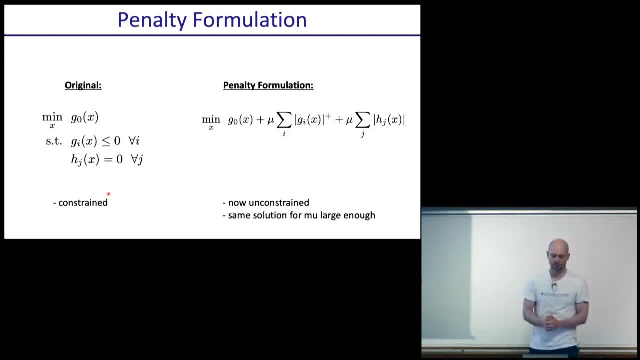 problems. Now, how do we use that to solve constraint optimization problems? Well, we introduced a penalty formulation, the original objective plus some coefficient mu times. what is really the sum of the constraints. And these constraints said that the value of G, of i over x, had to be negative. 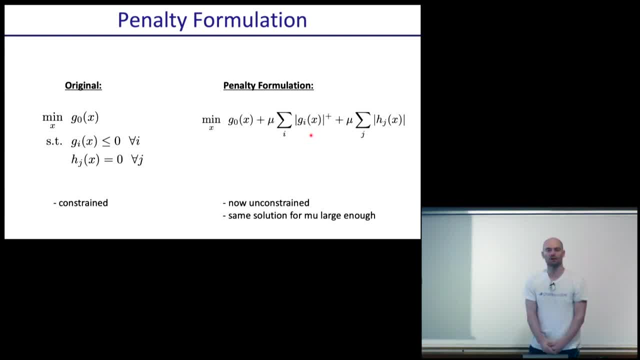 or zero And we see, we sum in the positive part of that. So if they're negative it doesn't contribute to the objective, But if it's positive it retains its value. That's what that absolute value with the plus means. 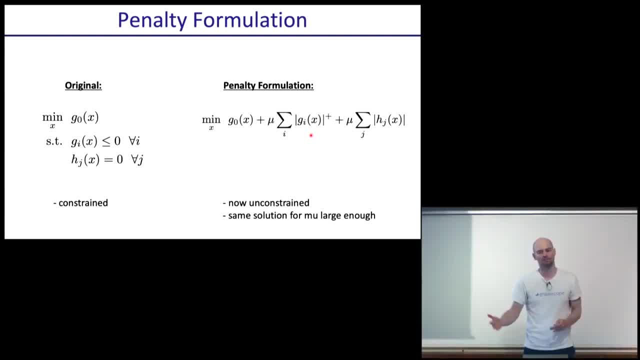 And it contributes to the objective. We try to minimize. so it's a bad thing. When it's positive, we get penalized. Same thing here. h, j of x is supposed to be zero. If it is zero, it does not contribute to the objective. 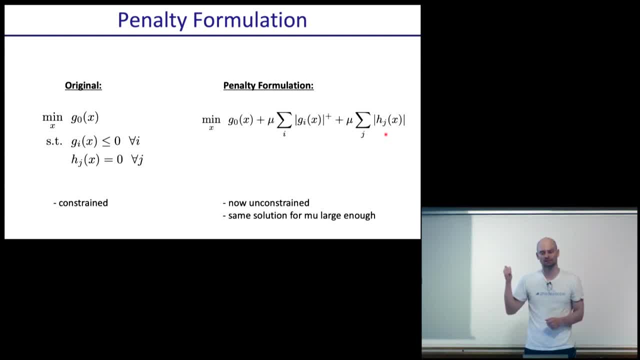 That's good. If it's not, zero positively contributes to the objective. Now there's a trade off between these constraint terms and the original objective, And so if mu is a small value, you might find an x that is actually not satisfying the constraints. 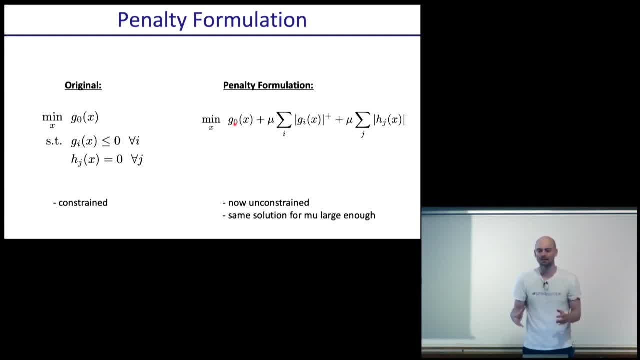 because it can do better on the objective. by violating the constraints It'll be penalized. but not enough to get the constraints satisfied. And what will happen in the outer loop is you crank up mu higher, higher, higher, until finally the constraints are satisfied. 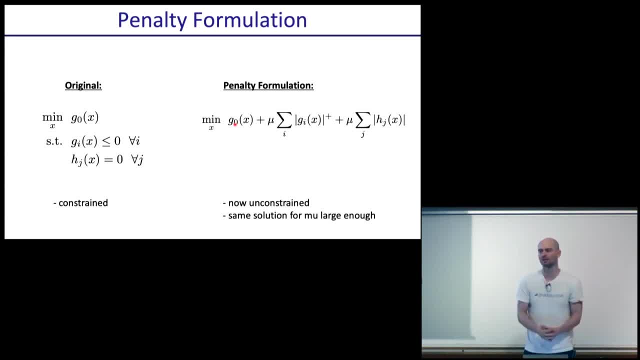 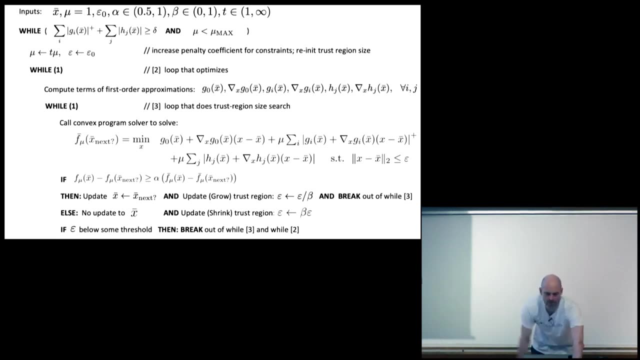 Or maybe you find that there is no local optimum from where you started, where the constraints are satisfied, Okay. So then from there we kind of broke it down into a detailed algorithm that's actually implementable directly by you know writing code. 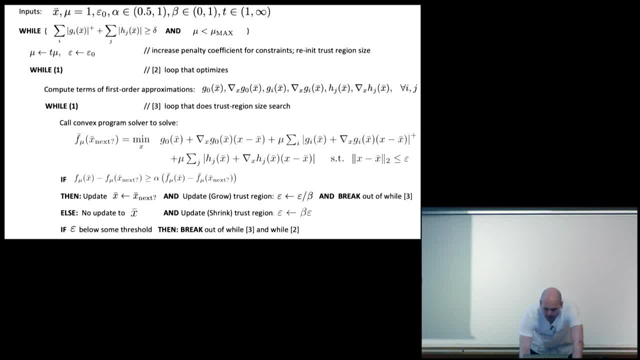 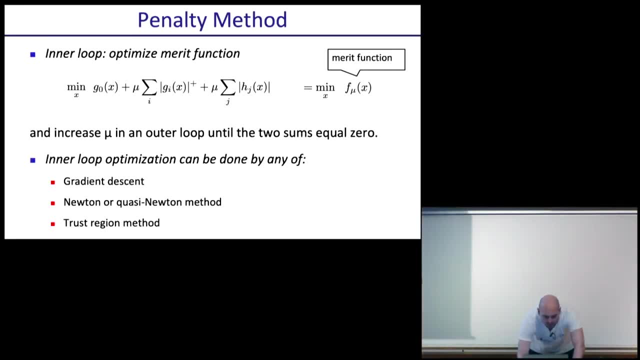 matching with what's on the slides here. The other thing we saw is that often a tweak used actually. let me go back for a moment. So once we saw this, we said there is a few ways of solving this. One is gradient descent on this objective. 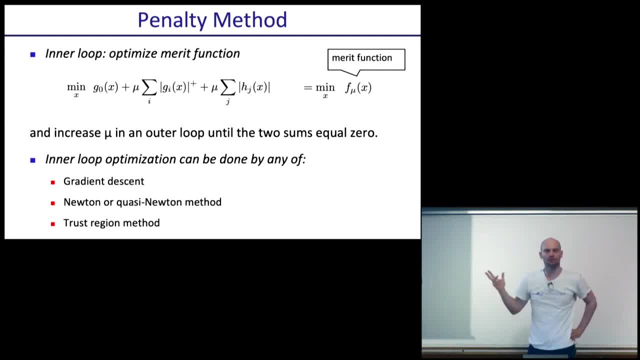 And then, when you're done, increase mu and repeat. Another one is a quasi-neutral. This is a Newton method. When you have optimized for x for a fixed mu, you're done with optimizing for x. you increase mu and repeat, Or you could do a trust region method. 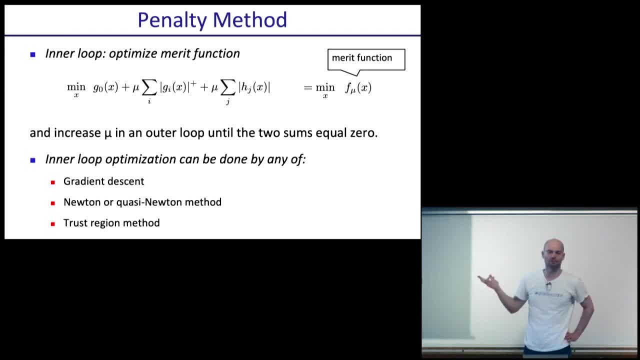 And the first two are totally fine to run. but a reason that often trust region methods are preferred is because these penalty terms have kind of a well, a very specific local structure that you can exploit in your inner loop directly rather than just looking at the first order approximation. 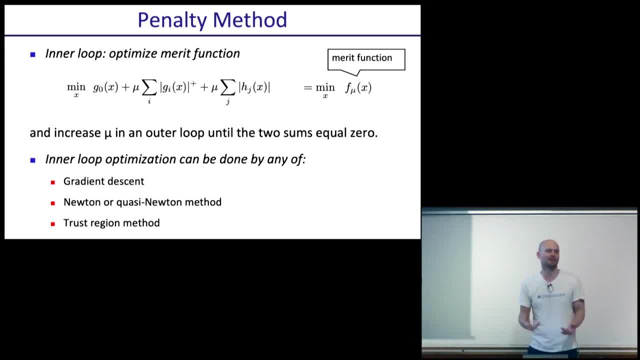 Because the first order approximation of these penalty terms is not a great approximation per se, because those two terms are not locally linear, where you want often to be, They're linear and another linear that together form absolute value, or linear and horizontal forming the value. 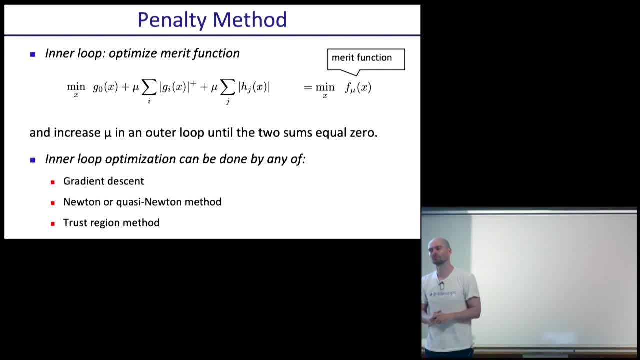 Yes, there's a question there. Yeah, so could you maybe give us a sense of if you were faced with some optimization problem that was forming what order you would try these methods? So typically, I would imagine that if your problem is relatively low, 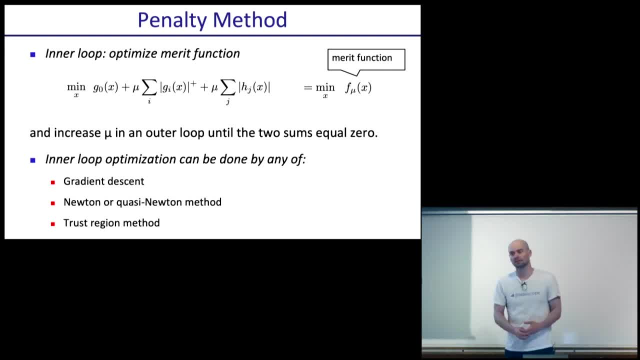 you would try a trust region method, because essentially you'll have solvers- which we'll look at later in this lecture- that will solve the inner part- the trust region approximation of problems- super quickly and very precisely, and then you'll iterate over mu. 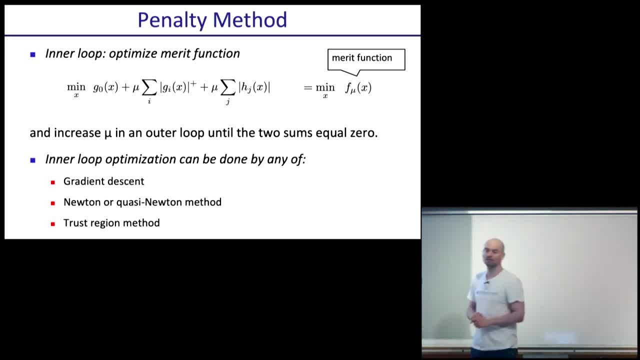 and ultimately you'll find a good solution. But these solvers often well, these dedicated solvers, often don't scale too well once you have really large problems. And so if you have a really large problem, I don't know, maybe a millionth error. 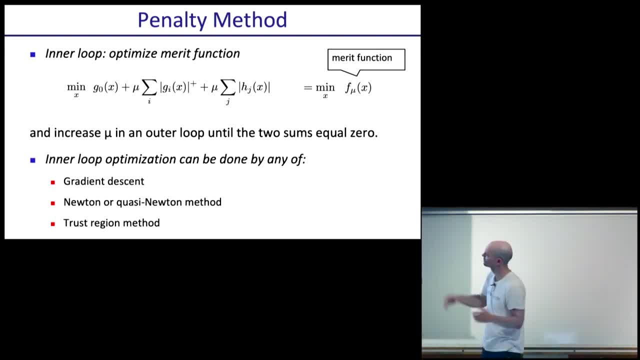 or something. it also depends on the sparsity and so forth and the constraints. but once you have larger problems at some point the trust region inner loop might become a little too expensive and you might resort to just doing gradient descent and hope that you find a reasonable solution that way. 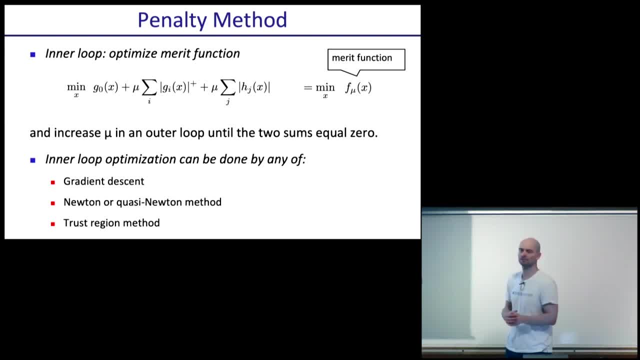 And then gradient descent typically will be pretty poorly conditioned because well different variables will contribute differently to the objective. so in practice it probably wouldn't be gradient descent but a quasi-Newton method. Think of gradient descent as something you probably would never realize. 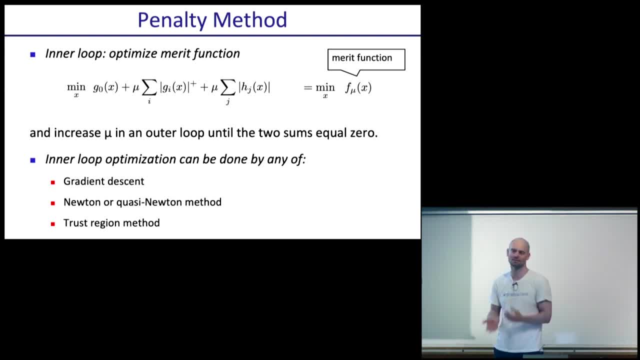 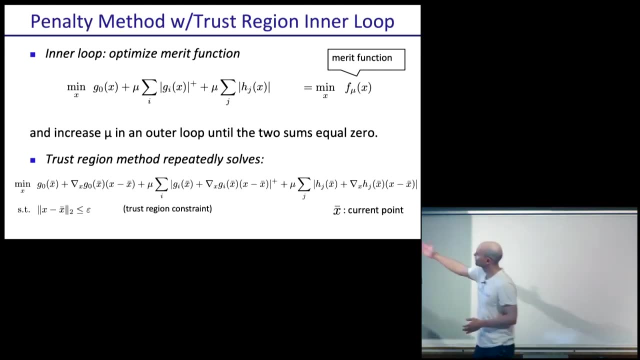 you'd never really run. You'd probably prefer a quasi-Newton because it's about the same cost to run but will scale things better. Now what happens inside the trust region is this problem is being solved, shown here. This problem approximates the objective. 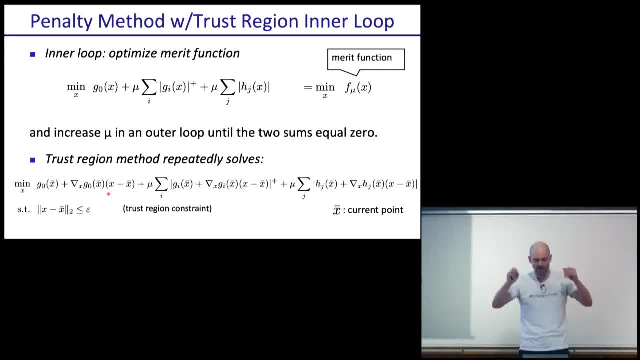 well, linear approximation approximates what's inside those penalty terms with their local linear approximation. By doing that, we actually have something called a convex problem, and convex problems, as we'll see, can be solved very efficiently. and so often this thing, this trust, region, local problem- 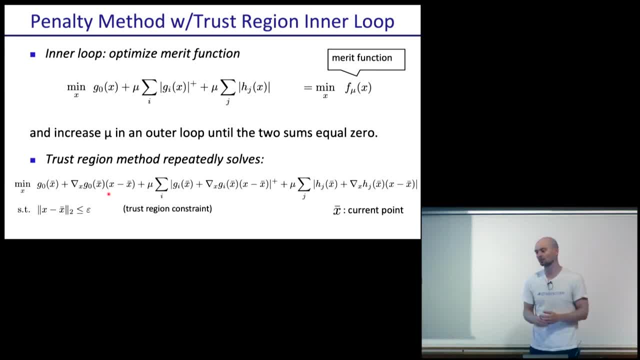 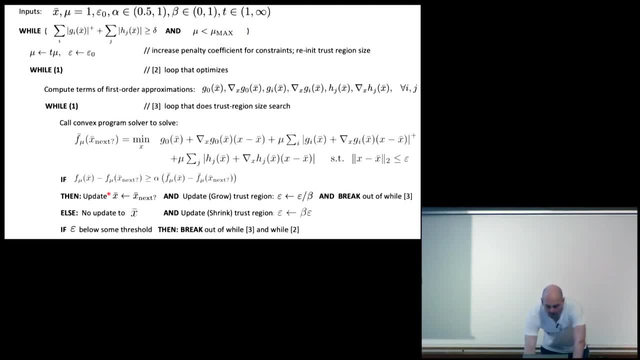 is solved with a convex optimization solver, unless the dimensions don't allow you to do it. We saw a little more detail about how to do this and then we said: actually, since we're gonna solve the inner loop with a convex optimization solver, 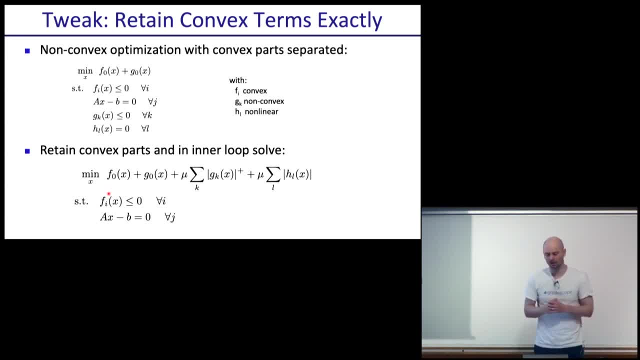 why don't we pay a little more attention to the inner loop, a little more care to looking at what actually is now our original problem? because imagine you had a constraint of the type. constraints lie between negative one, controls lie between negative one and plus one. 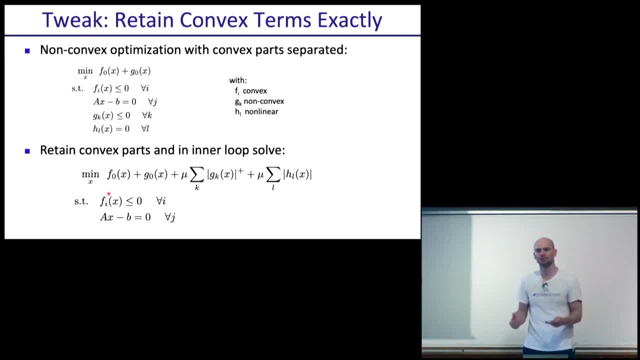 Well, we can just retain that exactly. We don't need to replace that with anything else, and so anything that's a convex constraint. we're just gonna keep and feed it directly as is, without approximation into the inner loop, solver, and so they won't become penalty terms. 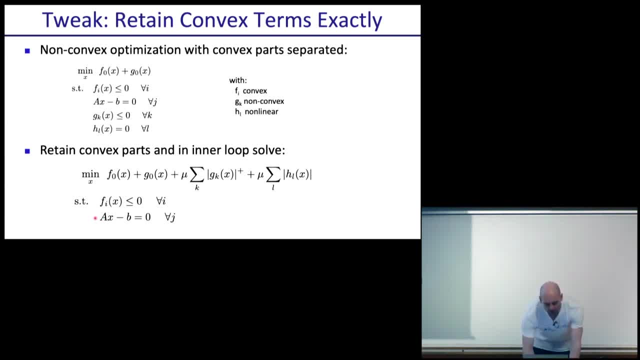 They're just retained as constraints here and then retained in that inner loop solver. So at this point we've seen all the outer parts. We've not seen what happens on the inside When we actually try to solve that problem shown there. 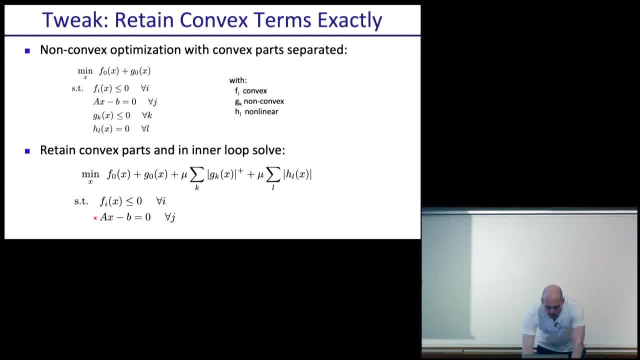 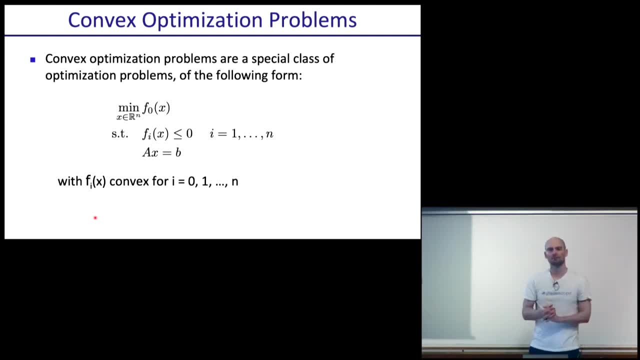 how do we solve it very efficiently, Okay, so let's now take a look at that. So convex optimization problems are problems where we have an objective and possibly some inequality constraints, some equality constraints that are convex, meaning every function fi here has to be convex. 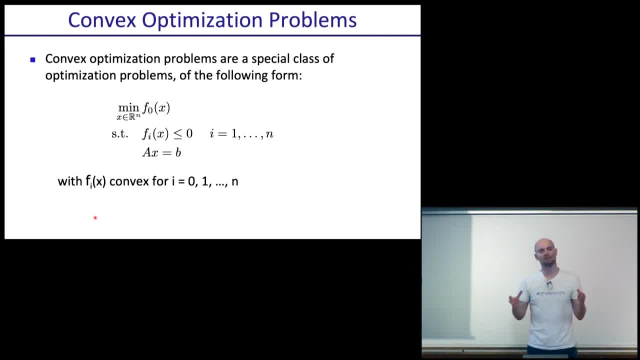 meaning every function fi here has to be convex. meaning every function fi here has to be convex. If a function fi is convex then it means it's bowl-shaped And the region where it's smaller than zero is a convex set where any two points in the set 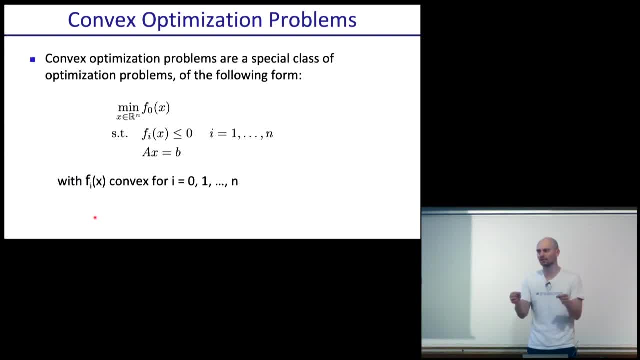 you take the line between those two points, that entire line lies within the set, And so it's a nicely shaped region of which it's easier to optimize than if there's disjoint sets or non-convex boundaries. Ax equal b is a linear constraint. 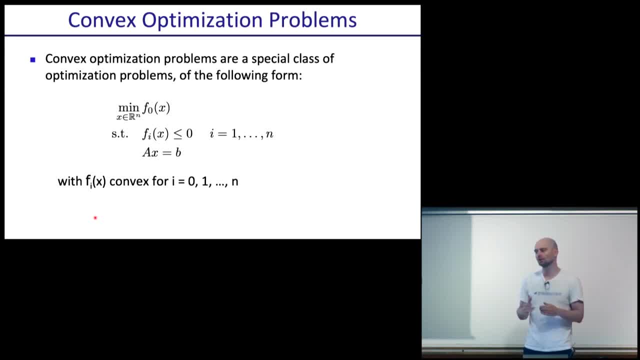 is our only type of equality constraint, Because once you have nonlinear equality constraints, the region of feasible points becomes non-convex, Because once you have a curve and you need to be on that curve, then two points on that curve, you connect them with a line. 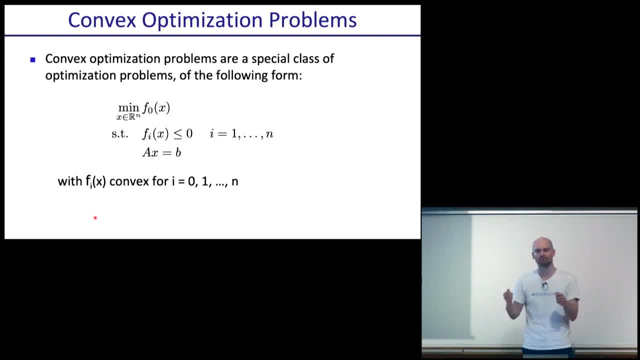 you're not on the curve anymore And so it's not convex anymore. Okay, so this is now our assumption. So it's a strong set of assumptions. but we've also seen how a problem that doesn't satisfy these assumptions can, in the inner loop, be molded into this. 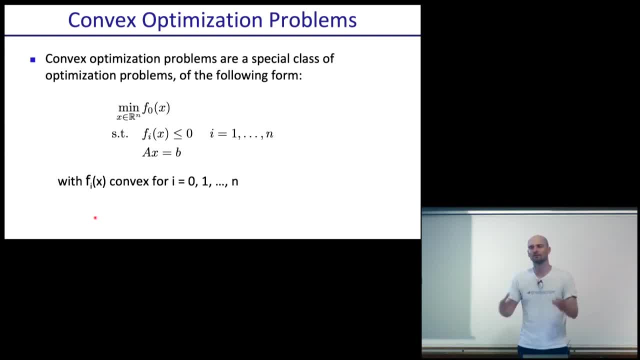 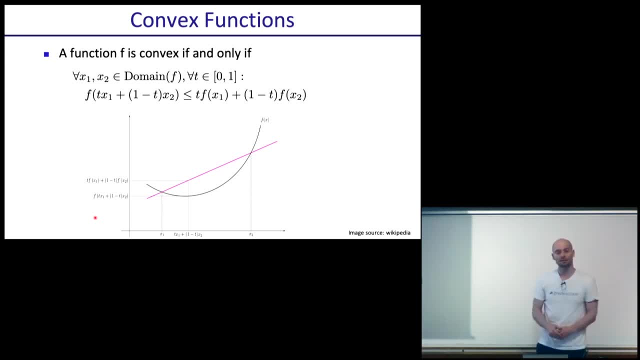 And in the inner loop we can apply this, even if the outer problem we're solving might be non-convex. It's a quick reminder. So it would look something like this: a convex function in 1D, but the way you test for it in higher dimensions is the same. 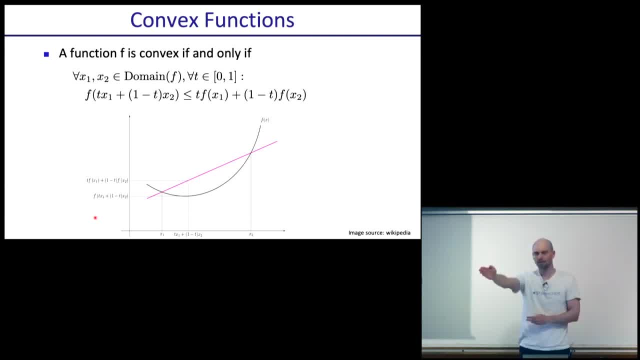 You take a slice in one direction and you look along that slice. What does the function look like? Does it look such that the line between two points lies above the function? Then it's convex. If not, it's not convex, It's a 2D function. 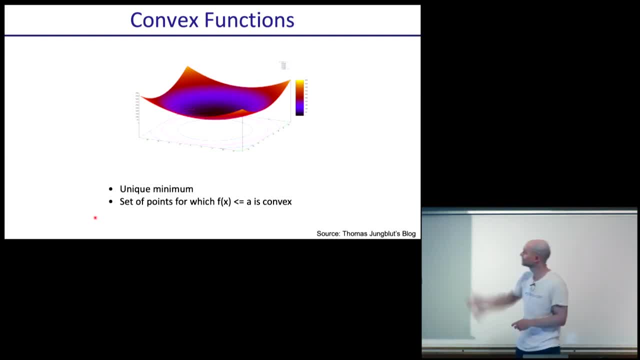 You can draw contours, but in general that's not gonna be possible. But if it is 2D you can look at it and the contours will be convex. Now we have to deal with two things. We have to deal with equality constraints. 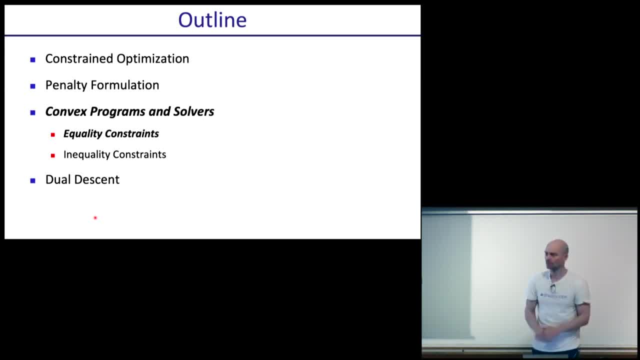 and inequality constraints. So let's first deal with equality constraints and ignore the inequality constraints, and then we'll look at the inequality constraints separately. So then the problem is of this form: Minimize over x f of x, such that ax equals b. And we'll see three different solutions. Minimize over x, f of x, such that ax equals b, And we'll see three different solutions. Minimize over x, f of x, such that ax equals b, And we'll see three different solutions. 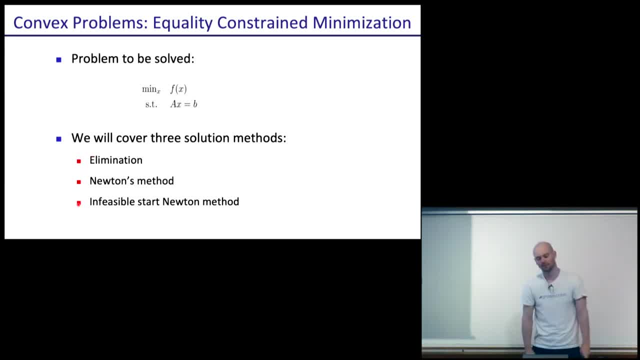 Elimination Newton's method and infeasible start Newton method. There might be different benefits to them depending on what type of problem you're solving, So we'll cover all three. Don't think of one as better than the other, It's just different situations might have. 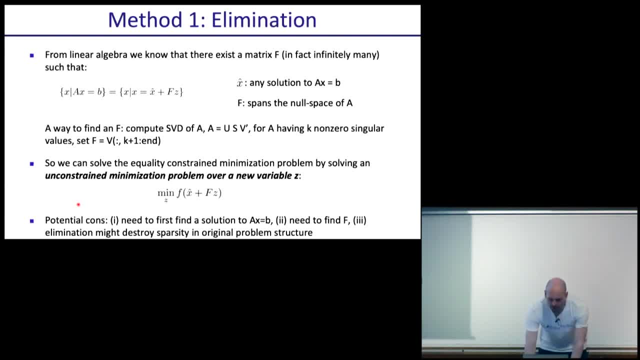 different methods be the right fit. Okay, so method one is elimination. When you have a set of equations x, such that ax equals b, kind of the canonical thing that you might have seen as well: number of equations equal to number of variables. 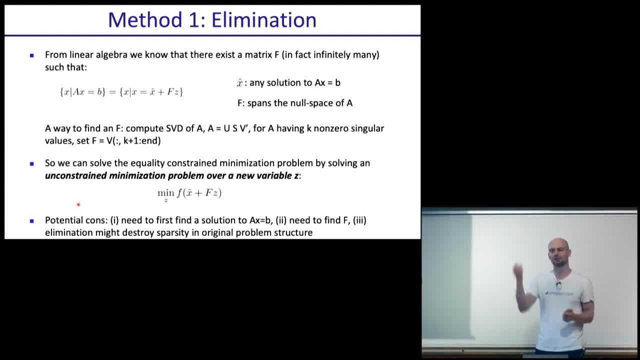 and there is a single solution, and then actually the optimization problem is not that interesting. It's just that one single solution is the optimum of your optimization problem. you're done Usually in optimization problems and then the other thing you might have seen is least squares. 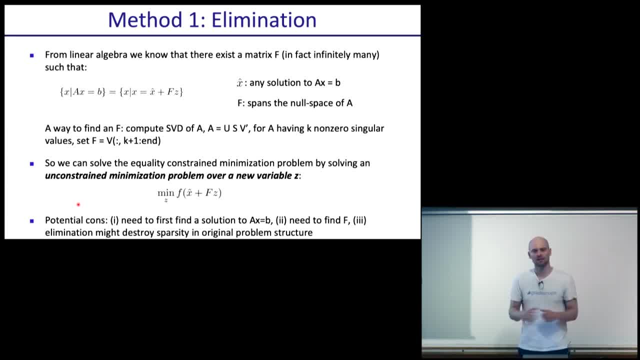 So we have a bunch of equations and there's no x that satisfies all of them. You try to find the x that's as close as possible to satisfying all of them. Here we're in the opposite regime. We're in a regime where there's less equations than unknowns. 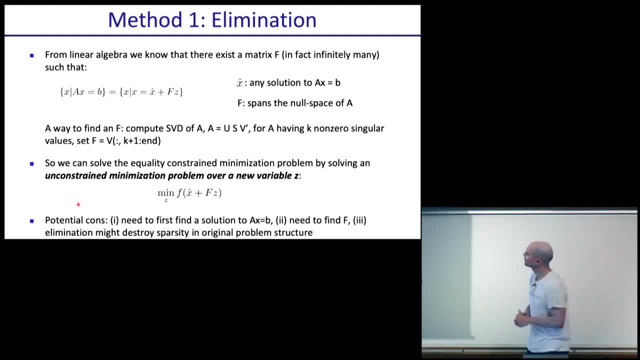 So there'll be a set of solutions. So ax equals b- less equations than unknowns. There'll be a set of solutions. When that's the case, linear algebra tells us there'll be a set x, such that x equals x hat. 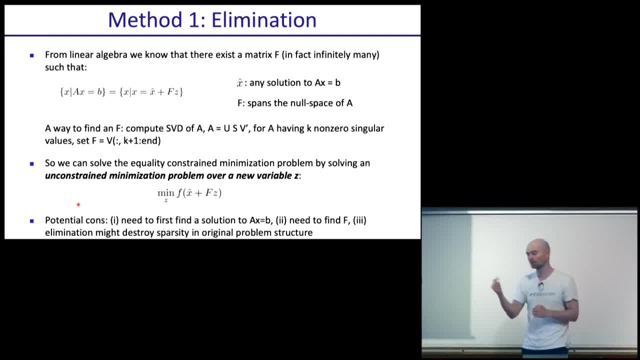 which is one solution. You just find one solution to the set of equations plus f times z, where f is a matrix and z can be any vector, then, of the right dimensions. And so how do you get this? Well, f needs to span the null space. 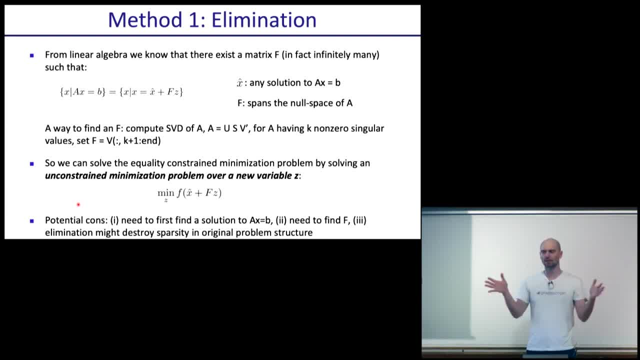 So f is a matrix of a meaning. f is something where, if you take a linear combination of the columns of a, any such linear combination of the- I'm sorry- any linear combination of the columns of f, you multiply that with a, you get zero. 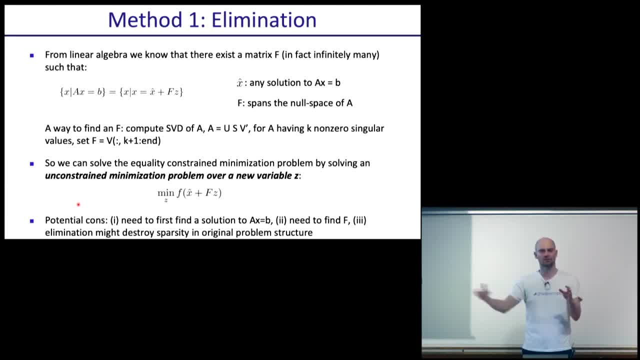 So we'll have a times f, times z, always equal to zero. How do we find this f? One simple thing you could do is compute the singular value decomposition of a. So singular value decomposition will say a equals. and let me draw a quick picture here. 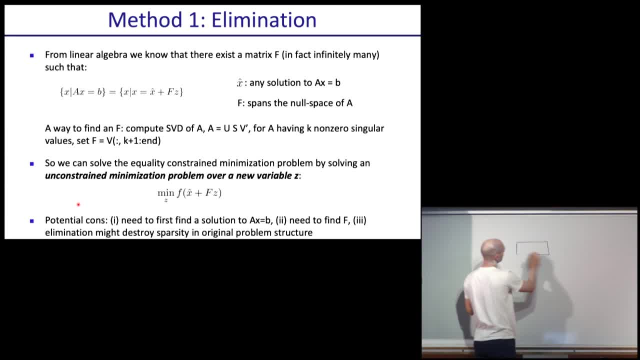 a is in this case a fat matrix, right, Whereas in least squares, which you're probably more used to seeing, it would be a skinny matrix. but here we have a fat matrix: less equations than unknowns. This is a and this will be equal to u sigma. 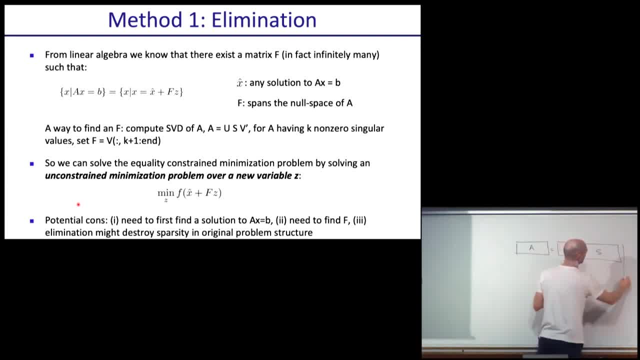 or we'll call it s there, times v transpose, and this one will only have entries on this diagonal here. It's not a square matrix, it's kind of a funny diagonal, but it'll only have non-zero entries here, which are the singular values. 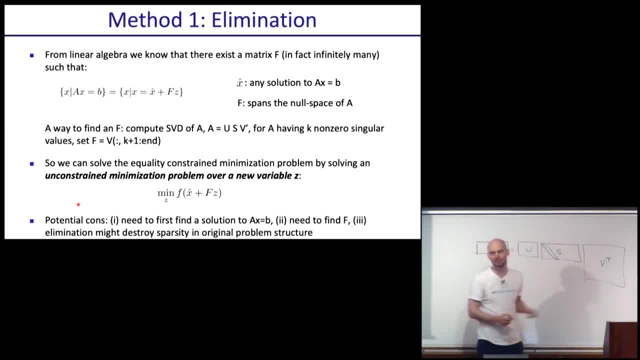 This will be an orthogonal matrix. this will be an orthogonal matrix meaning u, u transpose equal identity and same v, v transpose equal identity, same for v transpose v and u transpose u. So that's singular value decomposition which, if you actually don't remember, 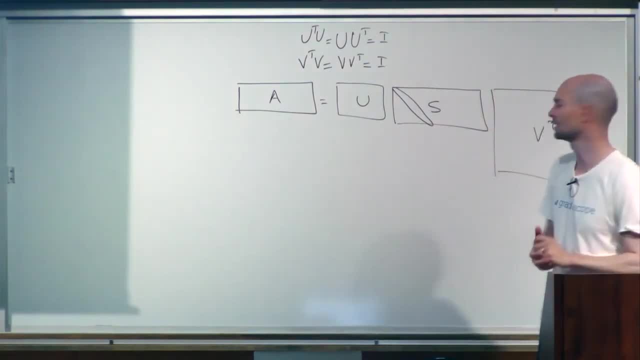 I highly recommend you restudy it because it's probably the most important concept in linear algebra And what we're saying is that, essentially, when we multiply, we want to find solution to ax equal b. We already found a solution: x hat. 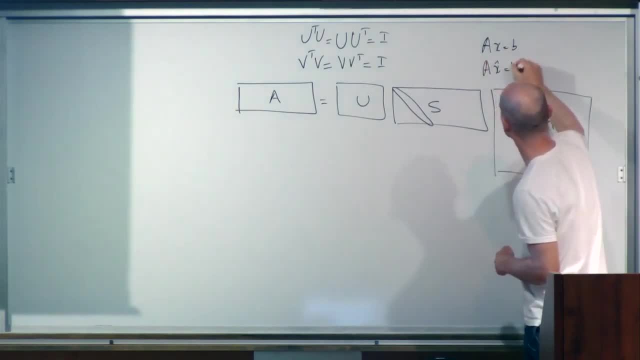 We know ax- hat equals b. What we're claiming is that we can find other solutions of the type ax- hat plus delta x equal b, And that these solutions can be found by essentially looking at this matrix v here and realizing that if you have a vector x, 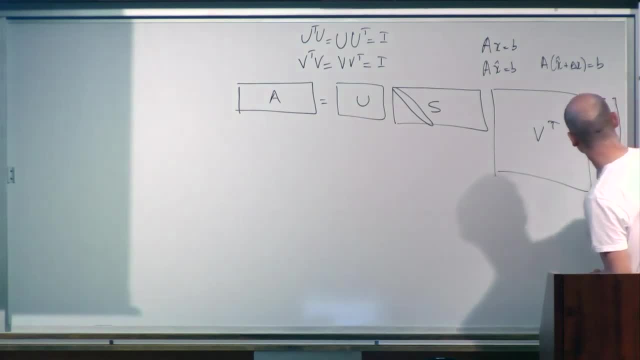 or x plus delta x. say x hat plus delta x. you're multiplying with v. transpose then the only thing that gets passed through, because these are the only here we have non-zero, but below it it's all zeros. so only thing that will get passed through. 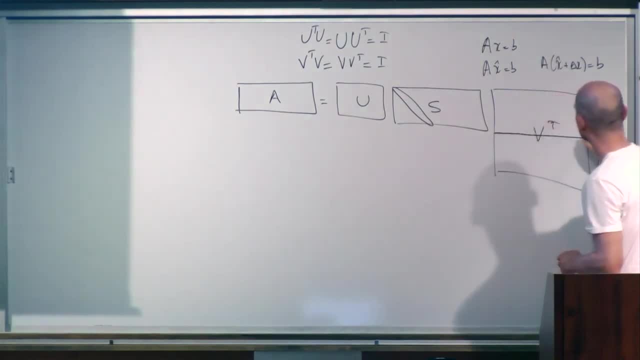 is what goes into the first set of rows of v. transpose: If your vector x has a non-zero inner product, with these rows, that will get passed through. That will have an effect on the outcome. We need to be careful we can't do that. 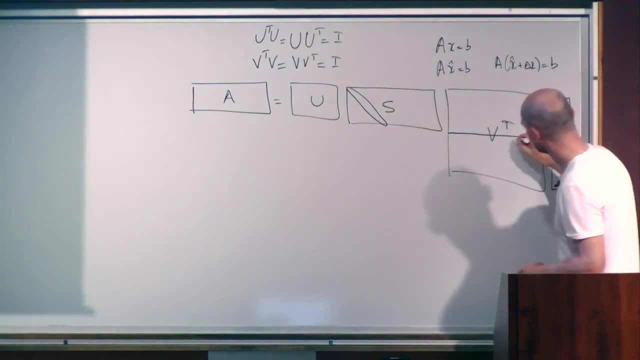 because that will make it not b anymore. But anything that has zero inner product with the top and non-zero with the bottom here will be passing through like nothing changed and you'll still get b on the other side. And what is this? 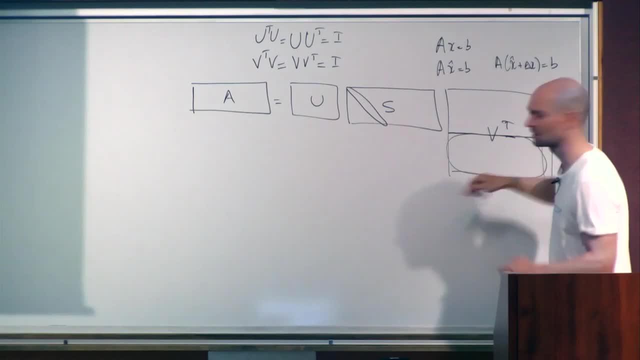 Well, this is v transpose. So really what? this is the last rows of v. transpose the last columns of v. This is the last set of columns of v that span. that are the basis for the things that we can add to the one solution. we already have x hat. 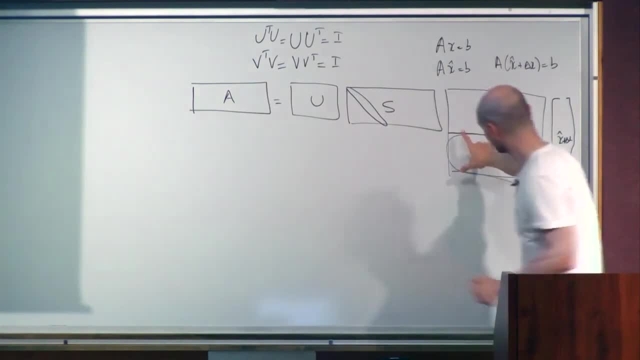 And so that's what we can do. We do single-valued decomposition. We grab these rows which we'll think of as columns, and we'll take these rows which we'll think of as columns, and we'll take these rows which we'll think of as columns. 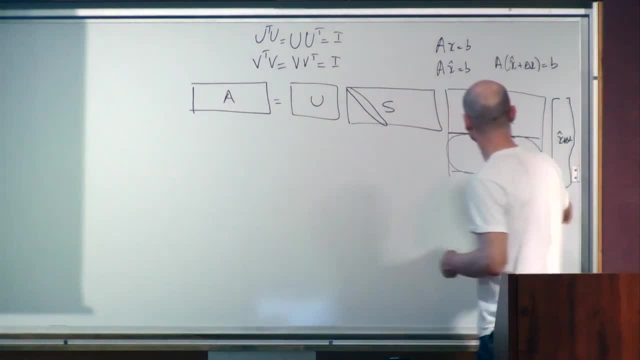 and we'll take these rows which we'll think of as columns now, and that is our f matrix. So this here is f: transpose lives down here. That's it. that's all we need. Okay, what are some benefits? 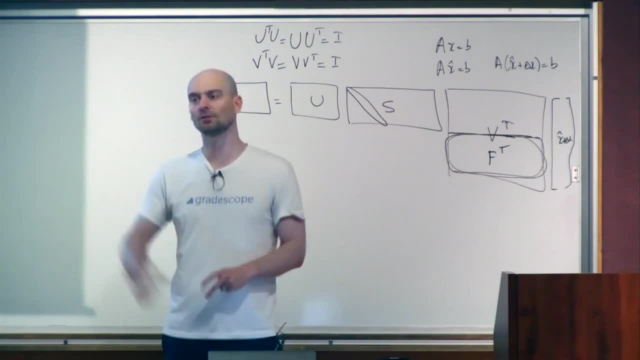 Well, one benefit is actually you reduce the dimensionality of the problem you're solving. You used to solve over your optimization, over x space, and z will be smaller, lower dimensional than x. so you now solve a lower dimensional problem And sometimes that's pretty convenient. 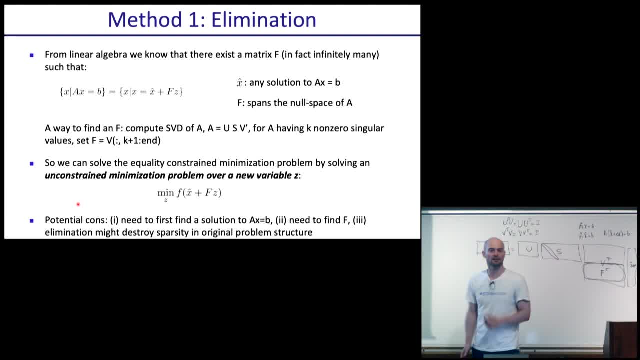 So that's one thing to do. Then often the number of constraints is not that high. then it will not reduce the dimensionality much. You might not care much for that Potential downsides. you first need to solve ax equal b. 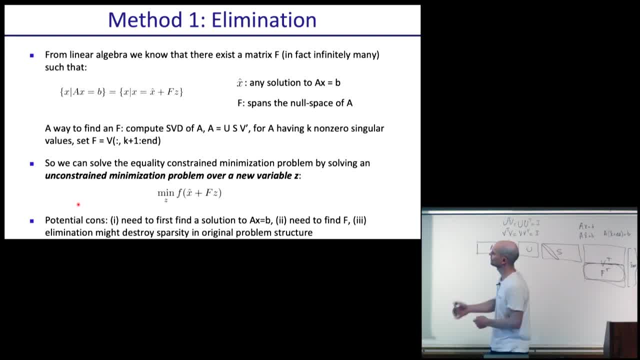 and find the null space of a, for example through single-valued decomposition or other methods, Then that'll give you f. And another big downside is probably the biggest one: that why people usually don't use this method is bullet point three. This elimination might destroy the sparsity of a. 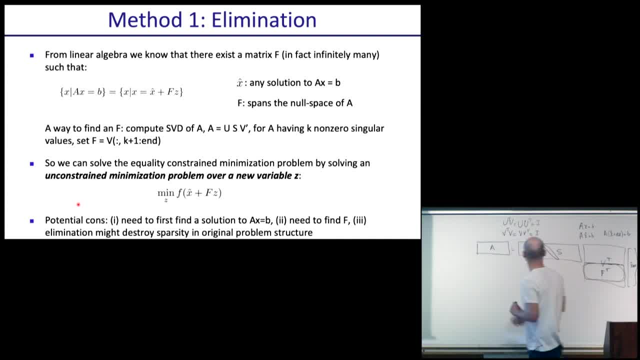 So very often when you set up an optimization optimization problem, you might have a high dimensional variable x that you're optimizing over, but the way it participates in constraints and in the objective is very sparse. So the matrix A would have mostly zero entries. 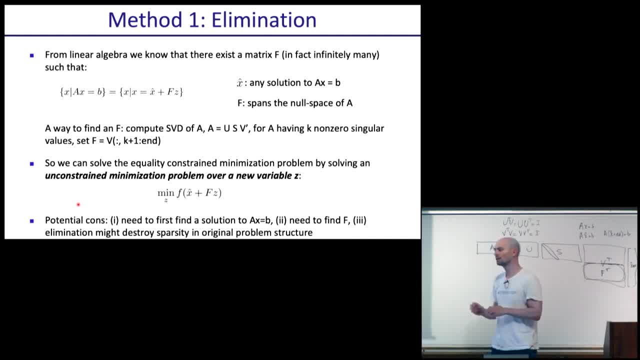 And even if your matrix A has mostly zero entries, your matrix F will typically be dense, And so, all of a sudden, you're dealing with a computation much more expensive problem, even though reduced, you reduce the dimensionality. And so if, of course, if A is not sparse, 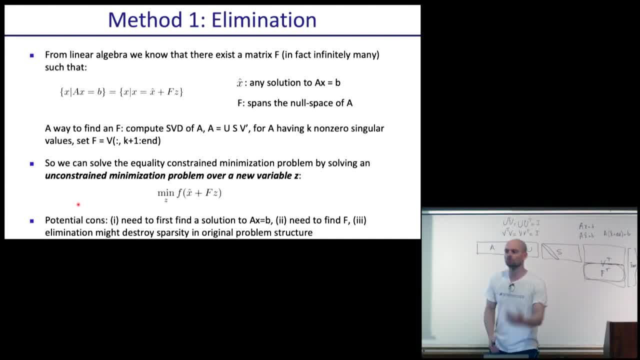 when you start out with there's no reason to worry about this, but most practical problems, A will be sparse and so three will be the issue, and you will not wanna do it this way. Any questions about this? So mathematically we have a way of solving the problem. 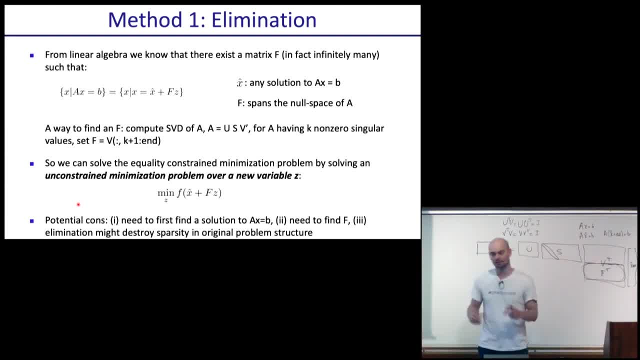 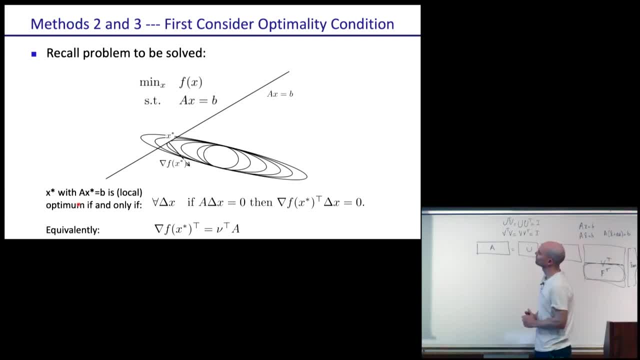 It's just that we know that in practice often we're not gonna wanna do it this way, because often A will be sparse. What else can we do? Let's think geometrically about the problem. We're minimizing some function f of x, in this case over two-dimensional space. 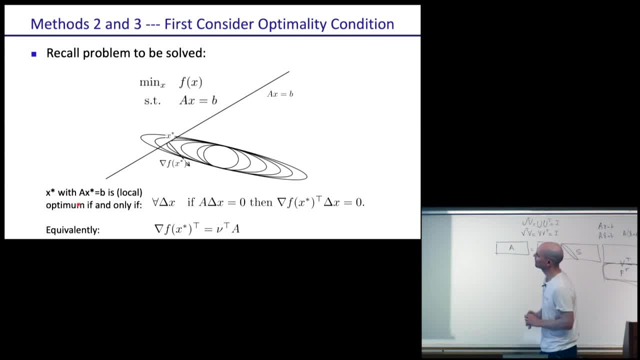 so we can draw a picture. We see the contours there of f, of x, And if there was no constraint we'd wanna land right in the middle over here. But there is a constraint: Ax has to be equal to b, So it can only be on this line over here. 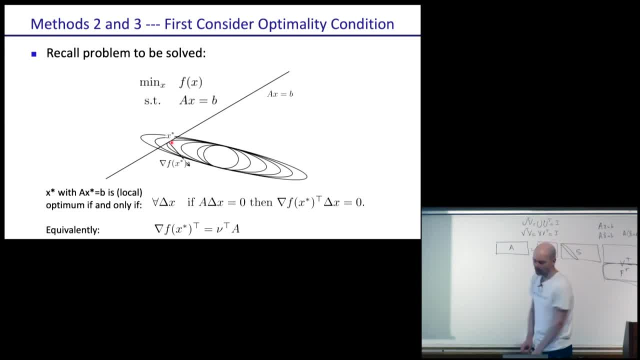 Well, can we geometrically think about what it means to be an optimum? We have to be on the line, And which point on the line is gonna be correct? Well, the point on the line is gonna be x And the point on the line is gonna be y. 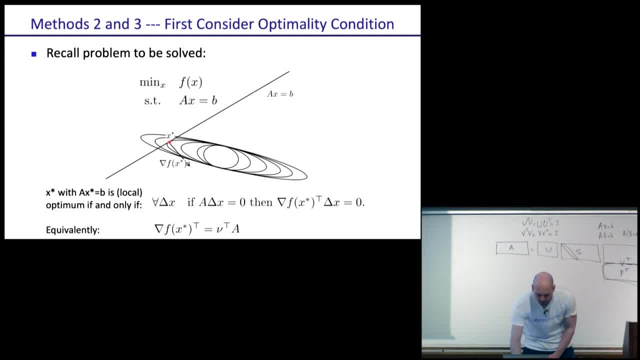 Now, the reason this point is correct is from here, the gradient points orthogonal to that line. So when we move to the left or the right, we don't get any improvement, because the inner product with the gradient will be zero, Whereas for all other points, when we're further out, 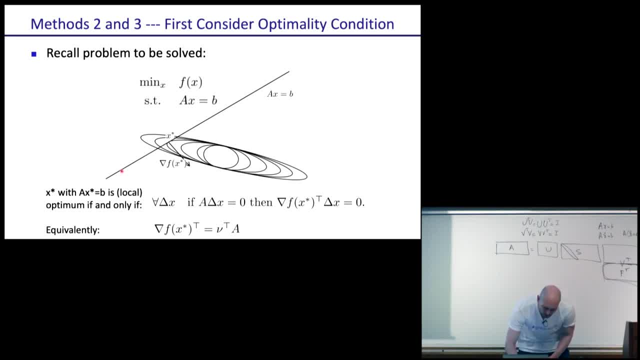 the gradient will be telling us to move in. And here the gradient again will tell us to move in along the line, And it stops where the gradient is orthogonal to that line, And so the optimality condition then becomes: we are at. 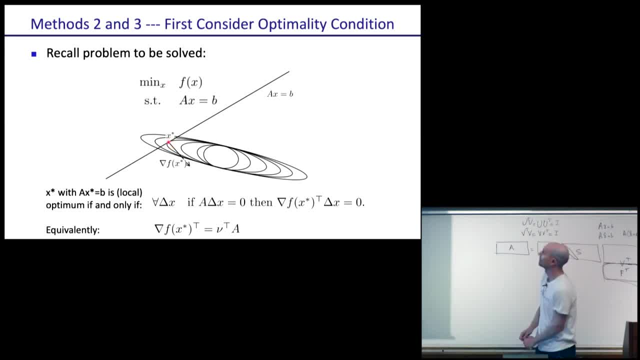 a constraint optimization problem. optimum in this case whenever the gradient is orthogonal to the line- In this case, in general, the plane or hyperplane, on which you need to live. What does that mean? Well, we'll do the bottom one here first. 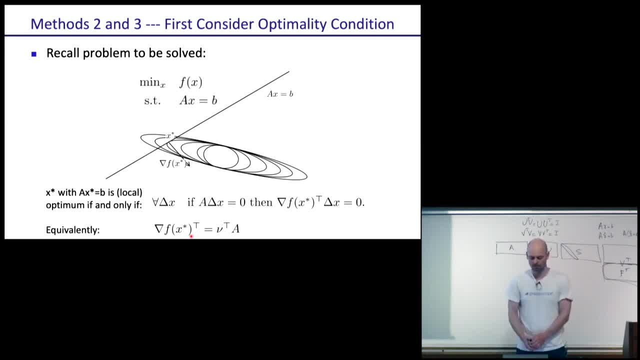 For the gradient to be orthogonal to that plane. what does it mean to be orthogonal to the plane? Well, the way you define that plane is by a set of vectors living in A. And you say A times X has to be equal to zero. 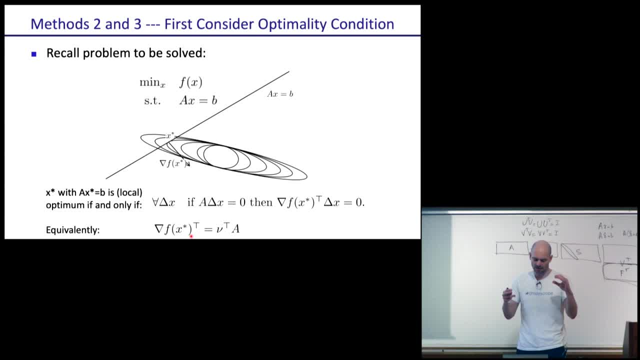 meaning that X or equal to B. So what it means is: A- the vectors in A span what is orthogonal to the plane. And we want the gradient to be orthogonal to the plane. So that means the gradient should be aligned with whatever are the vectors that live inside A. 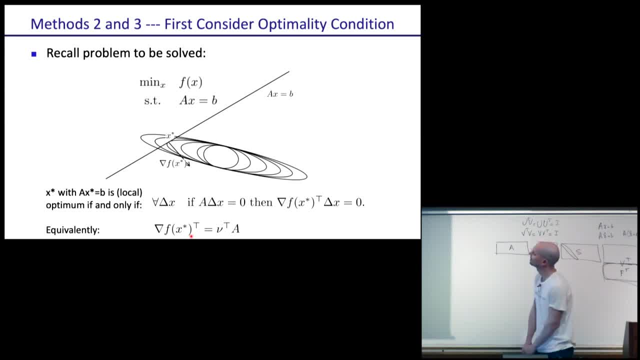 because they define orthogonality to each of the planes that you need to be in. So that's this condition here. You can also write it this way: for all delta X that we can apply to X if. for all delta X that we can apply to X if. 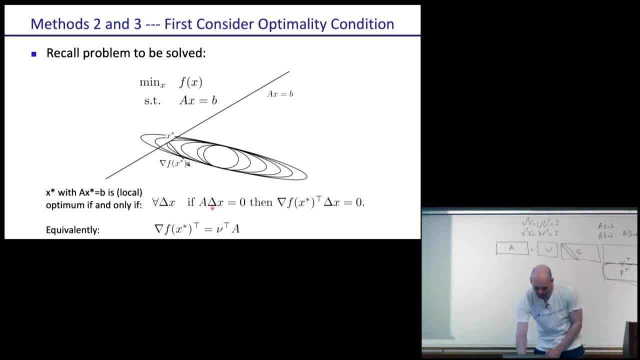 for all delta X that we can apply to X. if A times delta X equals zero means we remain feasible. because we start with a feasible, we're trying to check if we're optimum. If a change remains feasible, then for that change. 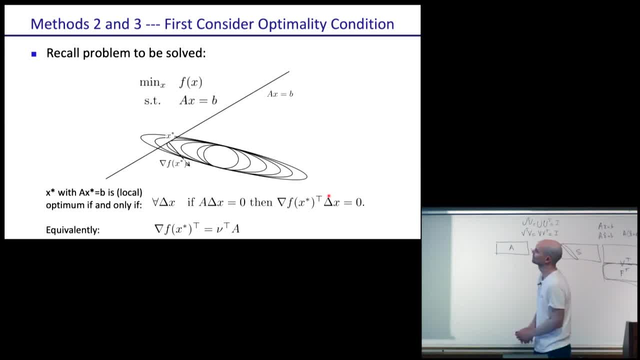 we have to be orthogonal to the gradient. So these are two equivalent conditions. Now one way to solve the problem is to just look at those conditions. Say, can I find a X and a mu such that the gradient equals this thing, or can I find a X such that A delta 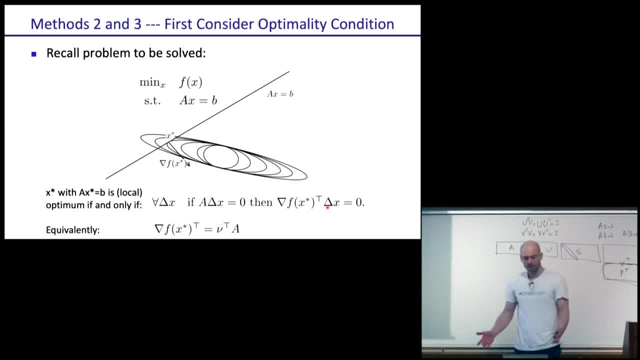 whenever A delta X equals zero. this is true. Maybe sometimes we can. let's see what we can do. So optimality conditions we're gonna work with is that we want AX star equal B and the gradient to be spanned by the columns of A. 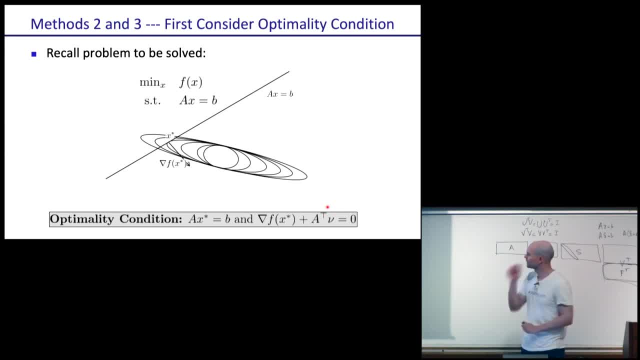 All right. so how do we do this? Sometimes you can do this analytically, So for some small problems, sometimes you can write this out and you can say, okay, this is just a solution. closed form: you're done. 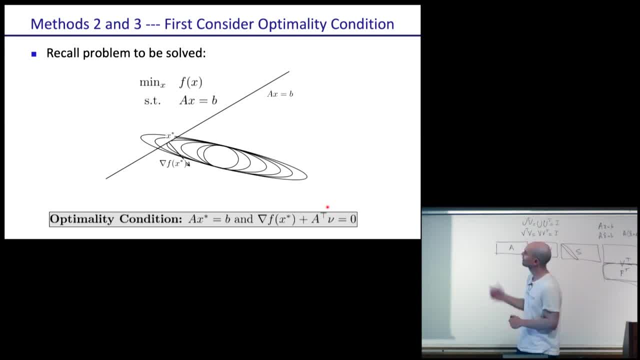 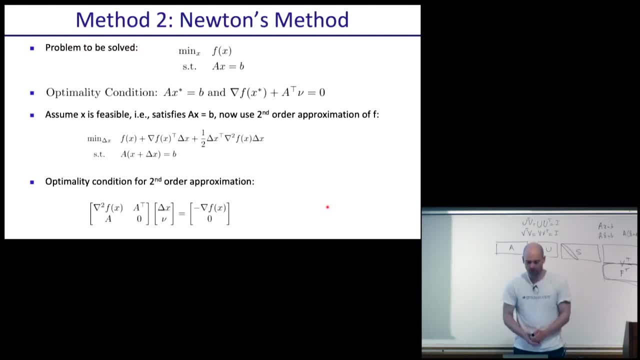 And then that's great, that's very convenient. Most of the time it's not gonna work. So we can actually extend Newton's method to this scenario. Here's what we do. We say: optimality conditions are here. Let's assume we have a feasible X. 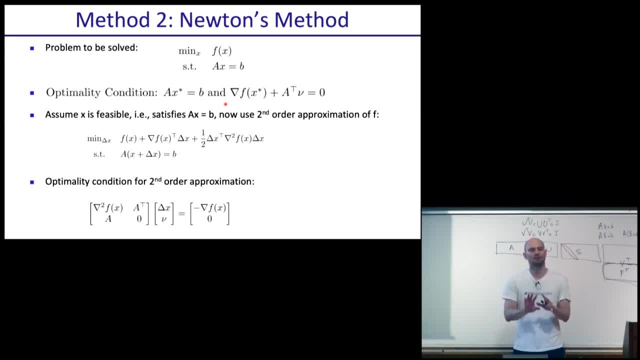 So there's an assumption. We will relax that assumption later. Let's assume we have a feasible X, So we already solved AX, equal. we have some X, not the optimal X, but AX, Then we can use a second order approximation. 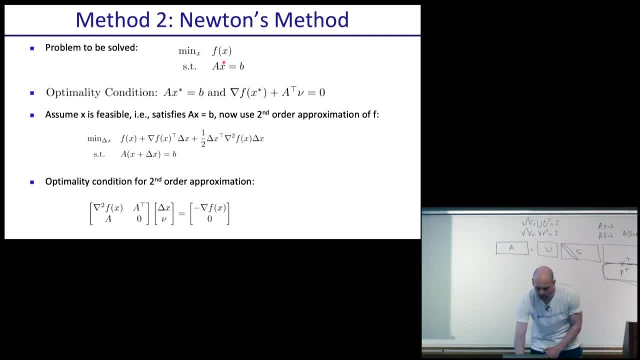 of the function F in this optimization problem here. So now we have this formulation over here. Now for the second order approximation of the problem. we can write out the optimality conditions which will give us this over here. So this is, if we assumed our problem. 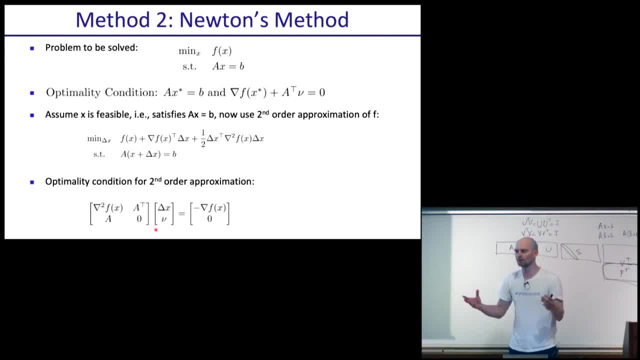 was actually a second order problem, which it is not. but if it were, then this would be the equation we need to satisfy And because it's a second order approximation, we take the grain to get those conditions. That becomes a linear system of equations. 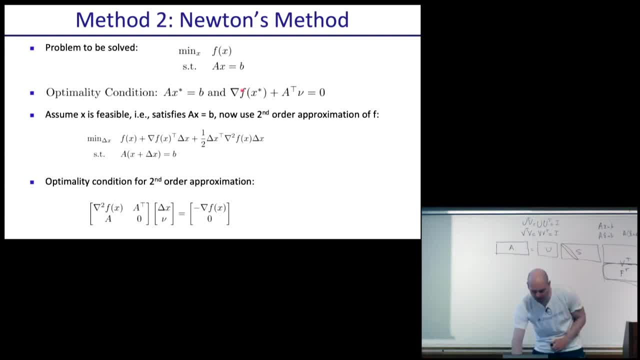 And all we need to do is solve a linear system of equations to satisfy the optimality conditions of the local approximation to the real problem, the Newton approximation to the real problem. And then, once we've done that, we can take a step. 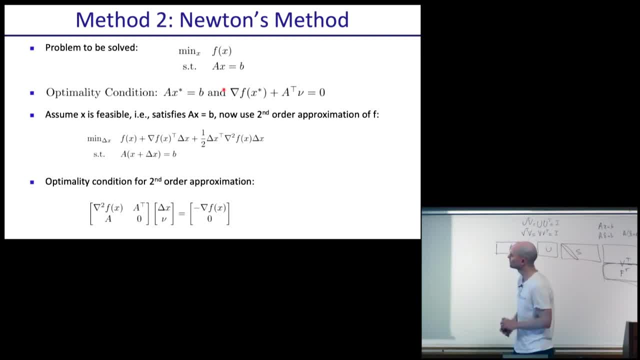 We're in a new spot. We take the new second order approximation and repeat. So computationally this is very feasible. It's very similar to Newton's method. Whenever Newton's method applies to the original problem without constraint, then you should be able. 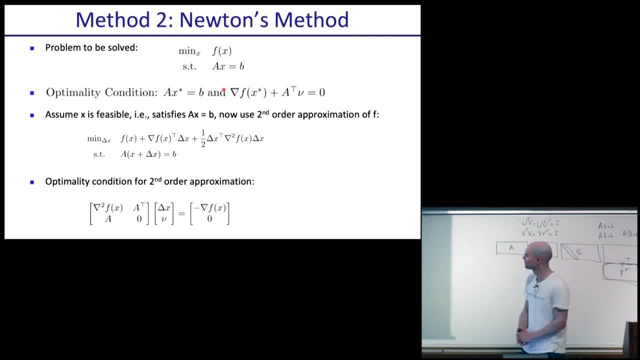 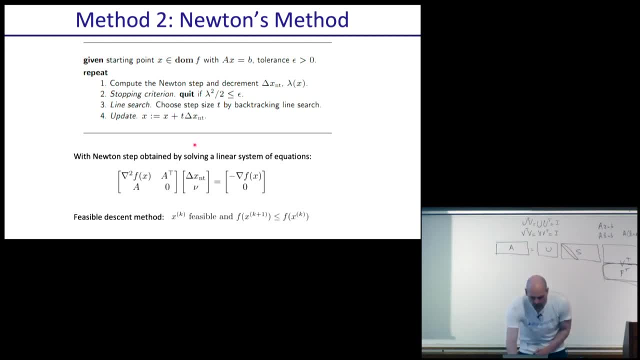 to also run this when there is the equality constraint. Maybe the only caveat: oh, let's give the full algorithm. So this would be the full algorithm. It's essentially Newton's method all over, except that the Newton step is now obtained. 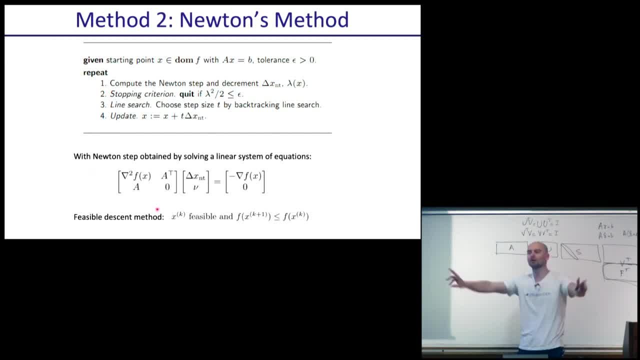 by solving this particular problem over here. What if there are no constraints? What happens Then? the A matrix is non-existent, so these parts disappear, then mu disappears and we just have the standard Newton step, Hessian times, delta x that we're trying to find. 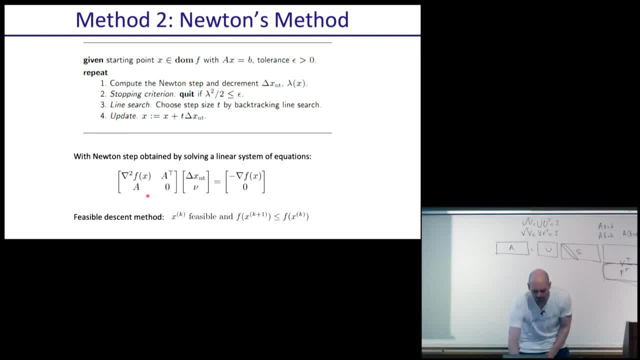 is equal to negative the gradient. So it nicely simplifies to what we already know. but if there is an equality constraint set, then we have this added to it. Now you might say I'd prefer not to first solve the system of equations to have a feasible starting point. 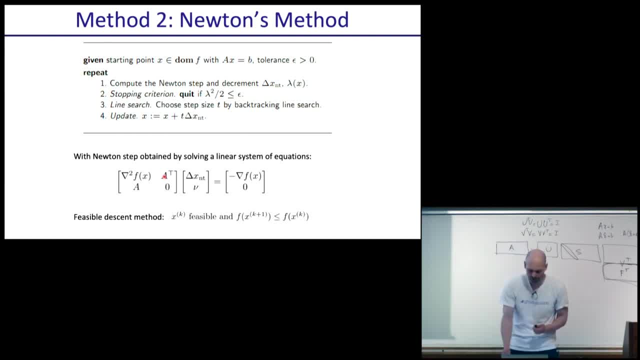 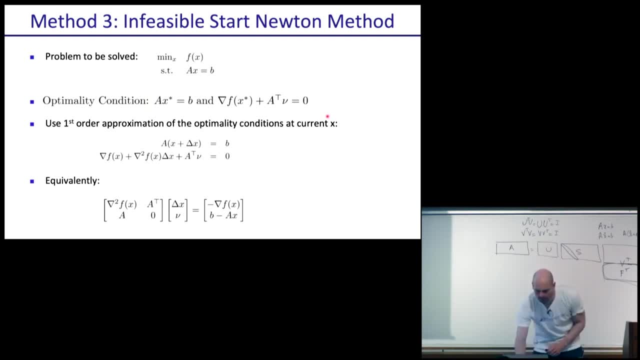 Can we do that, just having feasible start method? Actually we can. You can use the exact same idea. So remember our original optimization problem up here, our optimality condition over here. Then we're gonna do the first sort of approximation. 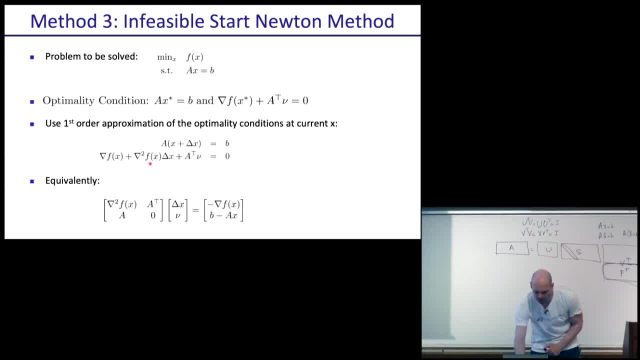 of the optimality condition at the current x shown here, And then we just solve that. So what's different between what we do here and what we did before? If x were feasible, then A times x will be equal to B. 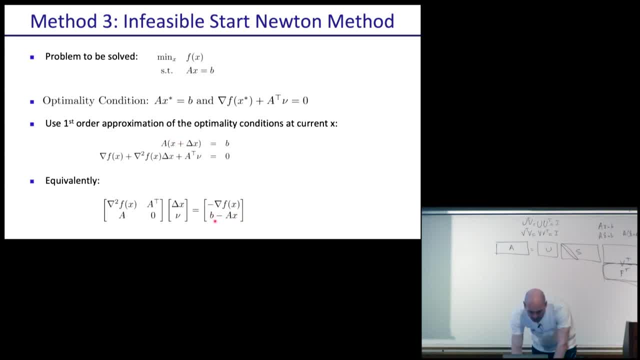 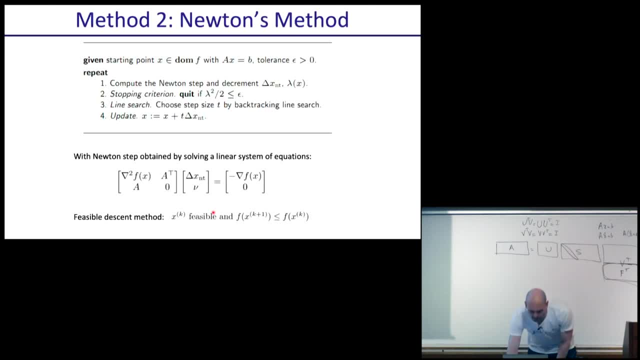 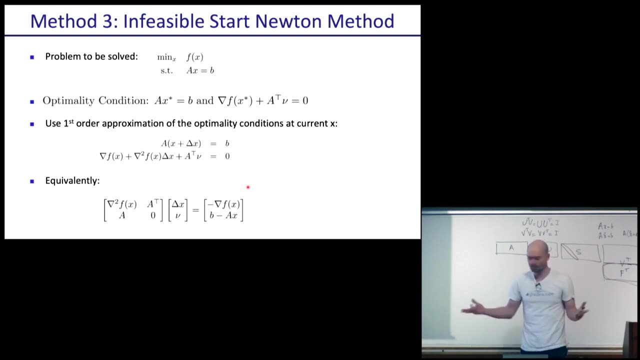 and so this thing over here, B minus A x- would be zero, and we have the original thing that we had on the previous slide where we have a zero at the bottom here. but that's the only difference. So essentially the same amount of computations to happen. 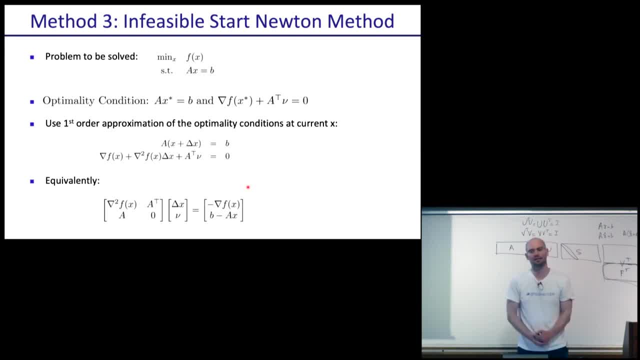 is just that you now have a B minus A x there, because we don't have a feasible x yet, and over time it'll find something feasible. Sometimes that's okay, Sometimes that's not okay. Imagine you're solving an optimal control problem. 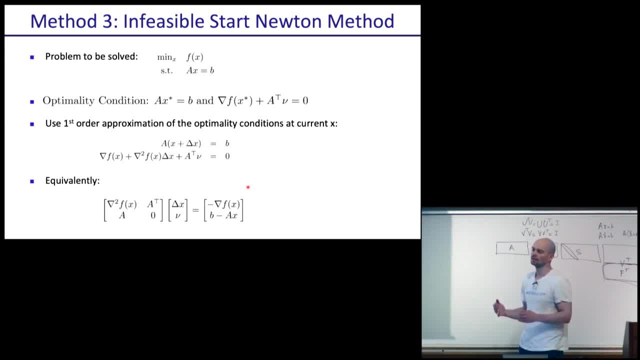 You're iteratively solving it, but you might run out of time and if your solution has to be feasible to be able to apply it, then you might not like this, because as long as you're not converged, you might not have reached a feasible point. 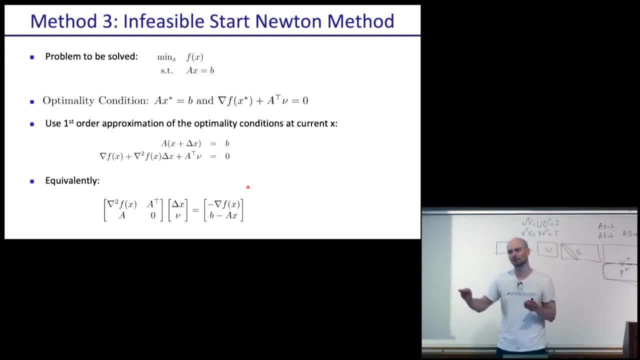 and you might prefer to first find a feasible point and stay feasible at all times, And so it depends on the situation you're in whether you really care about feasibility every step along the way now. well, you just care about feasibility once you're converged. 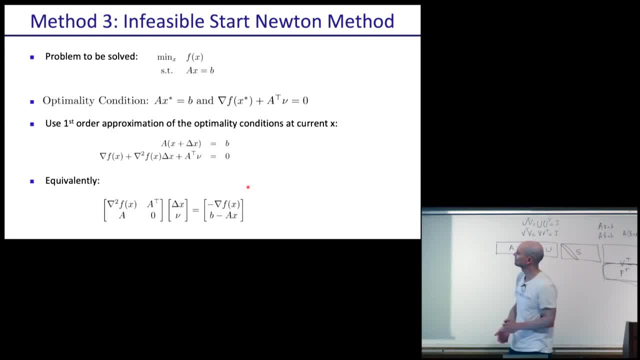 and if you're willing to wait till you're converged, then there's no reason to first solve for a feasible x. you can just wait until you're converged, and you know there's no reason to first solve for a feasible x. 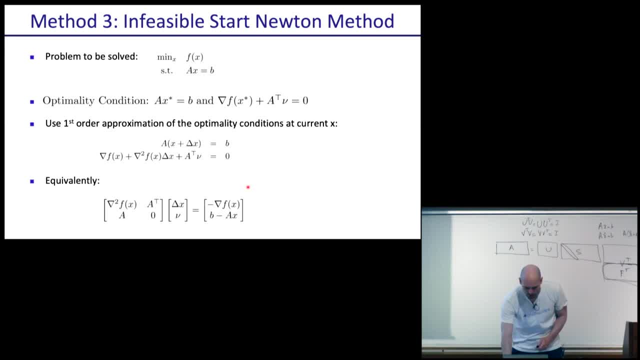 You can just run this. Okay, any questions about equality-constrained convex problems and how we solve them? Yes, Can you explain how we get the second-optimality condition? Okay, so the question is: how do we get this second-optimality condition? 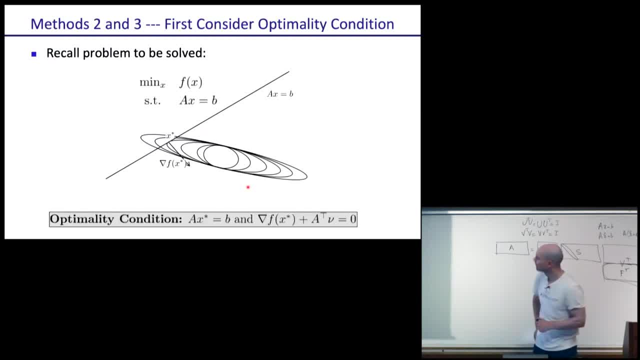 Let's go back to the drawing here. So there's two conditions. The first one is just a constraint, so that's given to us, We don't have to work to get that. The second one is saying the gradient of the function. 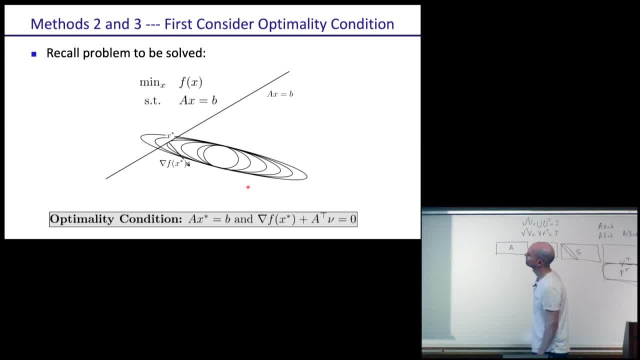 has to point in a direction that's orthogonal to how we can move in the plane. So it's saying gradient orthogonal to how we can move in the plane. so this is the plane we can move in. Gradient has to be orthogonal. 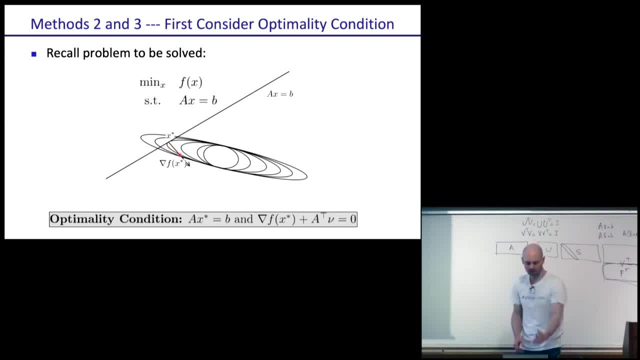 And why is that what it is Imagine? I mean, this is a 2D problem and so it's just a line. so there's just a single vector living in each one right living in A. it's just two numbers living in A. 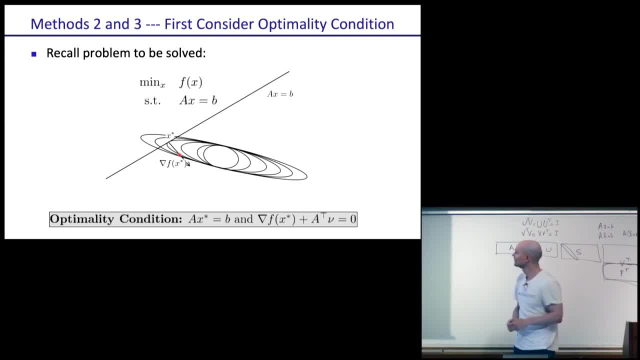 A1, A2, let's say we have A times X equals B, That vector A, that vector A for AX equals B, actually points orthogonal to this plane. That's how it works. to define a plane or a line, It's the vector that sits there, lives orthogonal. 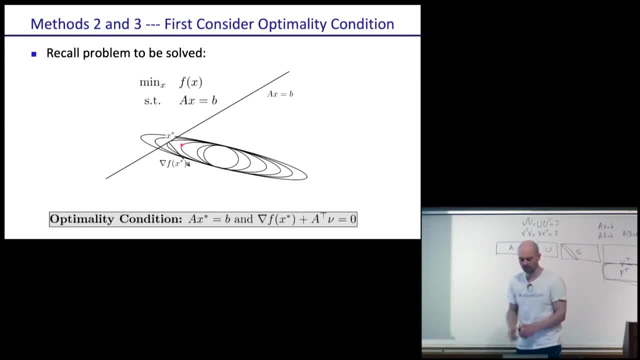 to the line itself. Essentially, what it's doing is saying that vector is saying: in the direction A you need to be a distance B out, And so you need to be a distance B out in direction A. So then at some point, your distance B out. 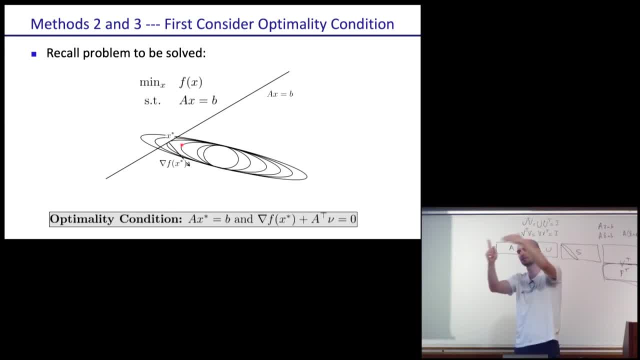 and everything orthogonal to A is on that line satisfies the condition. everything else does not, And so A points orthogonal to that line And we want our grain to be orthogonal to the line. So that's what we have there. We say our grain has to be orthogonal to the line. 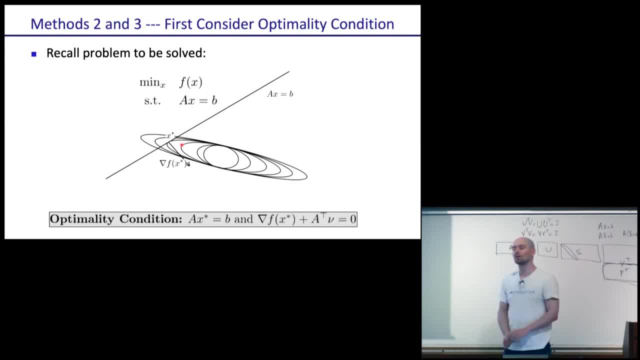 which means in the same direction as A. Now, when there's multiple constraints, multiple planes in a higher dimensional space, for each plane you can say it's okay if my gradient is aligned with the A for that specific plane, But it's actually okay to be aligned with any one of the A's. 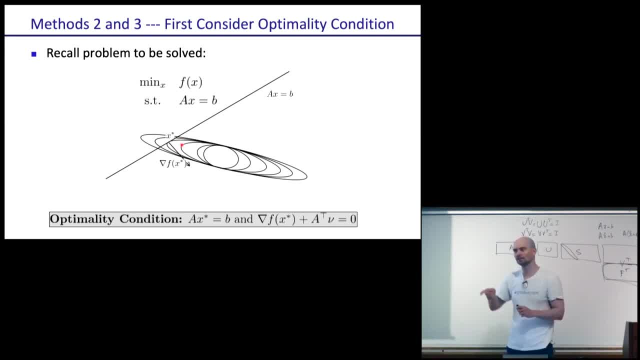 but not just any one of the A's, also any linear combination of those A's. And that's what this condition is saying, Because imagine you have two planes together they define a line. It's actually turns out, it's arbitrary which two planes you use to define that line. 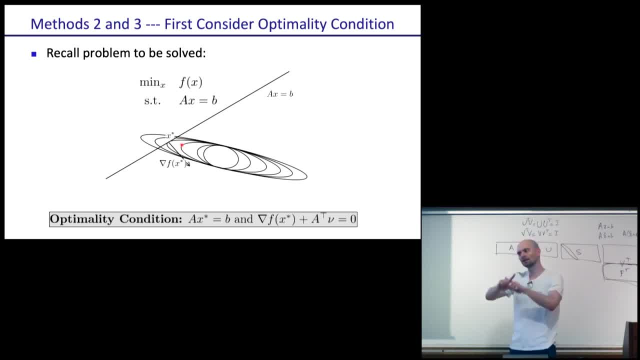 And the math works out so that you could take just the two vectors you originally had to define those two planes. You can take any linear combination and that will be everything orthogonal to that line And that will be how you want your gradient to be pointing. 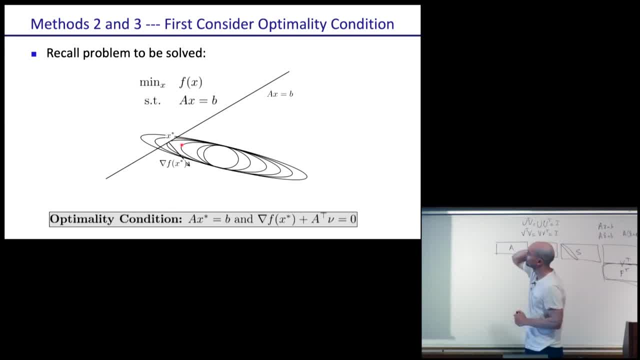 And then from here just to quickly recap, what we conclude is essentially that, even though this condition in general you cannot solve for exactly, if your problem is a second order optimization problem, you can solve it exactly. So we're gonna just turn to a second order. 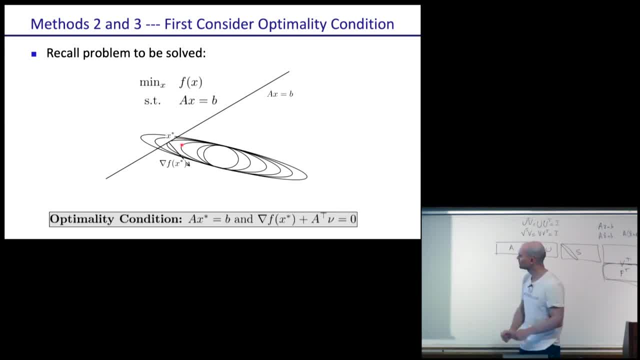 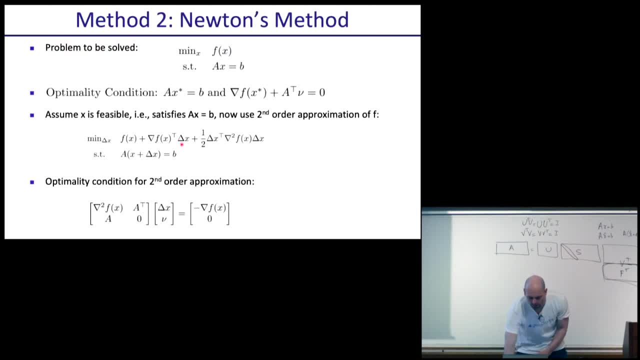 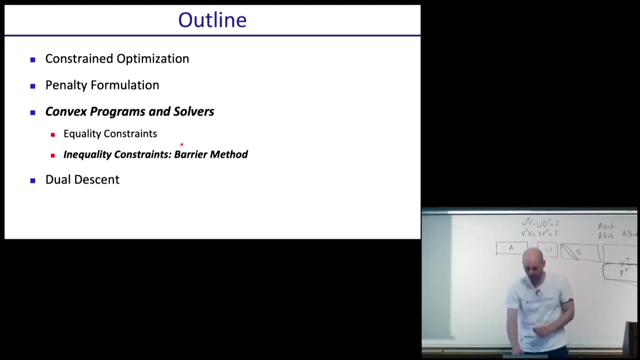 solve it exactly and repeat: If we start feasible, everything will stay feasible every step along the way. If we start infeasible, it'll gradually move towards feasible. Okay, now on to inequality constraints. So we're still trying to solve a convex optimization problem. 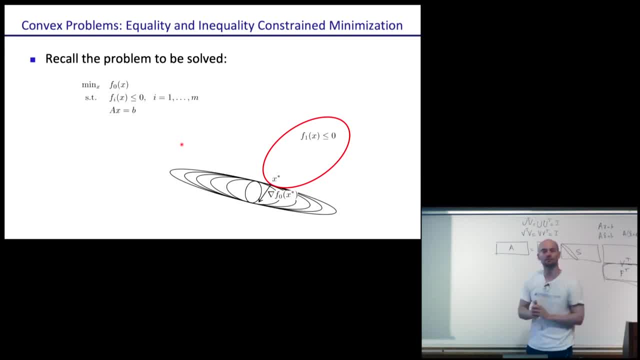 So what an inequality constraint would look like is something like drawn in red here. It's a region where if you take two points in the region, you connect them with a line. you're still in that region. So you're still in that region. 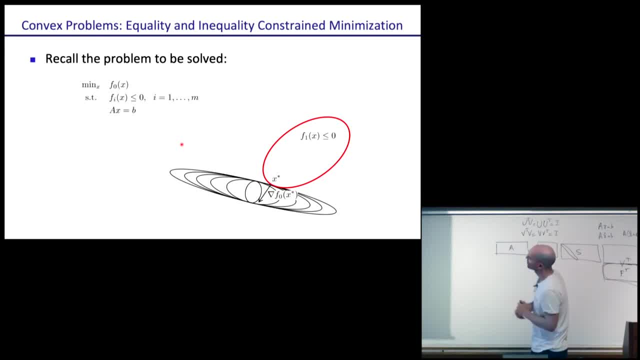 For this problem here. if it was not constrained, the optimum would be in the middle of that set of contours here. but it is constrained. You have to lie inside this region, So the optimal point will be here. We wanna be essentially. 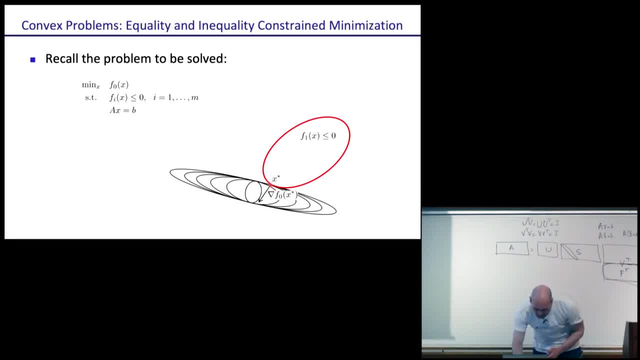 so it's gonna. a situation like this is gonna be on the boundary here, right where it can get to the lowest possible contour. it can probably reach within that set it's in. Now. one thing you might wonder is: why do we treat the inequality constraints? 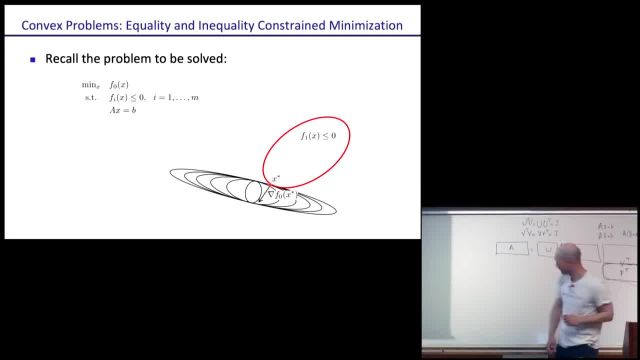 and equality constraints separately, Cause I mean, one thing you could say is: well, isn't it the case that I can just say, well, if I have AX equals AX, I have AX small equal to B, AX bigger than or equal to B. 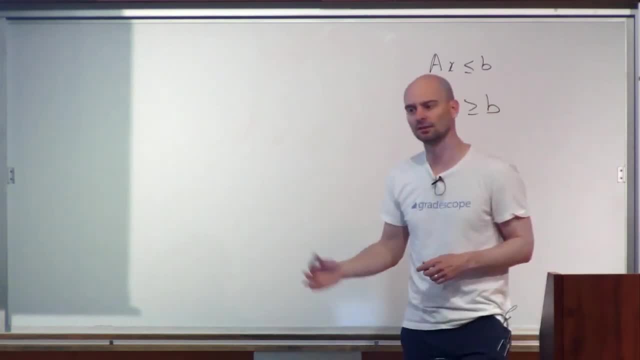 And I can just turn one equality constraint into two inequality constraints and have the same problem. But it turns out that the way we're gonna deal with the inequality constraints in this case is quite different, And it wouldn't really work if we phrase our original problem this way. 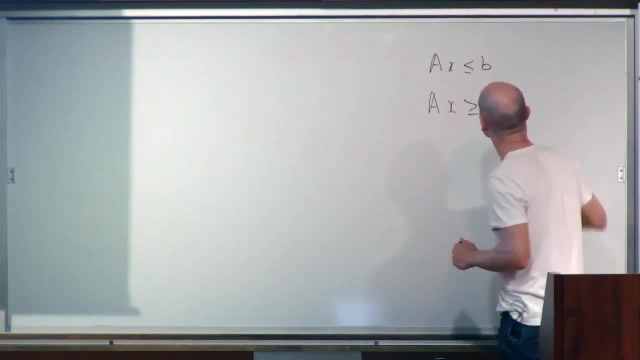 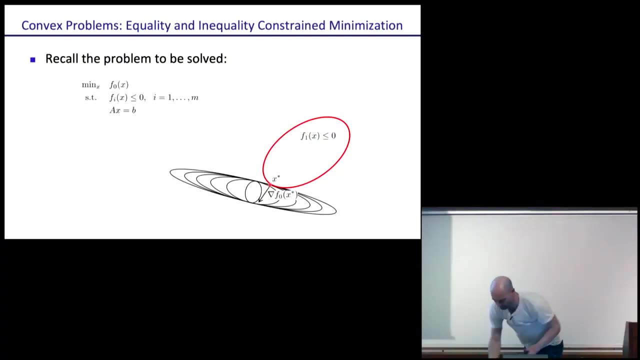 We have to keep our equality constraints the way they are All right. So let's take a look at how we deal with this. There's actually quite a few methods that can deal with solving this kind of problem. We're gonna see a specific method called a barrier method. 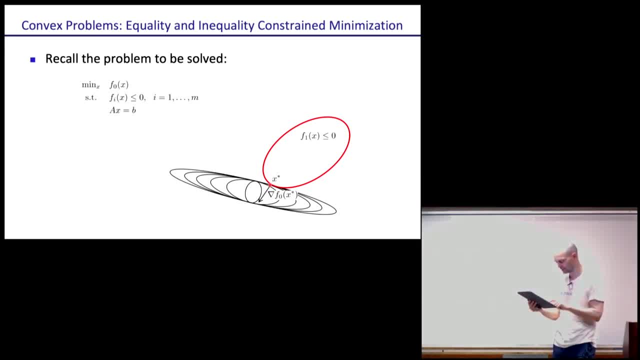 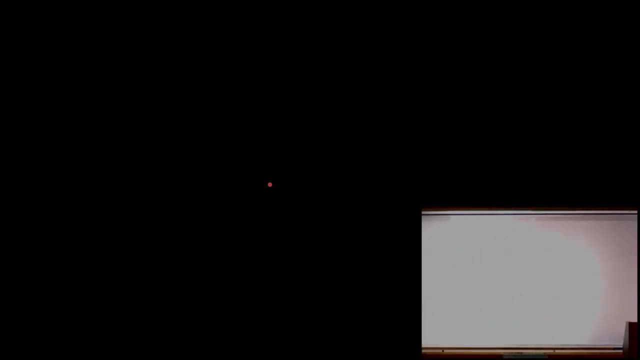 And then later I'll point you to some other methods that you might wanna check out on your own at some point. So let's raise that. The first one is: if we have a weak link into B, then you would've got the link there. 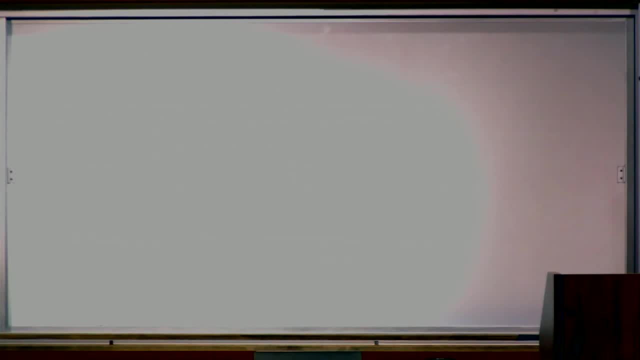 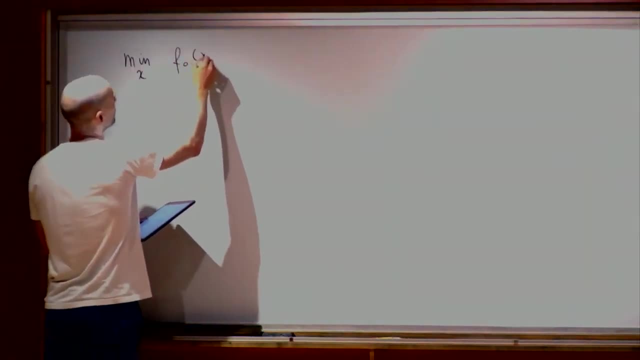 If you have a weak link, then you would've got the link there. I'm actually gonna start with the wrong one and start with this one. So if you have a weak link into B, then you're gonna raise that to up to here. 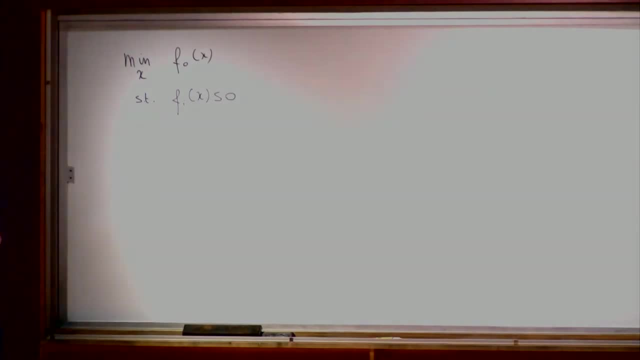 and then you raise that to this one up here. up to here. equality constraints here we can bring them back in using the methods we already have. later We're gonna actually do something somewhat similar to what we did with the penalty method. 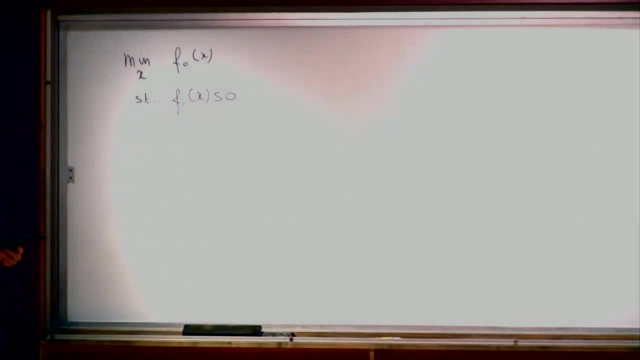 but it's not gonna be the same ultimate solution. but we're gonna say: well, this is a constraint optimization problem, but constraint optimization problems are hard to deal with. Let's see if we can turn it into a unconstrained problem. Well, what could we do? 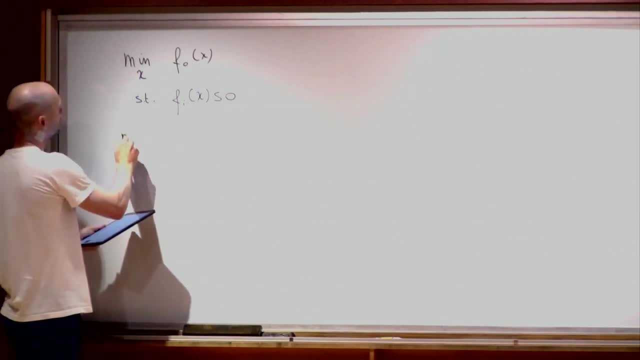 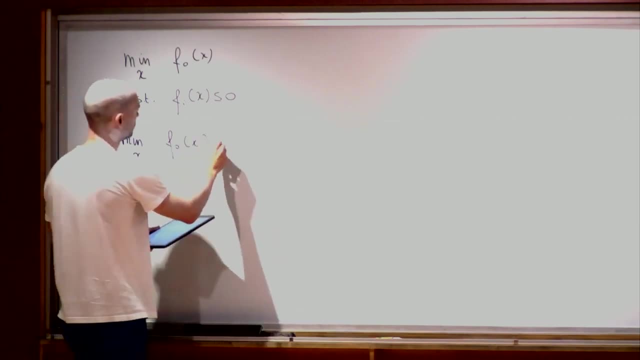 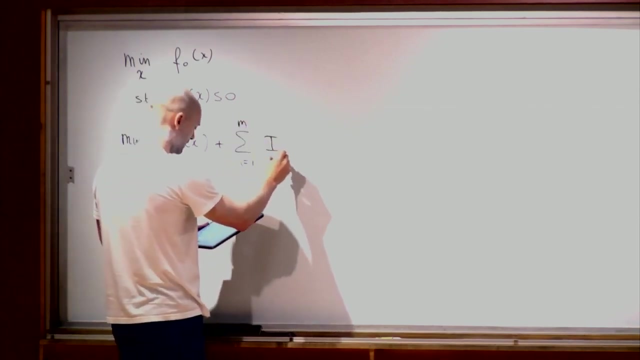 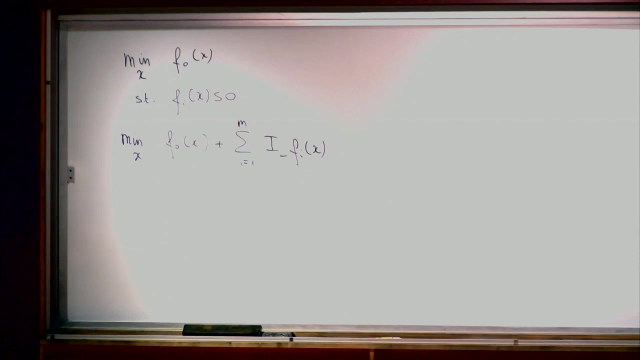 We can say instead: minimize over x over x, f zero of x stays the same, plus sum over all constraints of i negative fi of x. Now remember, with the penalty method we had something similar where we had this absolute positive part of the function. 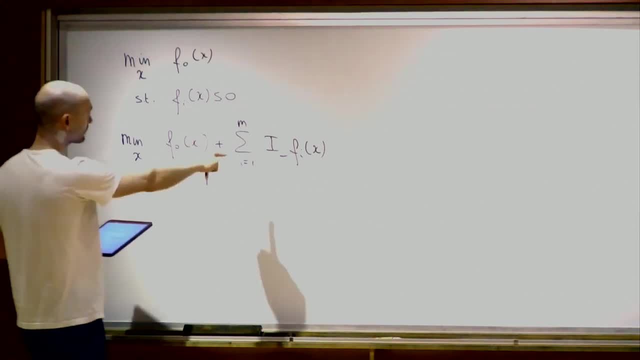 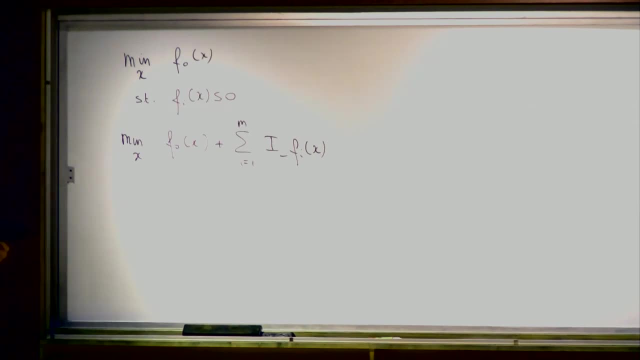 Here it's something different. What is this indicator negative thing? It means that if, if what's inside is negative, we make it zero, So it will not influence the objective, because then we're satisfying the constraint, we don't have to worry about it. 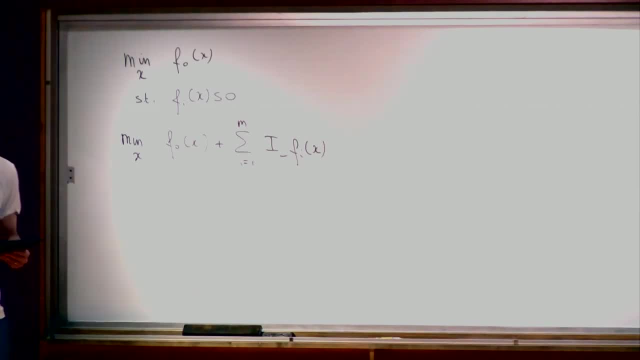 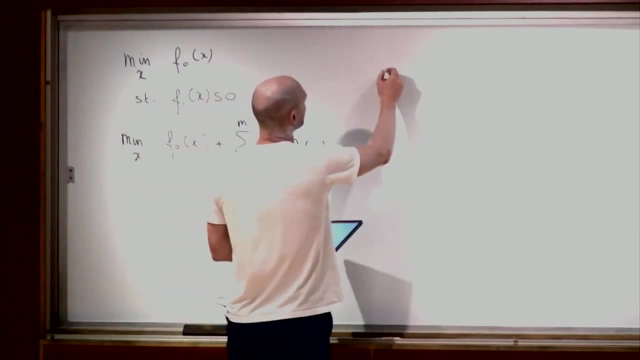 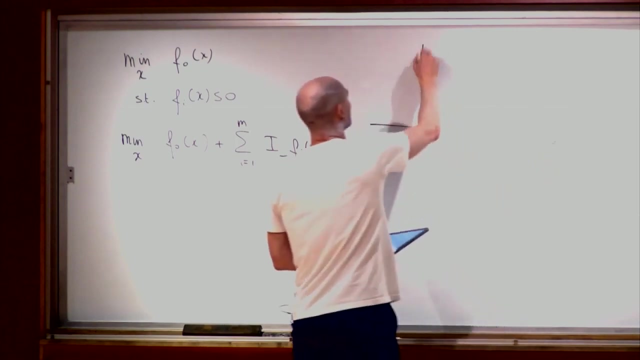 But if it's positive, we make it infinity, Okay. so then this is kind of crazy, but that's what we're gonna do. So we're gonna say our function, if this is f, i of x, living on this axis, on this axis. 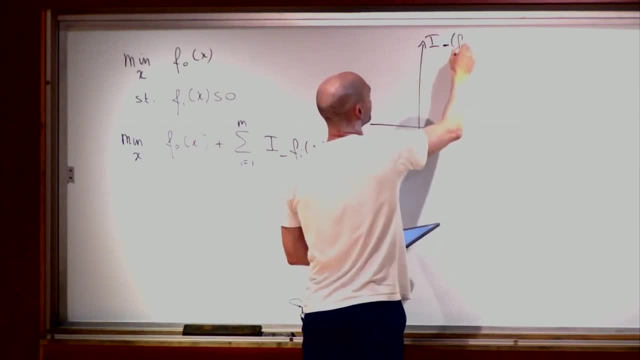 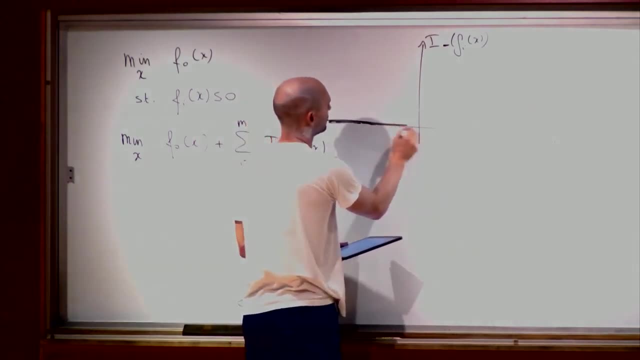 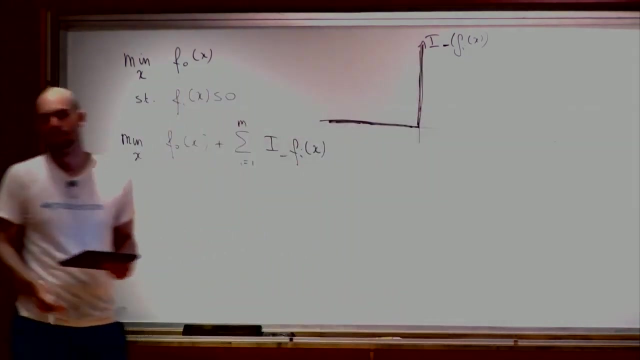 we have i negative of f, i of x. this function will be zero here and then jump to infinity over here. Now let's think about this: If we do this, does this problem have the same solution as this problem? Well, it does. 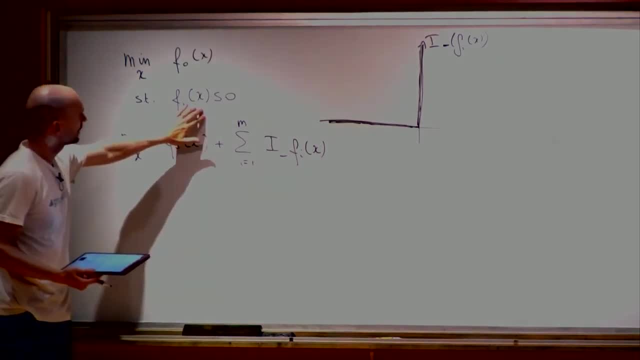 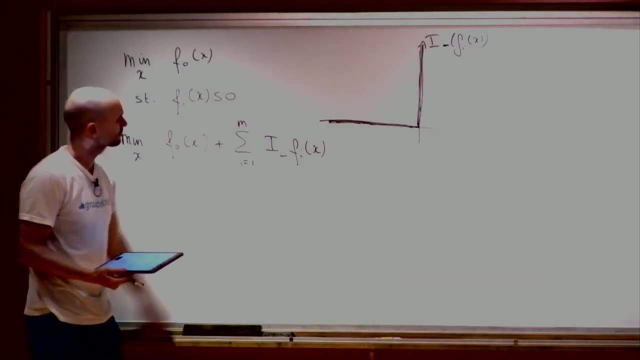 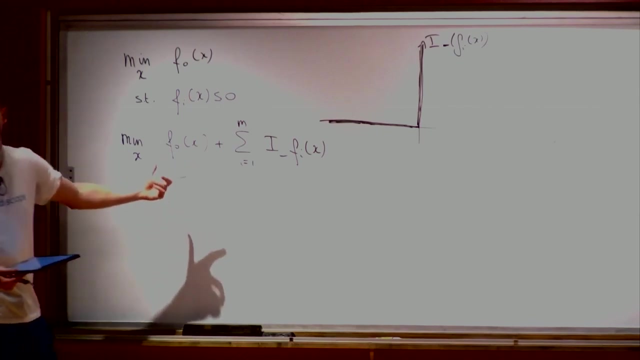 And why does it? Because whenever the constraints are satisfied, it will not influence the objective anymore, And so it doesn't influence the objective. Well then, we're just optimizing this function, and that's what we need to do when we're feasible. 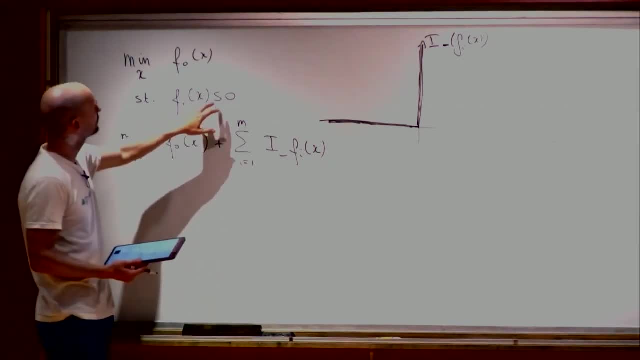 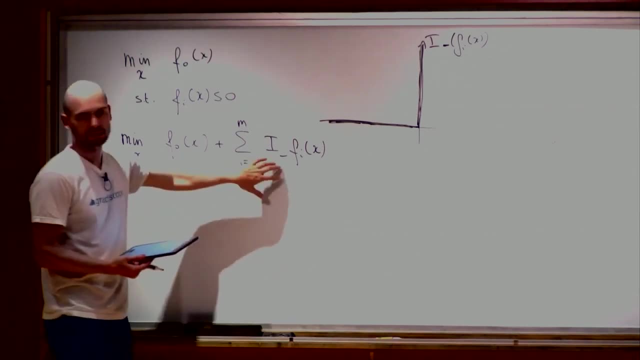 What happens when we're infeasible? One of these f? i of x's is bigger than zero. Well, what happens then is that this thing will be infinity. It makes us very unhappy in the minimization and we'll definitely not declare this. 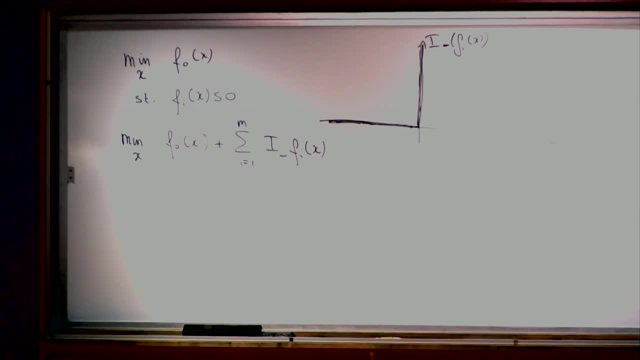 We'll definitely not declare the solution. So these two problems have the same optimum. Okay, why don't we like this formulation? The reason we don't like it is because it's a very poorly conditioned problem. If you think about it, you're optimizing this function: f zero of x. 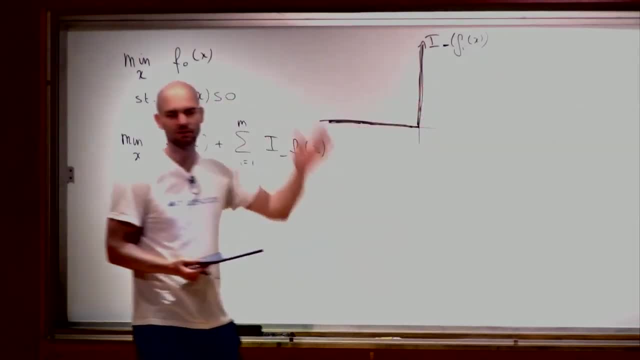 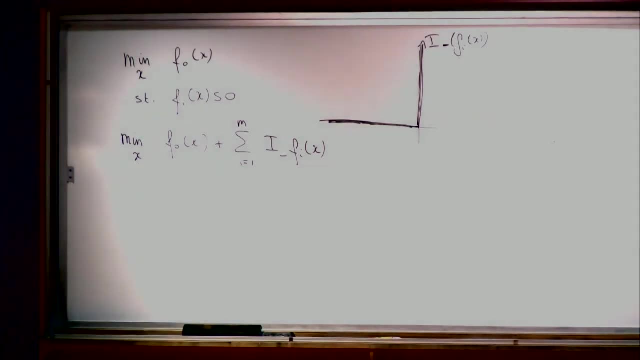 you're moving around and then, once you step a little too far, all of a sudden you're at infinity and you just didn't see it coming at all. And now it's bad, and actually it doesn't even tell you which direction to move. 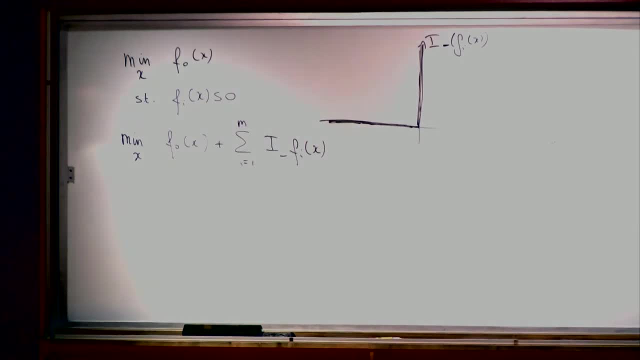 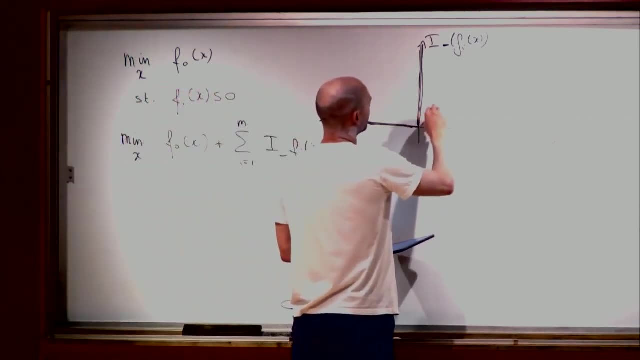 It's like infinity. everywhere where you landed now there's no signal anymore about what to do. Compare that to penalty method, which we saw, where it would actually have a slope going like this, and then, yes, when you cross the boundary you'd be unhappy, but gradually unhappy. 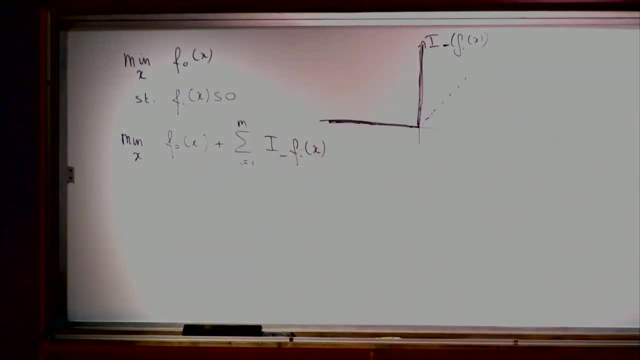 and know to move back to the boundary. Here we're not doing that. We're, in this formulation, making it infinity, but hence that also doesn't really work, because you don't get any signal on where to move. Question is: can we approximate this? 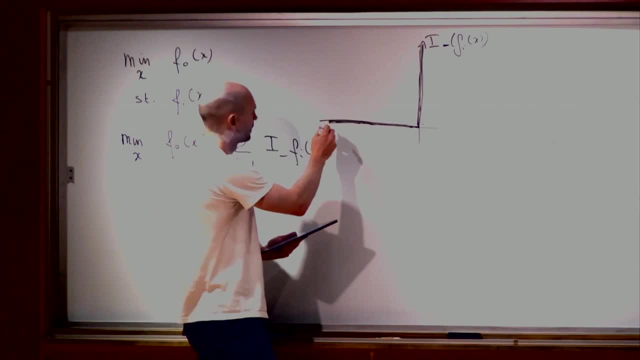 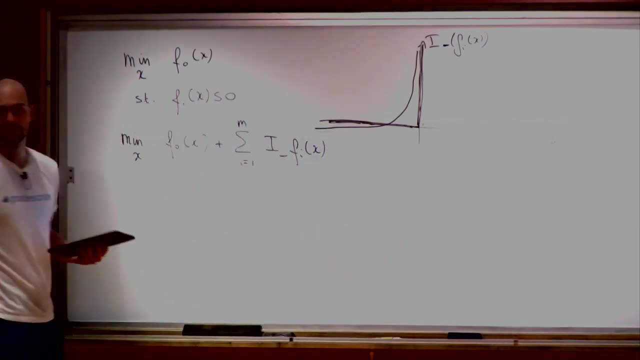 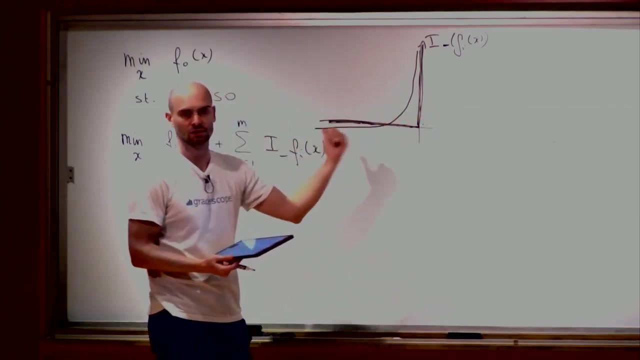 How about if we have a function that maybe is running this way and goes to infinity, but gradually? and so now you'll see it coming. As you move closer to where you're not allowed to be, you'll get more and more gradient force. 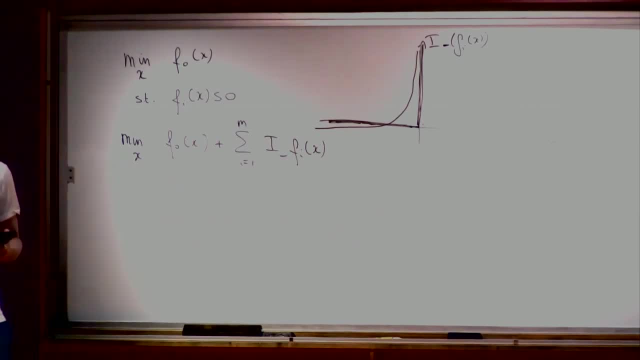 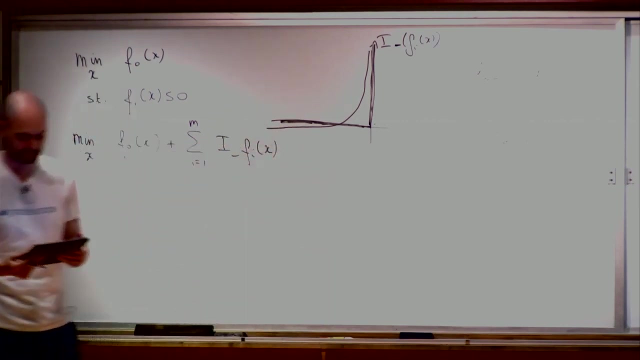 pushing you back in So you could take a function that does this. I'll give you a function. Let's see Log of minus fi of x will look like this. I mean I'm not saying it's, I mean it's gonna be cleaner than what I drew. 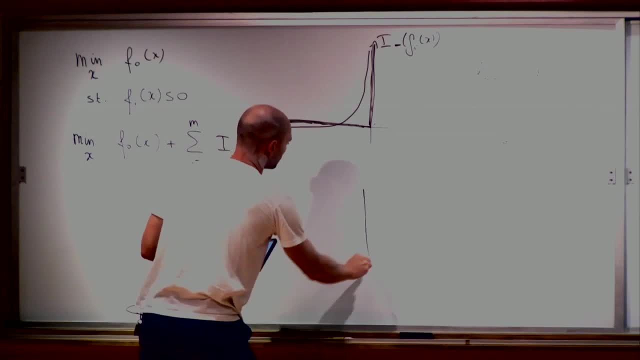 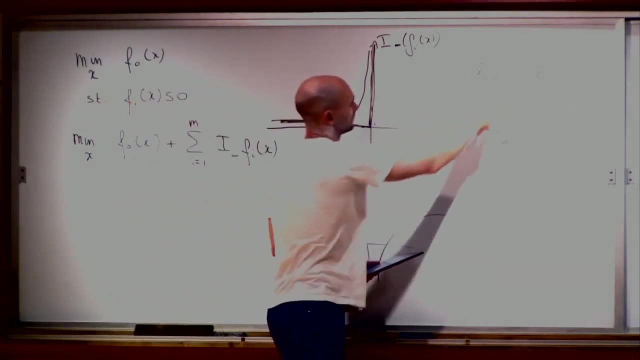 but the log remember log function. the way you're used to seeing it is this way. We're now flipping what's on the inside, so it's negative. so it comes on the other side. It's not living there anymore. 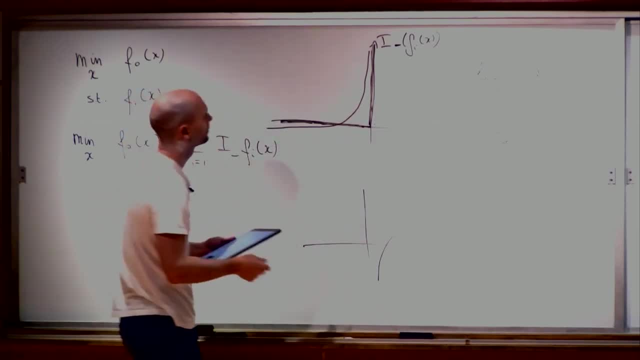 It's living on this side now and then actually the other thing we're doing, we're actually putting a negative sign in front to flip it the other way. so essentially flipped it this way and after we flipped it to this side, 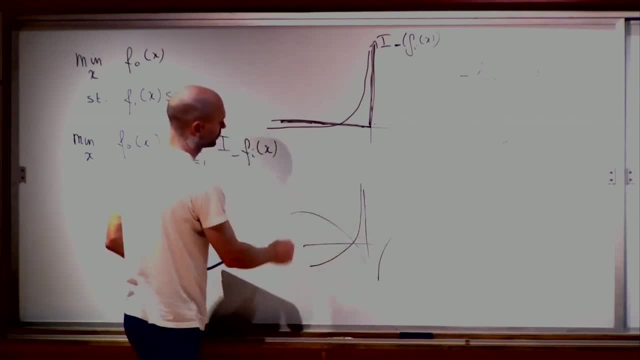 we then flipped it vertically and we end up with this function over here. which is this function? here is log minus log of negative x. So that function has the right properties. It goes to infinity at zero. so you don't wanna. 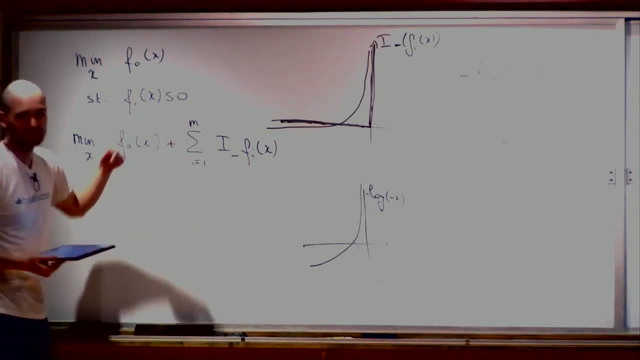 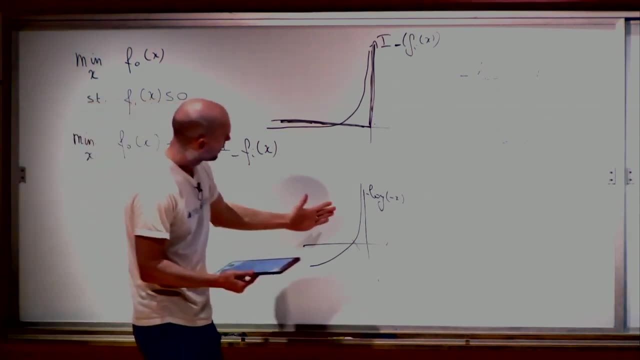 I mean, it's maybe not ideal. ideal because you say, well, I'm allowed to be zero, but you know what It's gonna be. fine, If you can be just epsilon away from zero, it's good enough. so it goes to infinity there. 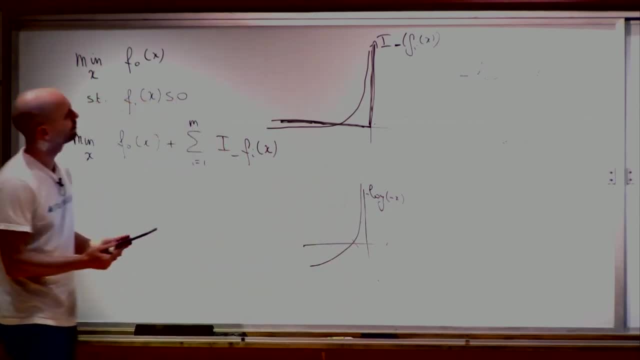 See you wanna stay away from it and you get signal. Now the tricky part is that it does have quite a bit of signal and it'll kinda keep you maybe too far away from the boundary. You might say well, anywhere here. 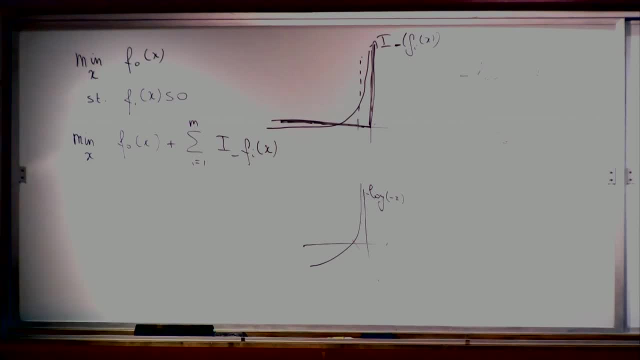 I'm probably never gonna end up. It's just too high cost in this new problem. so if I write min x, which is the new formulation, min x of zero, x plus, well, minus, because we have a negative sign in front of it. 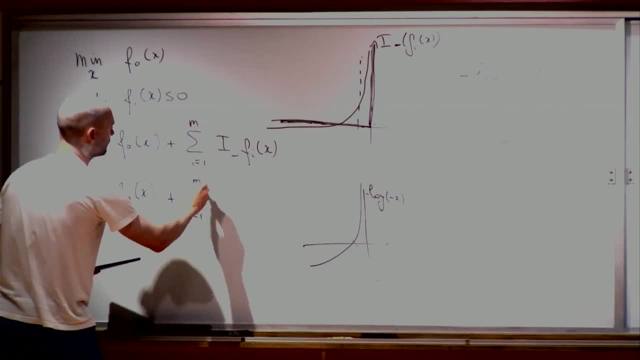 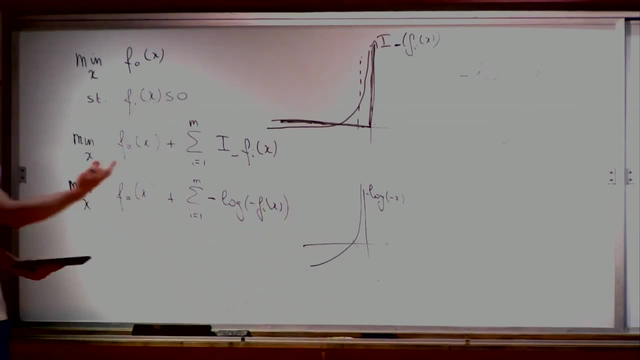 plus sum over i one through m negative log of minus fi of x will be kept away too far from the boundary to truly find the optimum. Yes question When you, if you output an x that does cross over to the positive axis. 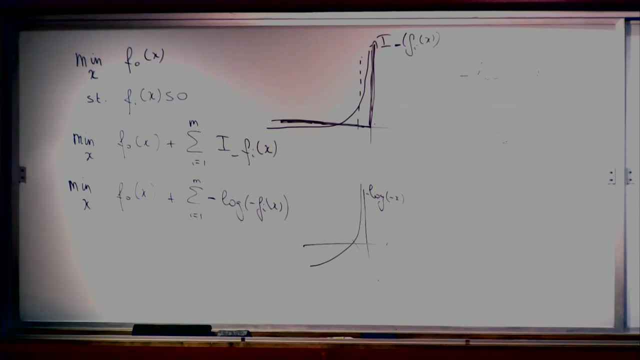 You're not allowed to In this method. you're not allowed to, and actually when you? this is a really good question If you can already imagine that we're gonna run a gradient method on this new objective or something like a gradient Newton's method and so forth. 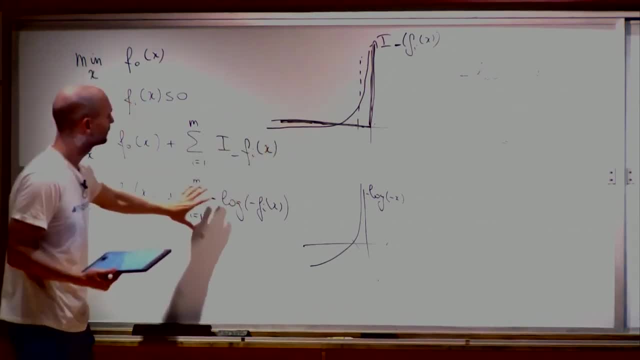 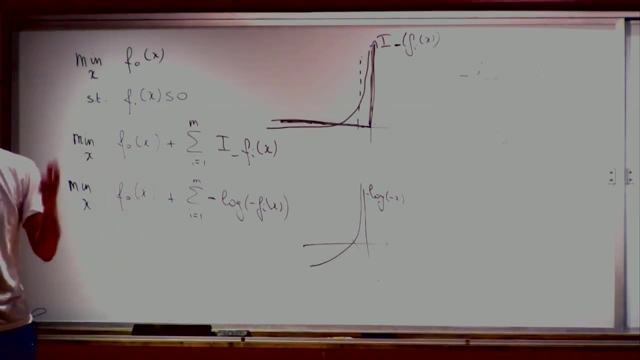 and if you take your step size too large on this new objective and you land on the other side, you're backtracking line search. Part of the backtracking line search has to be backtracking when it tells you infinity and consider it's still infinity past here. 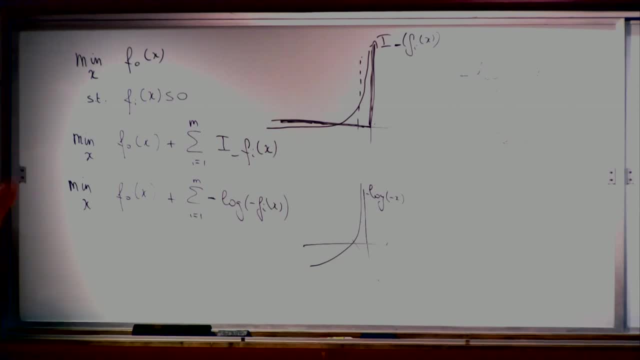 It'll give you not a number or something in practice, or a complex number, because a log of a negative number will be a complex number depending on the implementation you're using. Then you gotta check for that and definitely it's a kind of common thing. 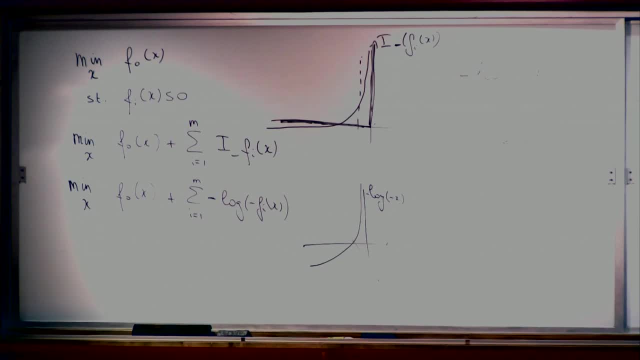 that can go wrong. You don't check for it and then, all of a sudden, everything's complex numbers in your optimization and you wonder where they came from. Well, they came from the fact that you took the log of a negative number. 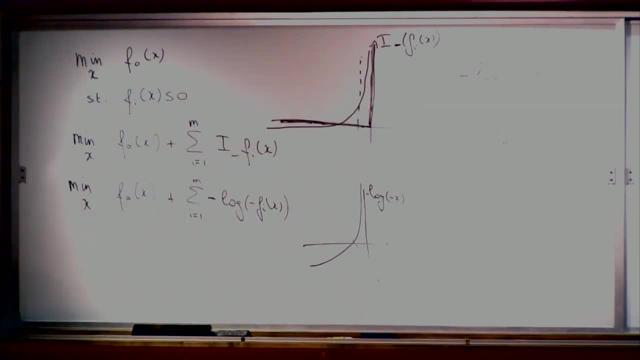 and they just start showing up. So that's something to be really careful with, absolutely, And so it's the backtracking line search that's supposed to catch that. It also turns out that for convex problems, there are certain things that you can do. 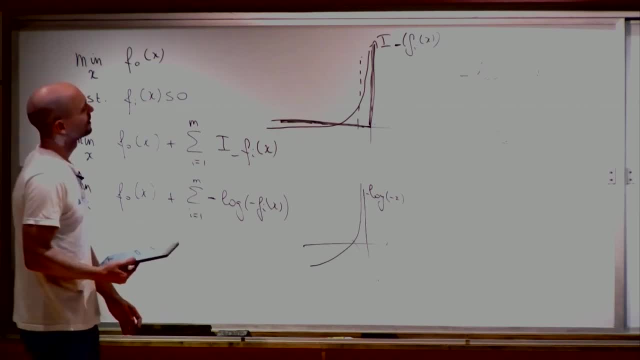 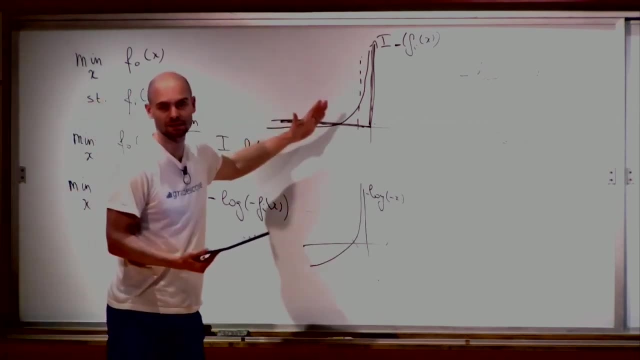 and there are certain guarantees. So there are certain guarantees that if you apply Newton steps, that it will actually not for the right kind of function living here, and log is one of them. there are other options, but log is one of them. 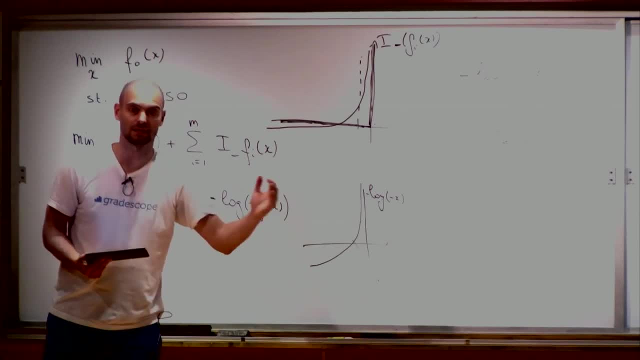 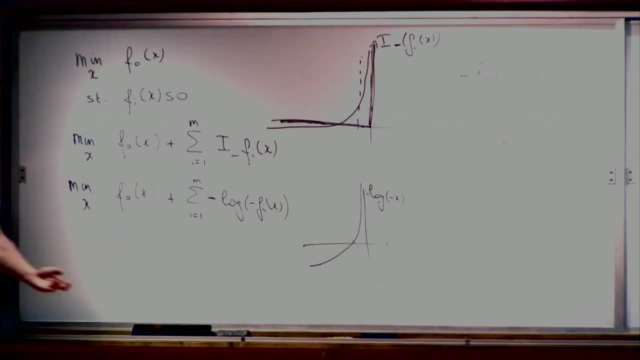 that your Newton step will not get you beyond the barrier. It'll automatically keep you on the inside. So you would not have that issue. But if you use gradient method rather than Newton's method, then the step size is somewhat arbitrary. 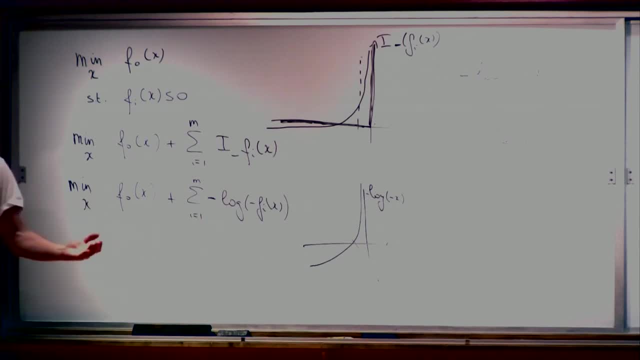 because we know when you rescale the problem you get a different step size just by rescaling the problem. So then you don't necessarily have those guarantees. You need to be very careful. So this problem will have a different solution from this one or this one. 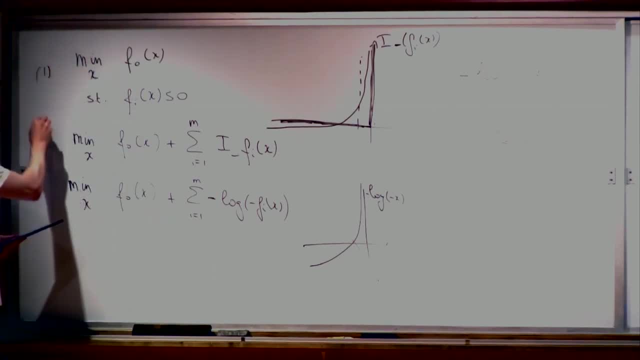 because these have the same solution. These two, one and two, are equivalent. Three gives us a different solution. But can we get closer? Well, the way we can get closer, by saying: well, minus log, minus f of x. 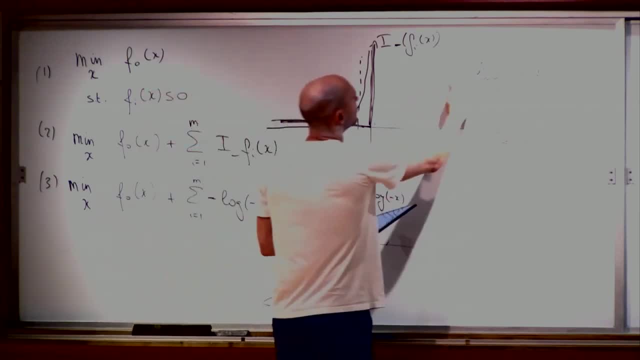 what if I actually rescale it? What if I actually rescale this? What if I put a minus one over t, for t, a positive number of log minus f of x? What happens? Well, let's think about it. If t is one, we have what we had before. 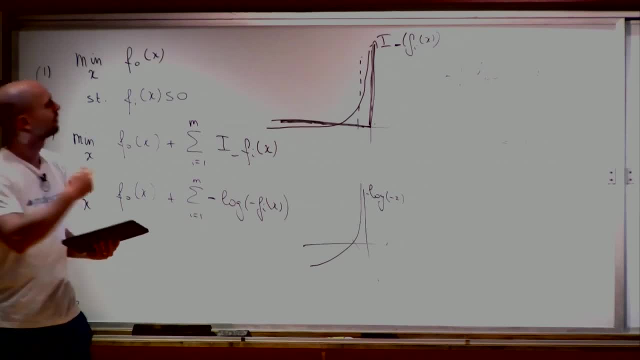 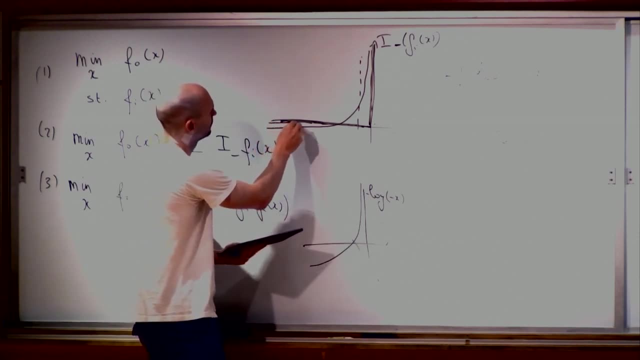 Now let's make t bigger, which brings us to a coefficient in front of this, bringing this closer to zero. So this function here then will run closer to zero. It'll still cross over always that Where the inner thing is one. 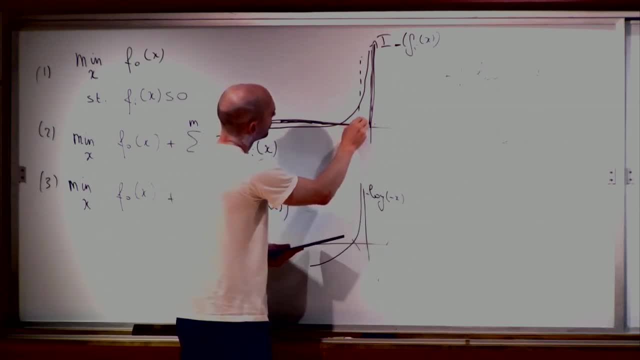 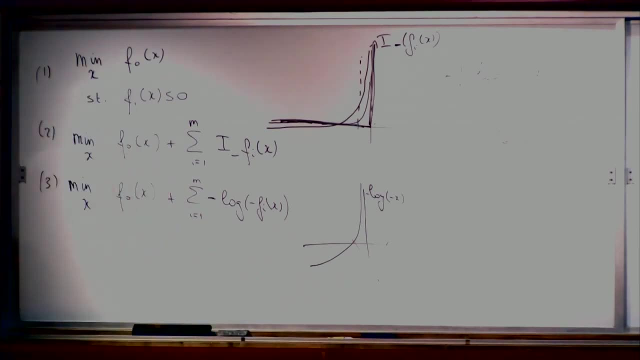 Then after here it'll stay closer to zero and shoot up later, And the bigger we make t, the more we are really multiplying with something close to zero and the more this function will be very close to being exactly zero here, just slightly below. 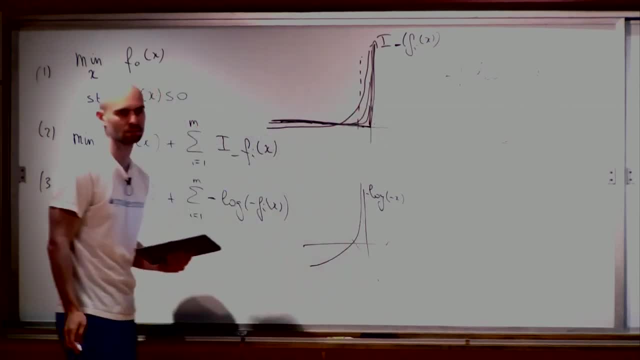 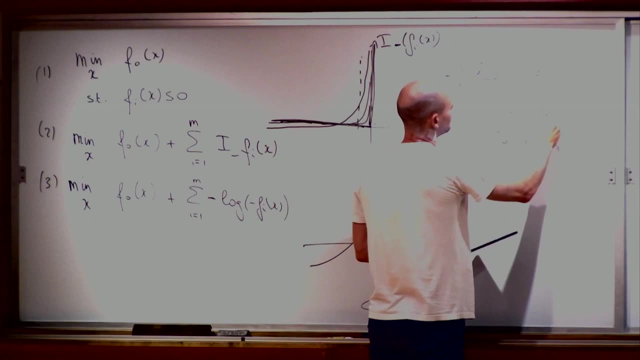 and then slightly above here and then only at the very end shoot up. So we can then say, well, okay, we got it. Just set t equal some large number, And then the problem will be almost equivalent to the original problem. 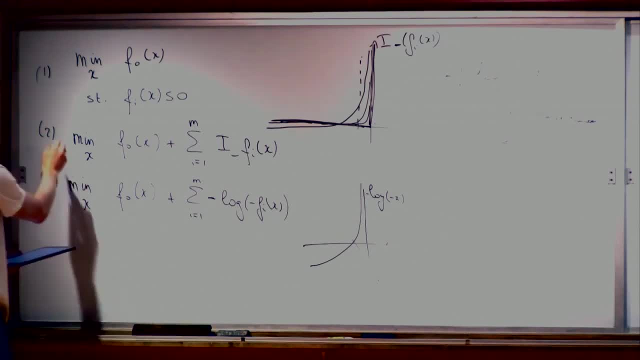 If we make t really large, like infinity, then you're actually back to problem two. So the limit of t going to infinity, you get problem two. But we also know in problem two we get no signal, And so intuition should tell you that. 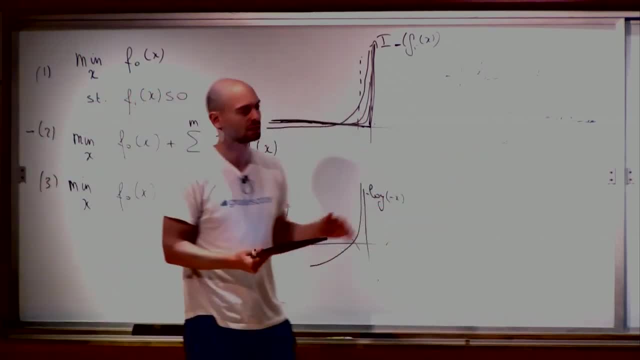 well, actually, what we should be doing is not just set t really large, because the larger t, the less signal we get in our optimization. So what we're gonna do here is we're gonna say, well, I'm gonna do something gradual. 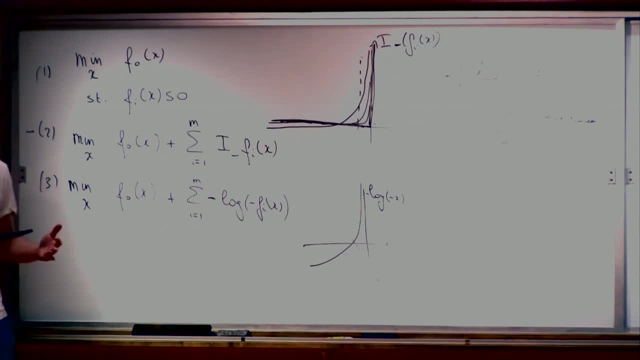 Start with a t. that's pretty small, where you get more signal about the shape, how your optimization problem is shaped, especially the constraints, because that's where it comes in. And then, as you solve it, for a small, initially for a small t, you've solved it. 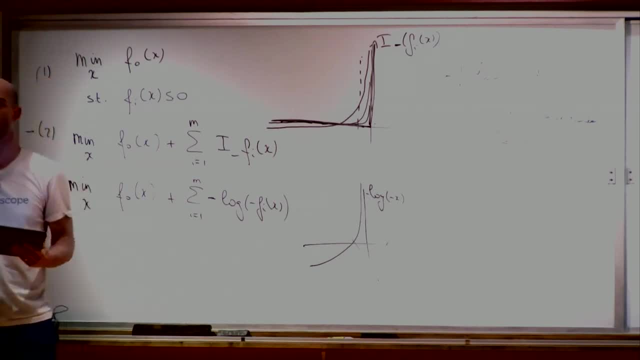 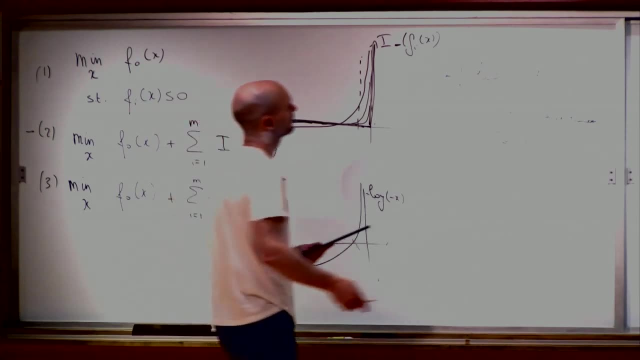 you make your t larger: repeat, repeat, repeat. So just like in a penalty method, we're driving up mu. here we're gonna be driving up t Funniest notation. for some reason, the way the notation is here is like: 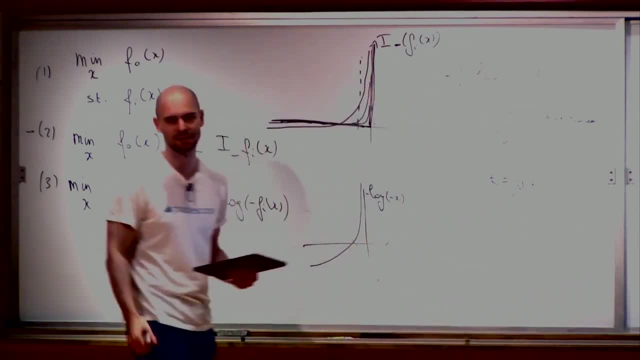 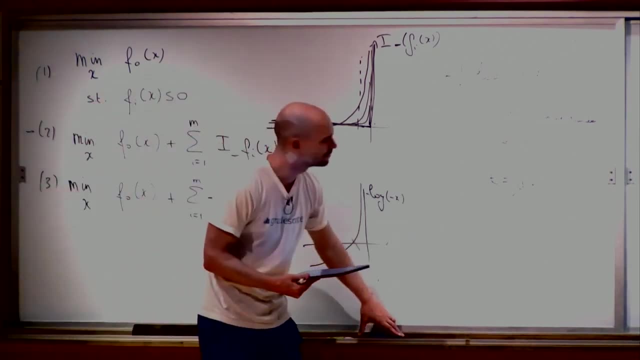 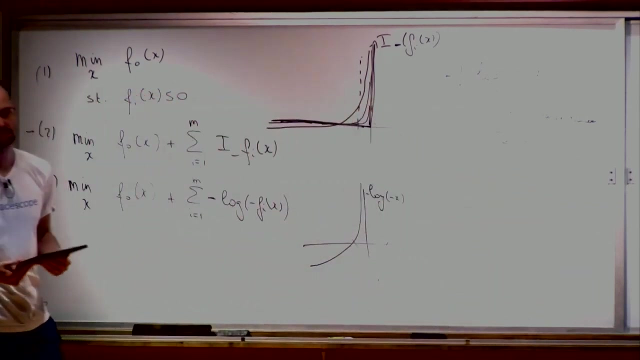 t will be mu times t in every iteration, whereas before we had mu equals t times. it was just standard notation that different literatures kind of, I guess, mix up the t and the mu and use it for the opposite thing. Okay, so any questions about this? 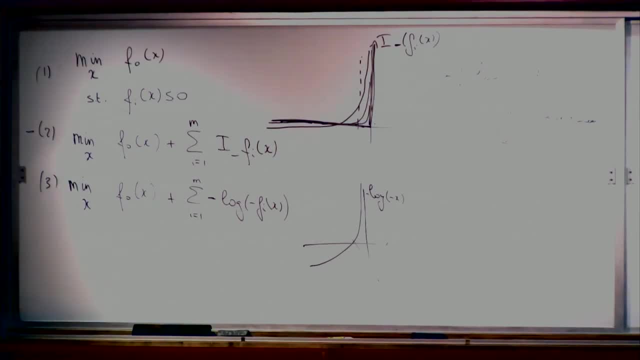 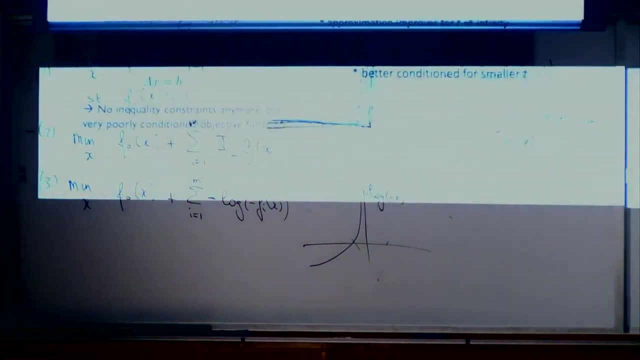 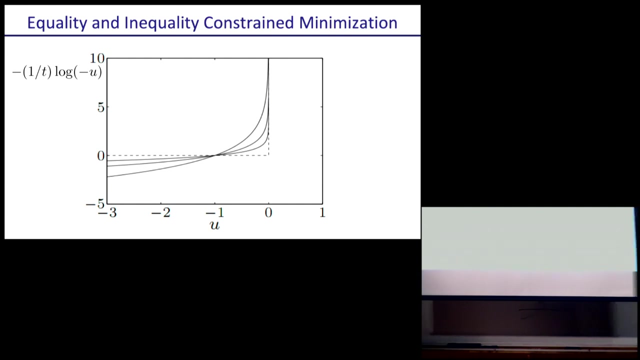 This is probably the main idea for the first half of lecture. All right, let's look at some results then when using this. So here's the slide showing the thing we had on the board. Let's zoom in on that plot as t becomes larger. 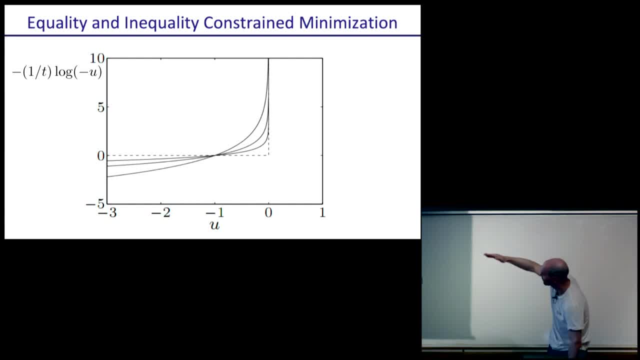 This thing gets closer and closer to horizontal first and vertical later. It's called the barrier method why? Because you put up this barrier that you're not supposed to go past, So you're supposed to start on the inside of it and never go past that barrier. 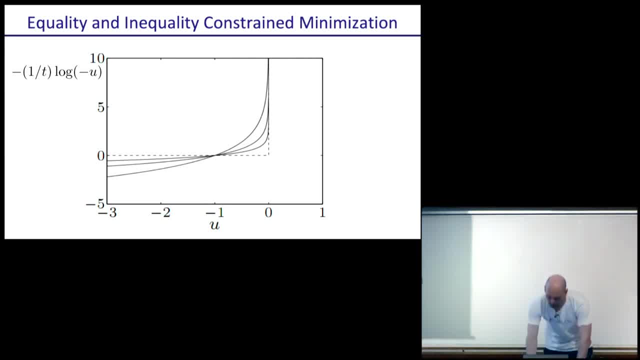 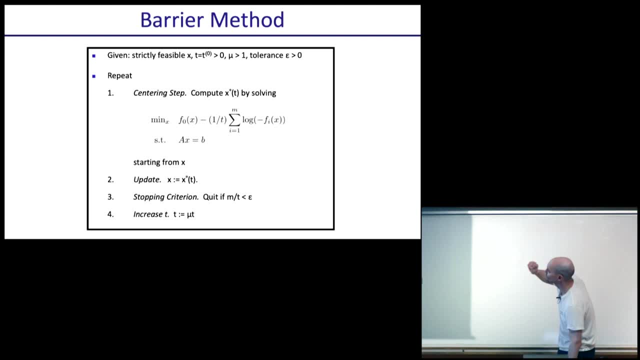 and it keeps you from escaping because it gets. it's pretty steep. What's it look like? Okay, you do a centering step. it's called You compute x, star t, which means the optimal solution for this surrogate problem here. 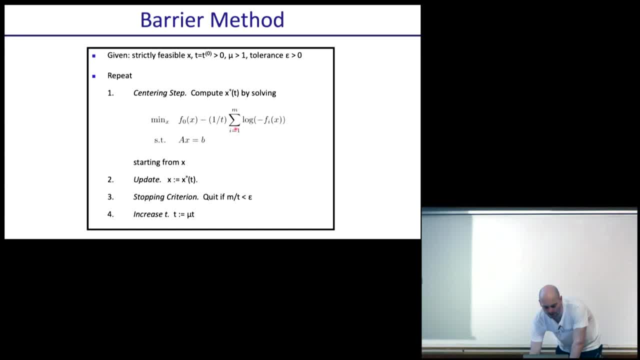 It's not the real problem. it's a surrogate problem, but it's close to the real problem. Solve this problem And you can still have equality constraints. We know how to deal with that. So now it's just a convex problem with equality constraint. 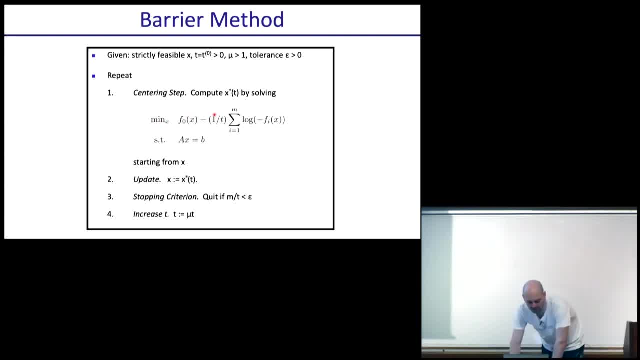 No inequalities anymore. It's not the original problem, but at least it's related. Once we found x star for that specific choice of t, we check the stopping criterion. Essentially, if our t has become really really large, then we're ready to stop. 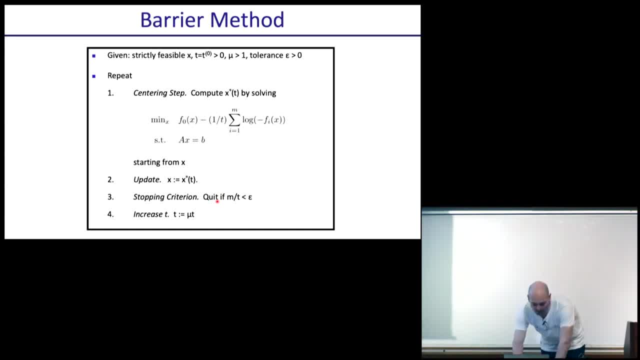 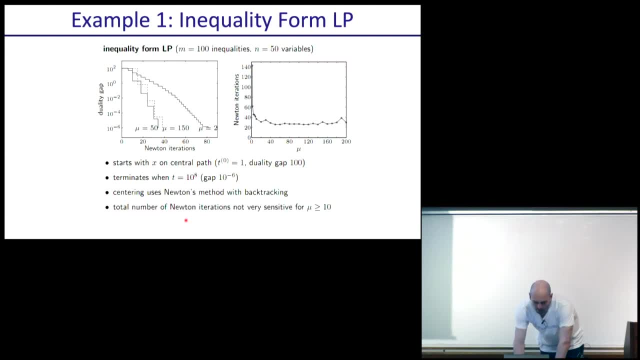 because we have pretty much the original problem. If it's not that large yet, then we increase t by a factor mu, and repeat. Here is this applied to solving linear programs, which is linear objective and linear inequality constraints and linear equality constraints. This was done with Newton's method. 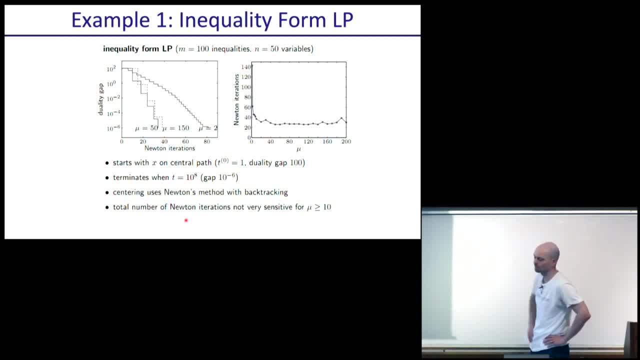 So Newton iteration is shown on the horizontal axis. Duality gap is distance from optimality measured in a specific way. It's on the vertical axis, logarithmic scale. We see we get this kind of quadratic conversions, just like we had with unconstrained problems. 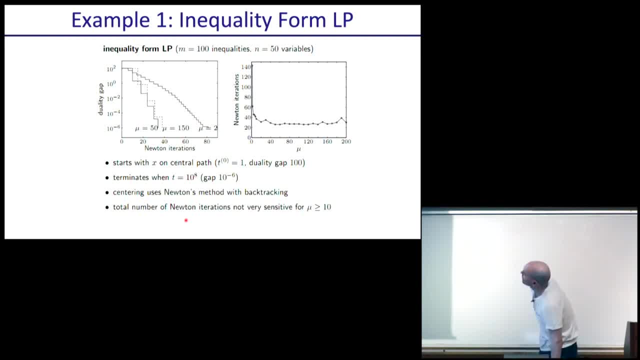 And we see it's not super sensitive to the choice of mu, but mu in the range of 10 to 200 seems to be reasonable. If you go below 10, that's the graph on the right. if you go below 10, the number of iterations you need. 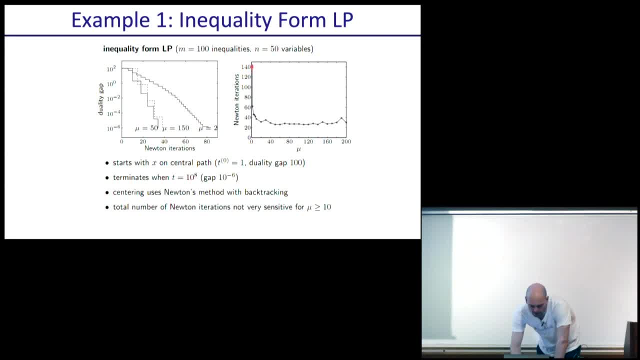 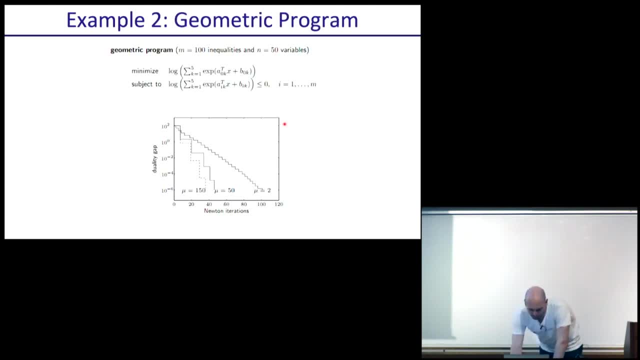 to get to meet. your optimality criterion is very large, 140 here versus just 20 here. So set mu larger than 10 for this kind of problem. Here's another one, The metric program, which is another convex program where you have log some exp in the objective. 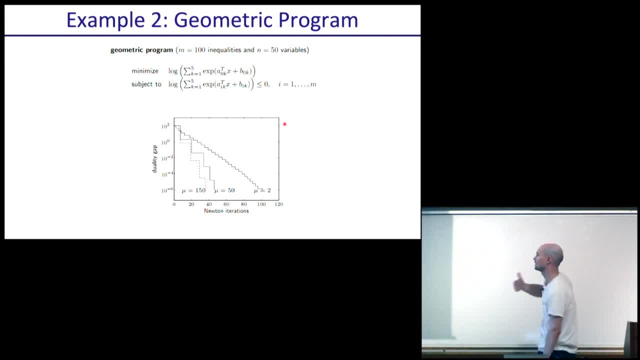 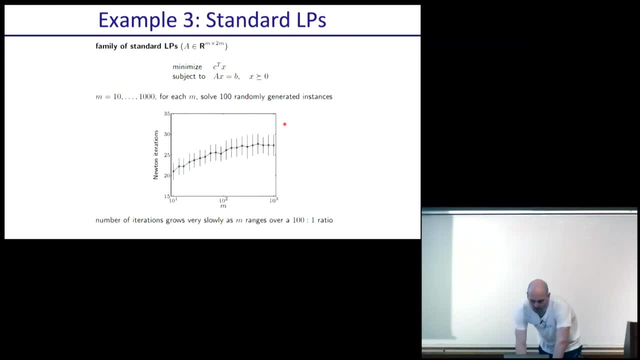 and log some exp in the constraints, You can run the same method and again converges in a very small number of iterations. Standard form LPs can be solved this way. What's interesting is that it doesn't really slow down. So m is on the horizontal axis. 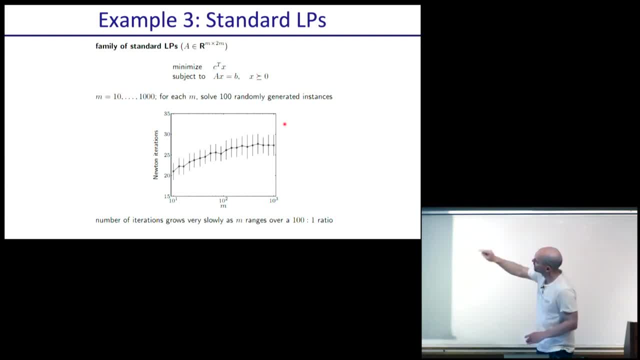 counting the number of constraints And the speed of solving this in terms of number of iterations needed. it doesn't go up much with the number of constraints, So it's fairly invariant the number of constraints, how fast you can get centered. 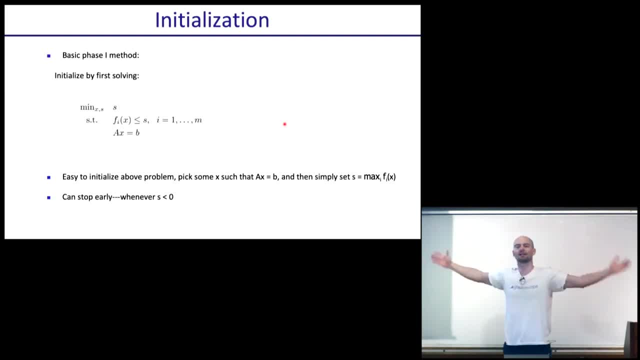 Initialization might be something you worry about, because for this thing we cannot be outside of the barrier, We need to be on the inside. How do we do that? Well, here's a simple trick: You solve this other problem first, which is called phase 1.. 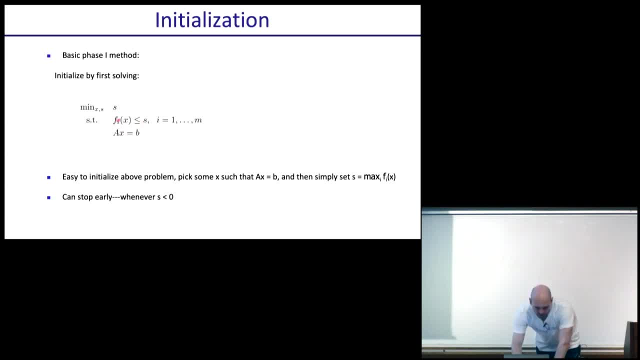 Original problem was you needed these to be satisfied in AX equal. but you didn't solve this problem first. You solved this other problem first, which is called phase 1.. And this will be well, you can just say: I'm choosing some arbitrary X. whatever I pick something. 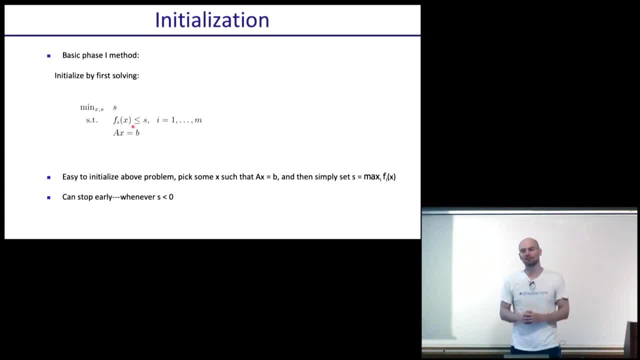 I then check what is Fi of X. for each Fi I see which one is the largest. I set S equal to the largest one And now I say, okay, now I have a new problem where I'm gonna start minimizing S from that starting point. 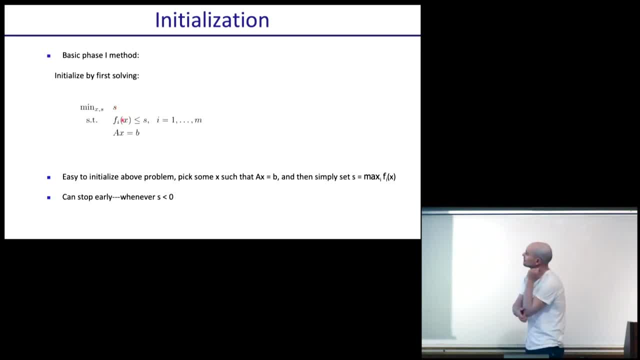 but I start feasible. So what I did is I said I wanna find in some sense the most feasible point, Because minimizing S means you might bring this below zero. If you cannot bring it to zero, then it's just an infeasible problem. 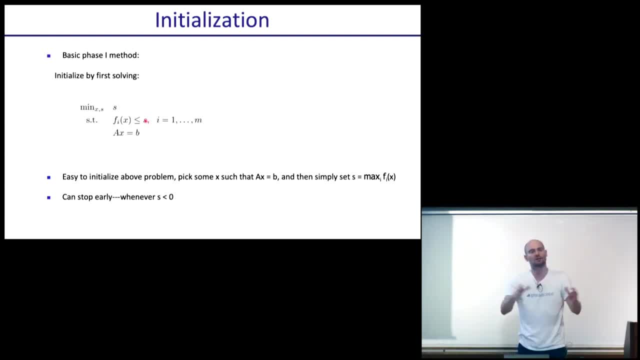 But if you can bring this below zero, you're kind of in the most feasible part of the space, the centered part of the space, ignoring the objective. You just wanna get centered, And so this one we can solve very effectively, because we can initialize by just making S large enough. 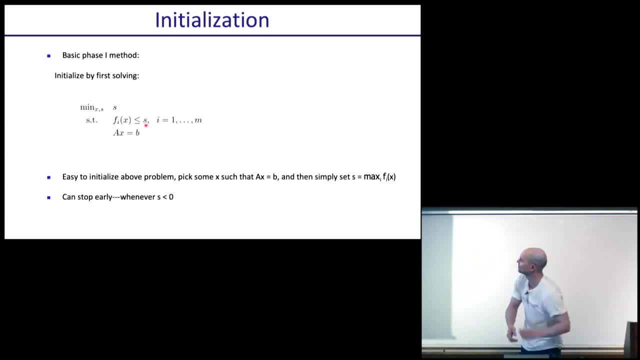 And then we're good to go. So that's a little trick here is we replace the zero on the right-hand side by a S, make it large enough, find the things that's most centered, and then we're good to go. 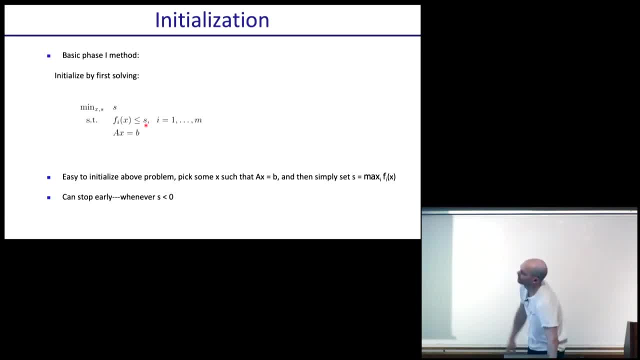 So that's a little trick here is we replace the zero on the right-hand side by a S, make it large enough, And then we can start the phase two, the actual optimization, Having just one S. here is one way to do it. 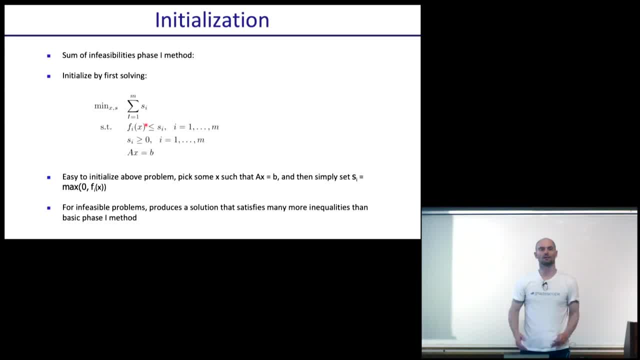 You could also have a different S for every constraint. That way you're kind of paying more attention, in some sense, to constraints that are harder to satisfy, and it might be slightly better conditioned Ultimately when you do this. the main advantage of doing it this way is that 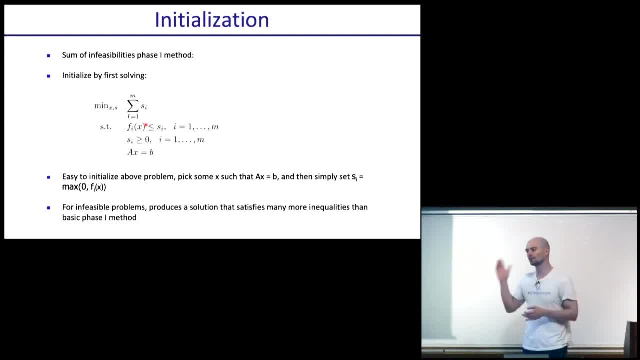 if your problem is infeasible, it does not have a solution. it'll help you identify which constraints are causing the trouble and making it not possible to be satisfied, And you can go back and say: well, is this even a problem I should be trying to solve? 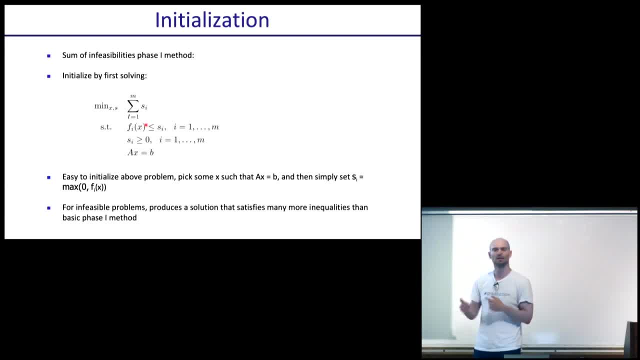 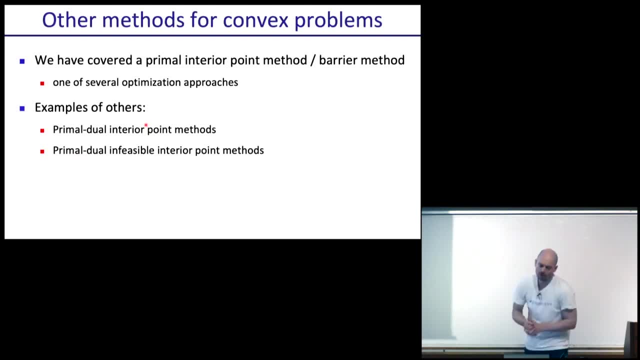 because apparently it's not feasible to satisfy all the constraints. You can change the problem you're trying to solve and go again, Okay. so what are some other methods for convex problems? What we've covered is a primal interior point method or a barrier method. 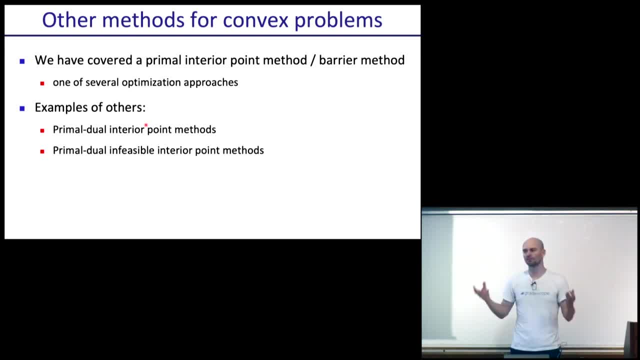 What it means is that we're always in the interior of the feasible set while we run this method. It's primal, because we only pay attention to the X variable. We know when there's constraints, you can form a Lagrangian which introduces dual variables. 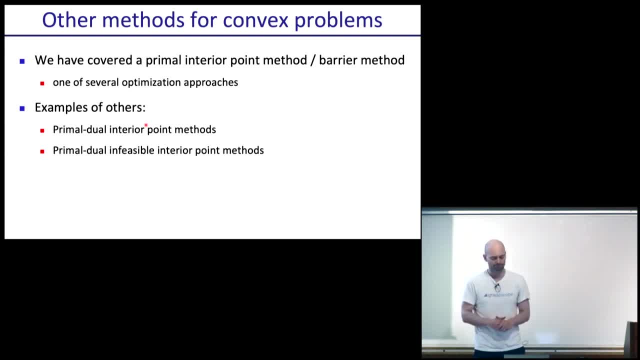 and we don't pay attention to those in this method. So that's one of several ways of solving this kind of problem. There are other methods that people use that are, I would say, a little more intricate, but they could be of interest to you at some point. 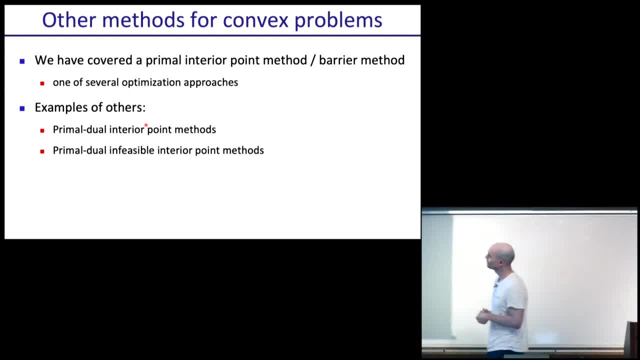 Primal dual interior point methods. it's well, it's, you know, it's where you have the same thing happen both in primal and dual space. So you have a feasible dual space, a feasible primal space and you solve for both variables at the same time. 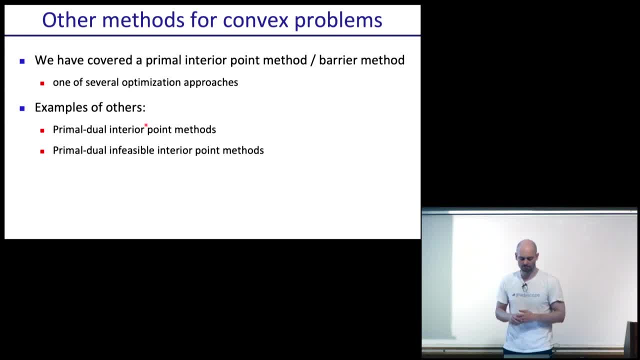 Then primal, dual, infeasible interior point methods. essentially, they will say: I still need to be feasible in terms of the inequality constraints, but my equality constraints I can violate, like we saw before, with just equality constraints set up. and that's what they will do. 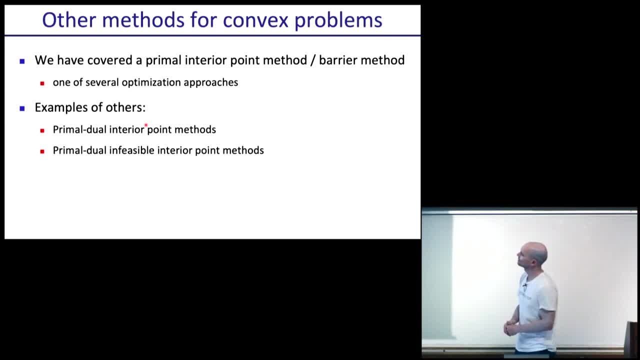 So there's a few different ways of solving these kinds of problems. One of the reasons you might care about solving the dual at the same time is because there is a property that says that the primal problem will be this convex ball. the dual problem will in some sense be this like: 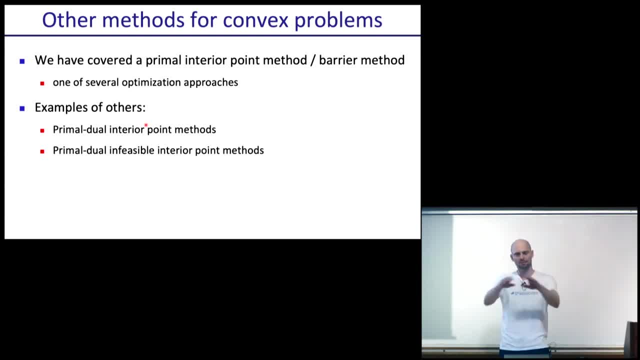 oppositely shaped ball living below it and at the optimum they will touch. And so as you check in your dual space what your value is, it's taking the primal space where your function value is. the difference between them is the upper. 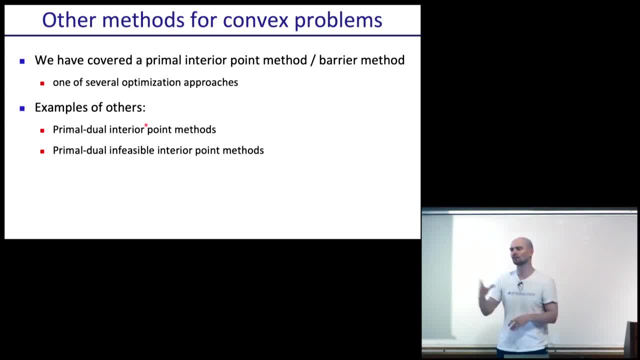 and the lower bound on how far away you are from the real optimum, And so, by solving both the primal and dual at the same time, you actually get this information about how far away you are from optimum, which is often nice to have Any questions about the barrier method. 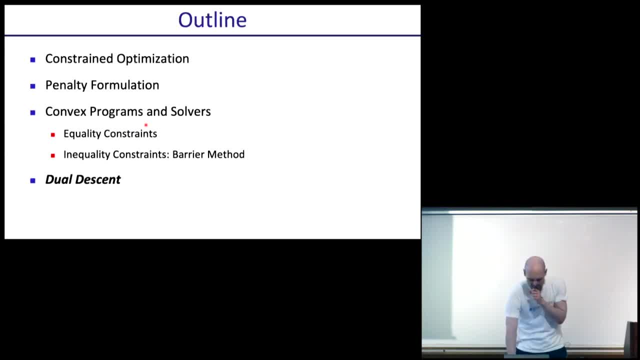 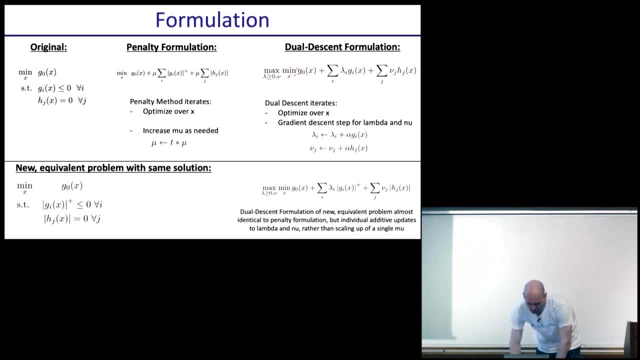 Then the other thing we covered at the end last time was dual descent. This is yet another way to solve a constraint optimization problem, shown in the top right here. What I didn't have on the slide last time was the explicit update: Like in dual descent, you optimize over x. 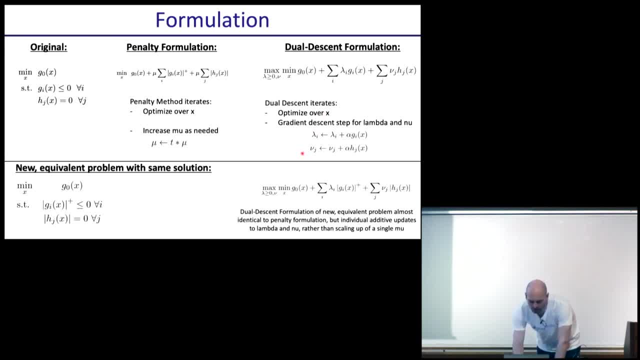 once you're done optimizing over x for a current choice of lambda and nu, you update them with gradient descent, which is just as simple as actually gradient ascent, because it's maximizing just these updates over here. That's all you have to do for the dual variables. 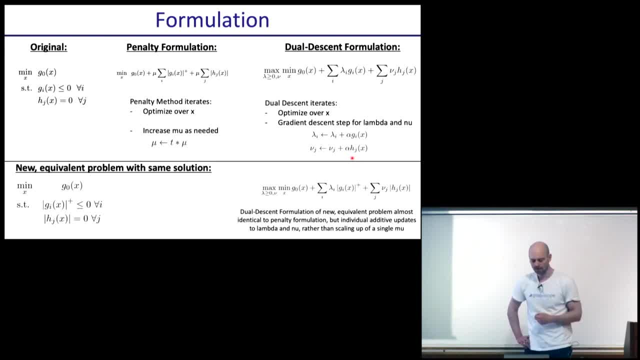 and then you solve again for x and repeat. Thing I alluded to and also didn't have on the slide is the bottom part here- is that this original problem is a new equivalent problem with the same solution If g of x has to be smaller than zero. 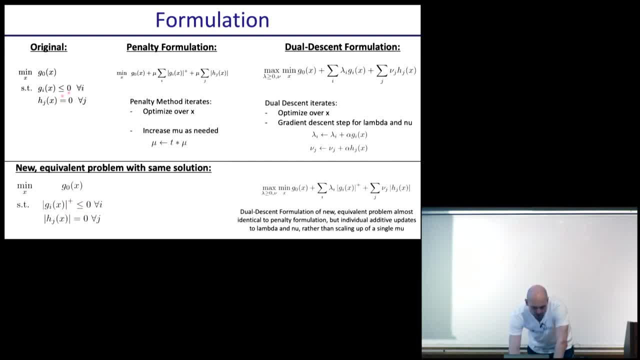 then the positive part of g of x has to be smaller than zero. If h g of x has to be equal to zero, then the absolute value of h g of x has to be equal to zero. So then we can form a Lagrangian. 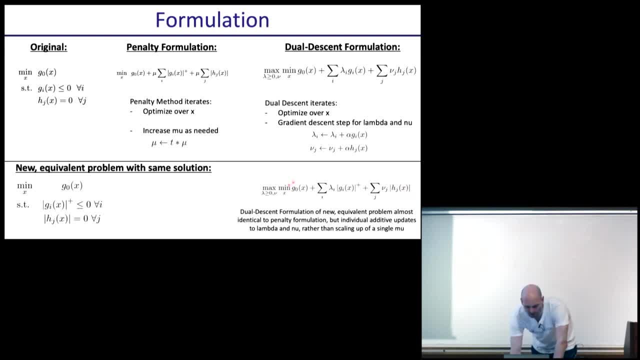 for this problem, which gives us this thing over here And now, all of a sudden, it looks a lot like a penalty formulation. If you run dual descent, we have these additive updates to each of the dual variables When we run penalty formulation. 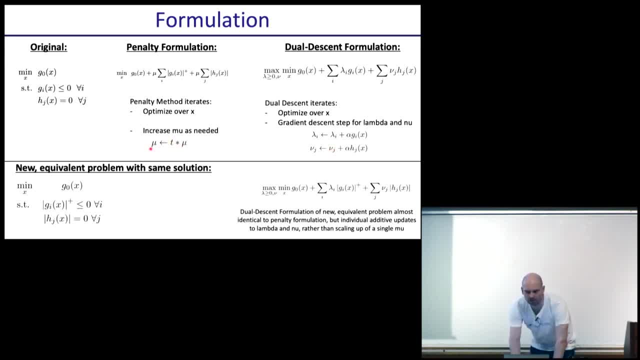 we just have a single dual variable, in some sense mu, that we just scale up periodically. Other than that, they're essentially the same at this point. So one of the places dual descent is used a lot is when you have just a very small number of constraints. 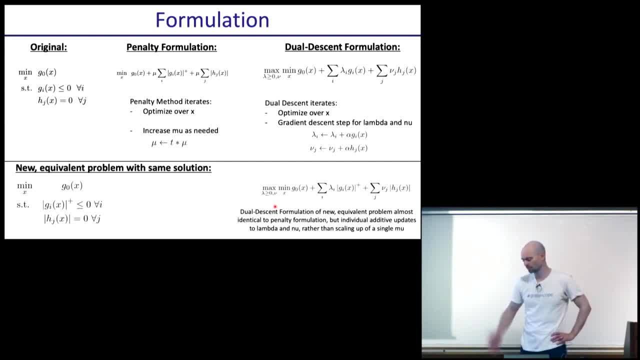 Like you might have maybe. for example, a recent place where it's used is precision policy optimizations. We'll cover a few lectures down the line. Say you want your policy to stay close to where it used to be. There's a constraint about that? 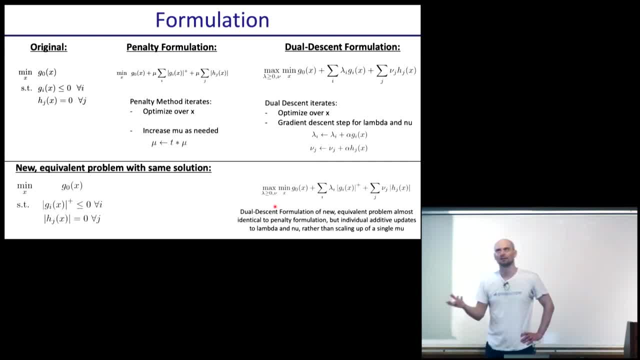 Well, if you wanna satisfy that constraint but you don't have the ability to run this kind of full optimization machinery, you just wanna run gradient descent on the original problem. this is what it allows you to do. You can keep your original problem. 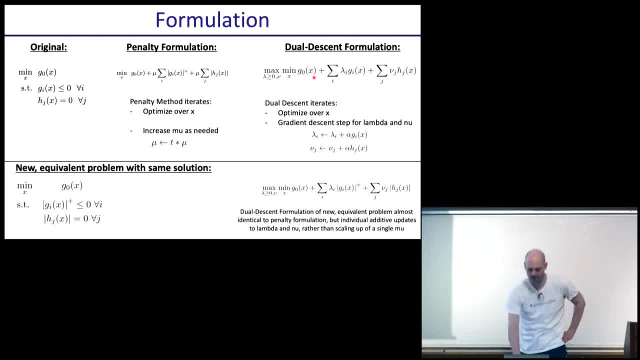 you add your constraint, just run gradient descent on your original problem And we know that if this lambda is set correctly, you're solving the correct problem anyway. And so you're just doing gradient descent on this and periodically tweak your lambda to ensure you're actually solving the problem. 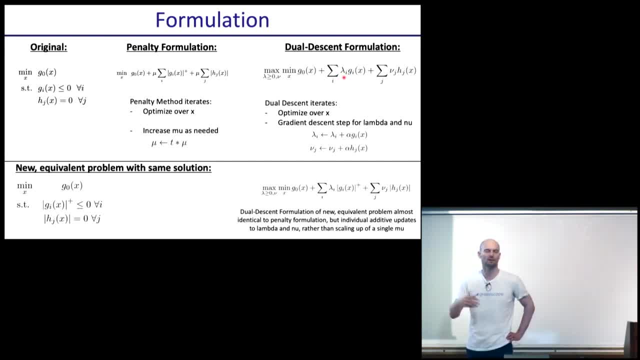 you're supposed to be solving, And so it's a way to stay close to the problem. but if you're solving the problem, that was unconstrained in everything you're doing, just periodically you need to make a slight adjustment to the objective, to tweak it. 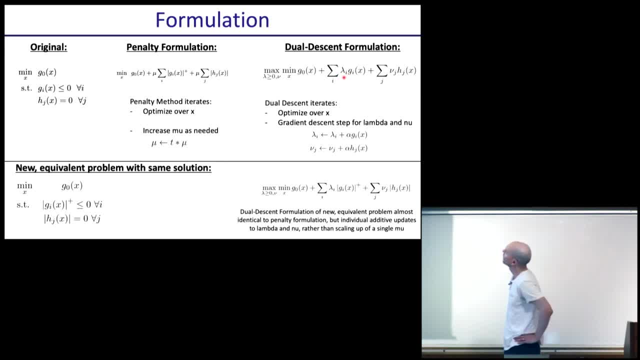 to make sure you're solving the constraint problem, And so in TRPO effectively, what it led to- and we'll see some of these things later- is that TRPO is a second-order method, effectively, which makes it hard to apply. 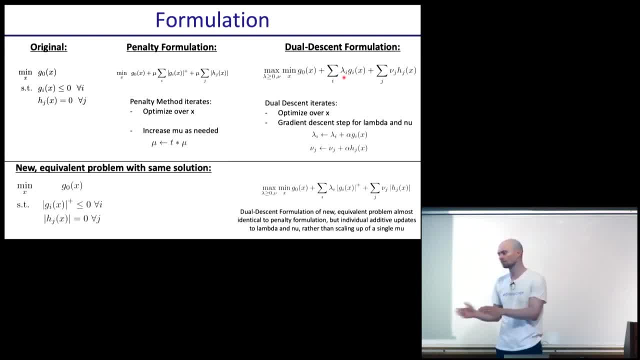 to large-scale problems at times. PPO proximal policy optimization will essentially do something close to this, where you would just adjust the Lagrange multiplier in front of the constraint and everything else can remain first-order all of a sudden and much more scalable. 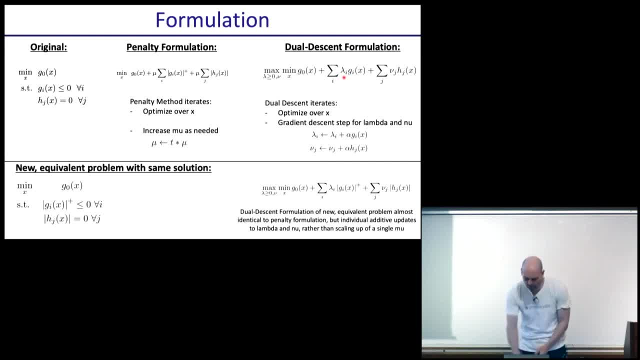 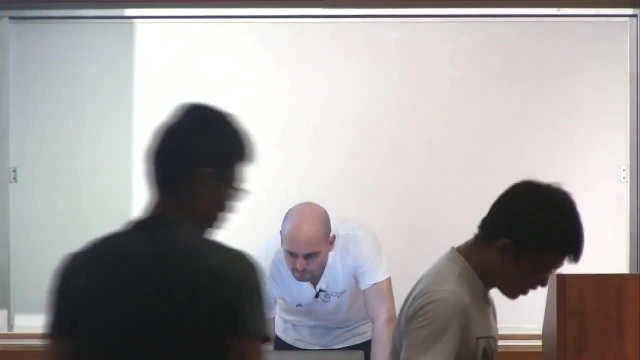 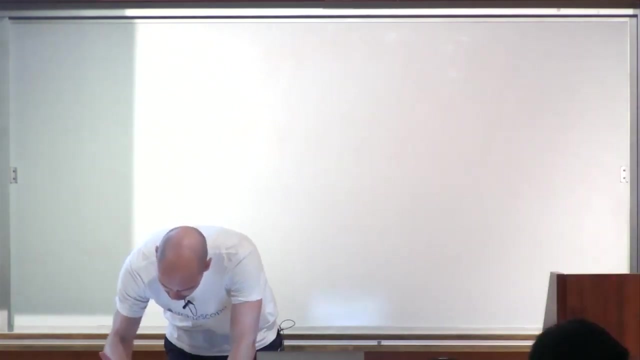 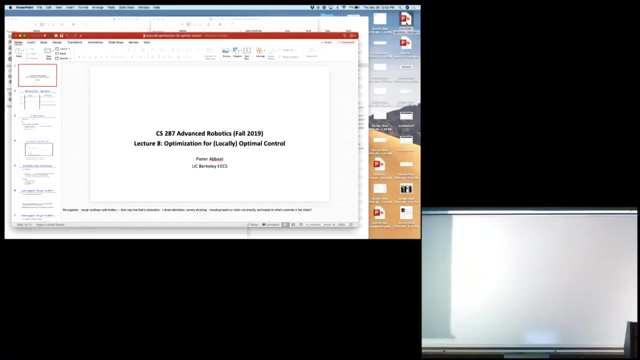 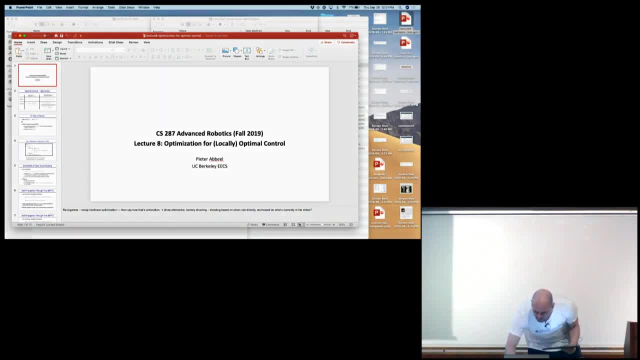 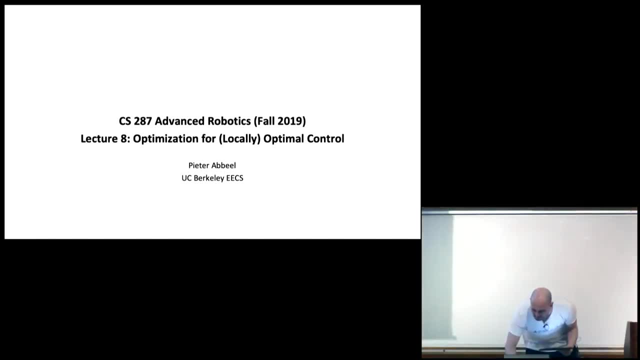 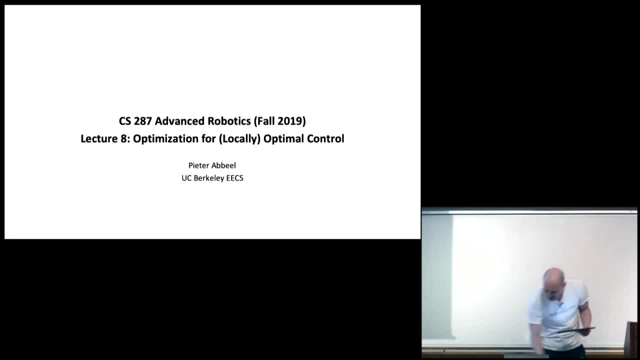 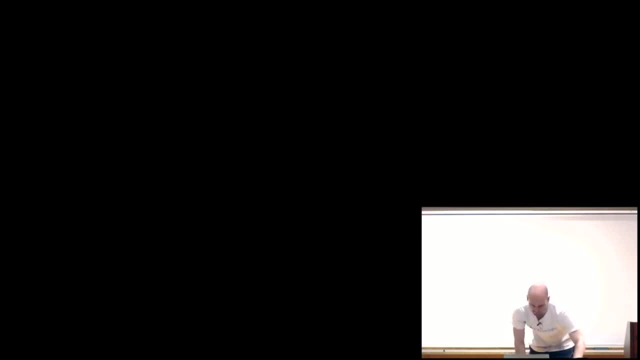 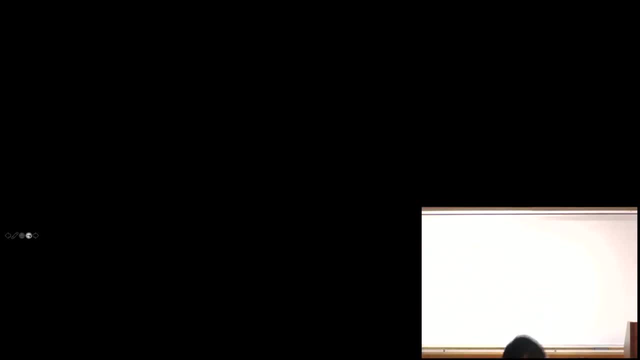 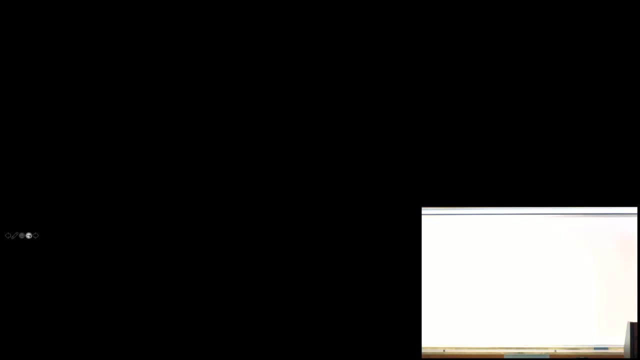 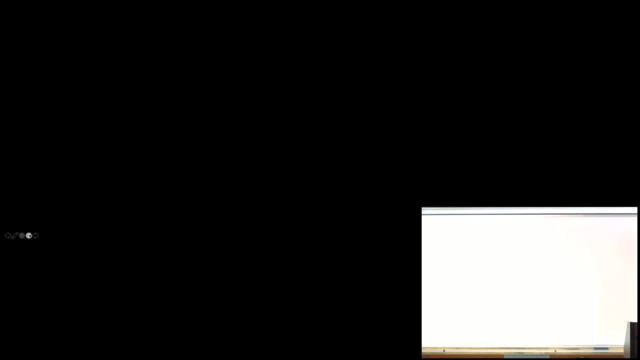 to solve, which is optimal control. It turns out there's many ways to formulate an optimal control problem and an optimization problem, So the key thing we're going to cover for the second half here is a breakdown of formulations, Because once it's formulated, 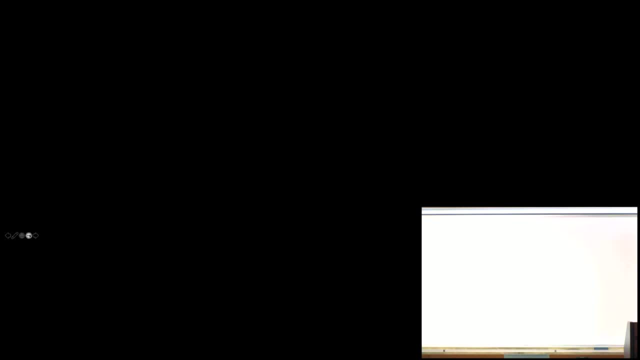 we already have solution methods. It's all about the formulation now. So there is two types of formulations in terms of the first axis is shooting and collocation. So the difference between shooting and collocation is whether, in shooting, you directly optimize over the controls. 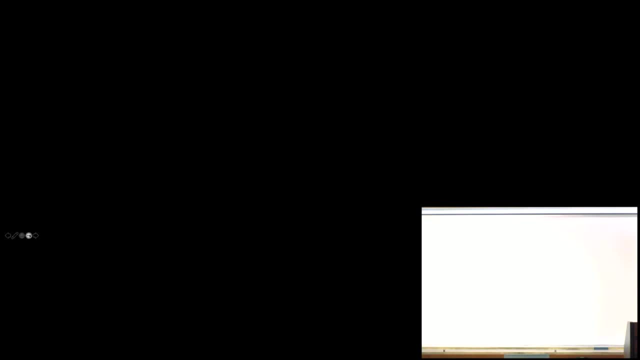 and don't really pay much attention to the state variables you encounter along the way, Whereas in collocation you optimize for both at the same time. Let me make this more concrete, And for now we'll do this: to return open loop controls. 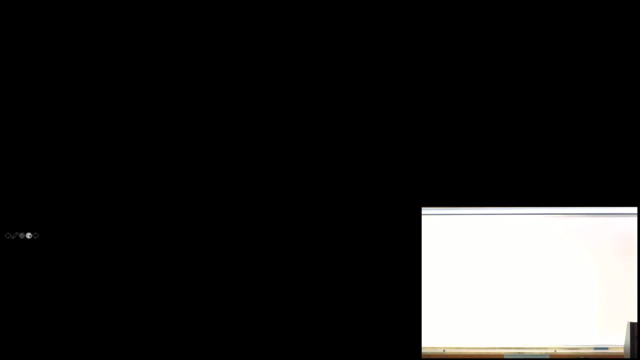 So what we'll return is the sequence of controls U zero, U one till U H, Cause that's our optimal control. from We find a sequence of control that optimizes our cost, Shooting will be minimize over U zero, U one up to U H. 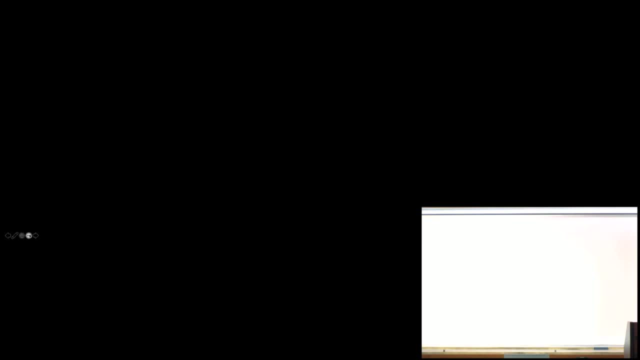 The cost for being in state X zero times zero and taking control of U zero, plus the cost for being in state X one at time one and taking action U one. But we're not having X as our optimization variables in a shooting method. So real we'll have is we'll have cost for F. 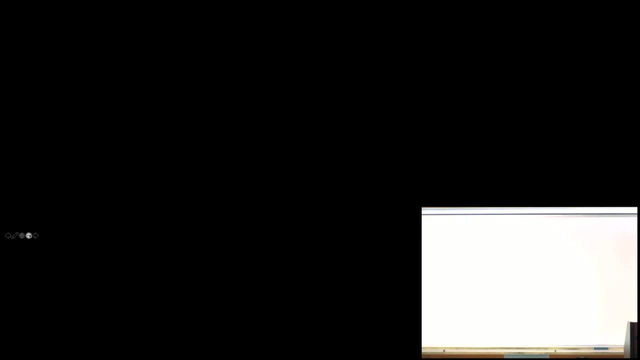 which is the dynamics of X zero, comma U zero, which is X one. but we don't put it in the optimization. We eliminate those variables: M, control U one, then plus the cost for being in state X two, taking control U two. 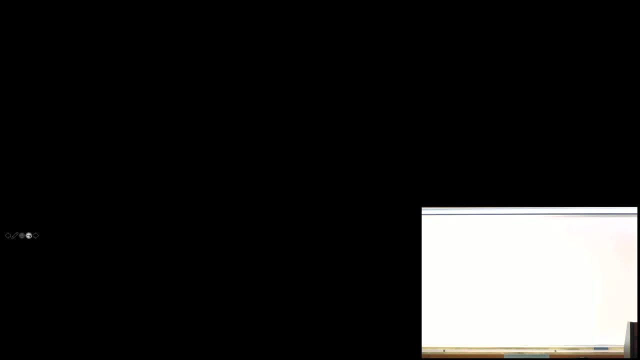 but again, we don't have an X here in the shooting method, We have only U variables. So it'll be F of F of X, zero, U, zero, U, one, U, two and so forth. That's a shooting approach, The collocation approach and we'll talk about based on. 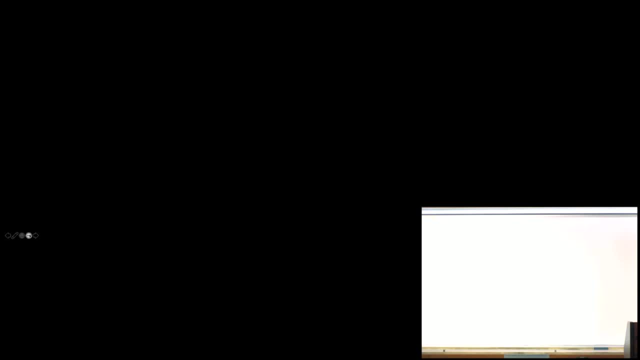 will be exactly what I'm gonna talk about next: benefits and downsides. in a moment. collocation approach would say: you know what? I'm just gonna keep the x variables around. So I'm just gonna say: minimize over u zero x, zero. 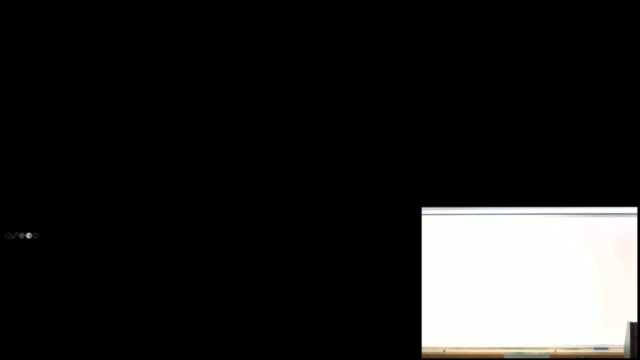 I should phrase it the other way: x zero, u zero, x one u one, all the way till x, h u h. The sum t equals zero for h of the cost of x t u t. subject to x, t plus one equals f of x t comma u t. 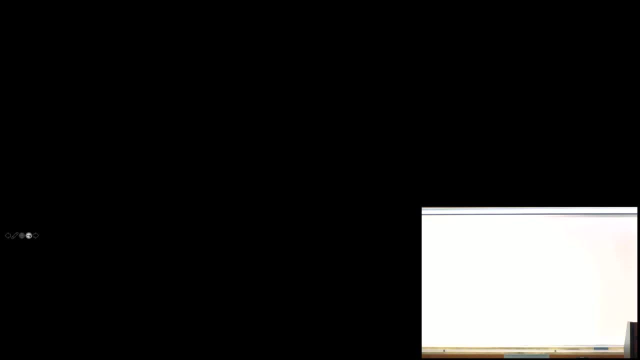 Because x's cannot be arbitrarily chosen. we have to choose them to satisfy the constraint. There could be other constraints, like u's have to line up some boundaries and so forth, but let's not worry about writing those up, So let's think about first. 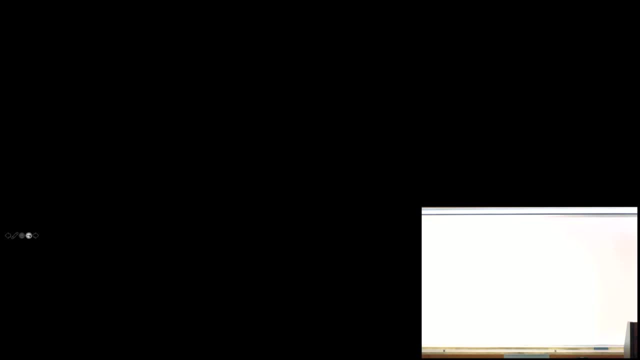 if we solve this problem or this problem, the optimal solution is gonna be the same thing. It's gonna be the same sequence of controls. There's no difference, And we have optimization methods at our disposal, so why would you even care about different formulations? 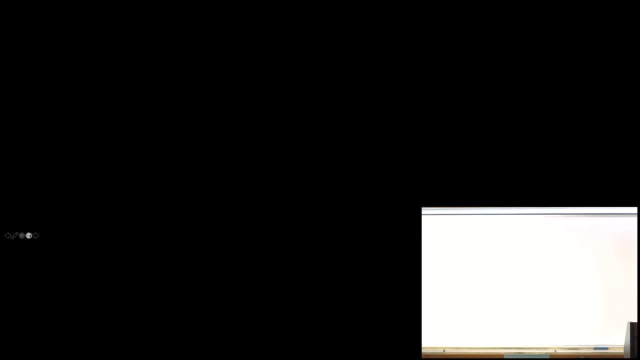 one versus the other. Well, think back about these optimization methods. When they work well don't work well. People have an issue with. optimization methods is when they're poorly conditioned. Some variables have much more influence on other variables in complicated ways, and so forth. 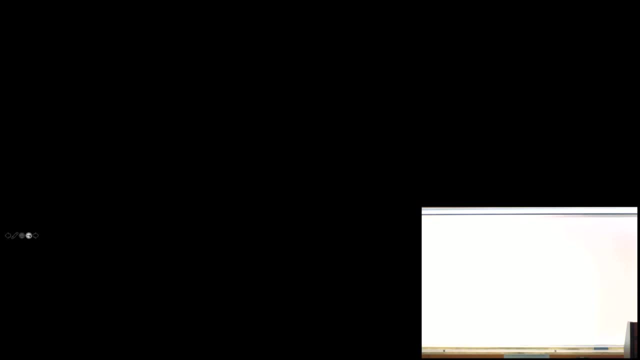 Well, that's gonna happen here. It's gonna happen very directly, because u zero is coming in everywhere and u zero has an effect on what the final state is going to be. Imagine you're controlling a car and u zero is saying how much you steered. 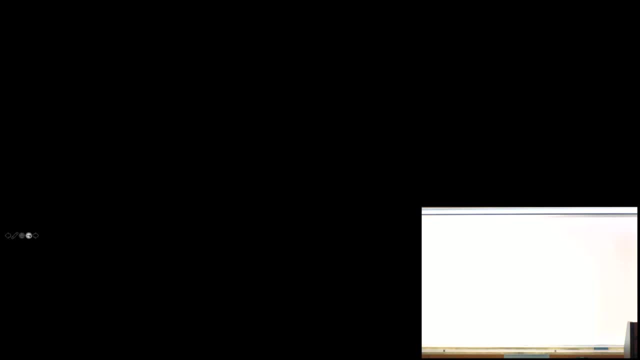 to the left or right in the very beginning. Well, that'll have tremendous influence on where you end up at the end. If you steered 90 degrees to the left in the beginning, it'd have a completely different place than if you did not do that. 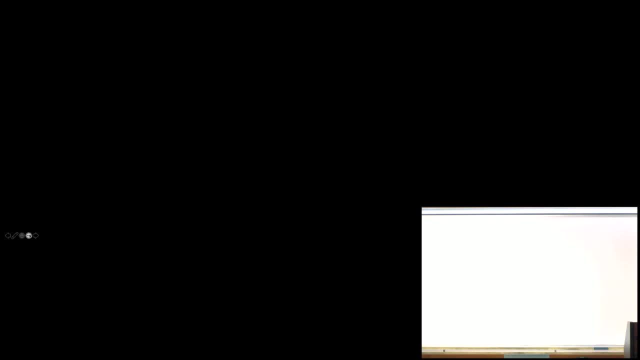 And so shooting methods in general are gonna be poorly conditioned pretty much by design. Hence difficult optimization problems to solve Doesn't mean they're not solvable. I mean we have second-order methods you can deal with at times, but it's typically gonna be harder to solve. 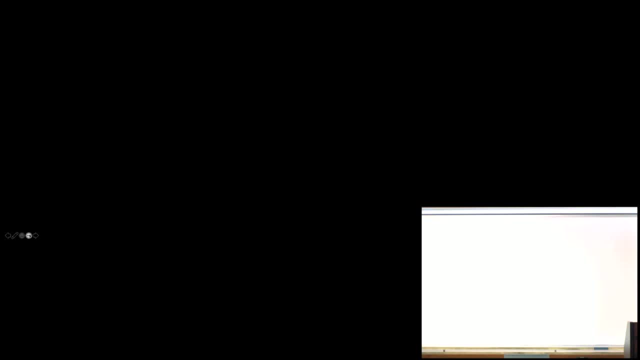 What's the upside? Well, if your state space is very high-dimensional, imagine you work- I don't know- in image space You have a f function that goes from image to next image to next image. Well then your x variables will be used. 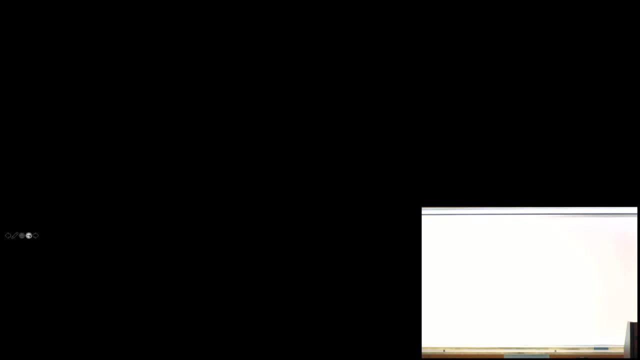 there'll be one megapixel images of a million variables at every time, Then well, if you have to keep them around explicitly, then maybe it's harder to deal with. So the dimensionality of x might affect whether you can afford a collocation method or not. 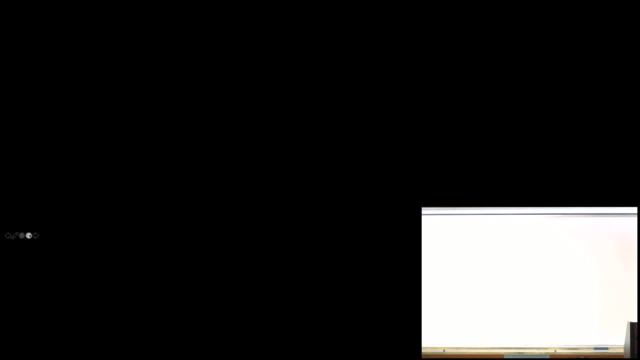 especially when u is low-dimensional, it might be convenient to keep the problem as a whole low-dimensional. that you optimize over The collocation method nicely decouples. What's the effect of u zero? Well, the effect of u zero doesn't propagate anywhere. 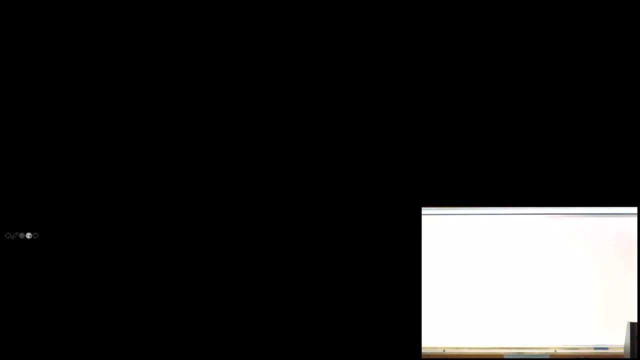 into the future. If you use constrained optimization, the way we've seen it, well, all that'll happen- let's say you use a penalty method- is that, if you look at the terms that appear in the penalty method, is that u, zero just appears? 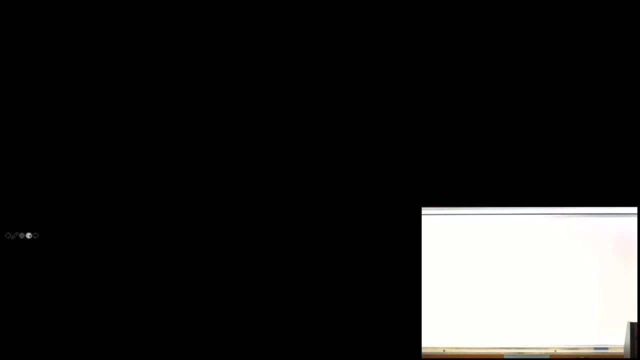 in the very first constraint, and that's it. It does not have any effect on anything that happens later, And so the x variables decouple the optimization problem, typically make it a lot better condition than if you do this kind of propagation through time. 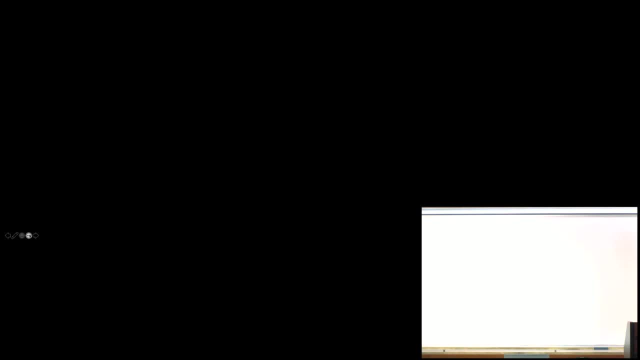 of all the controls and effects they have in the future. Now, this, in both cases, is solving for u's. You can actually do the same thing: solving for feedback policies. Let's say we want to return pi theta a feedback policy. 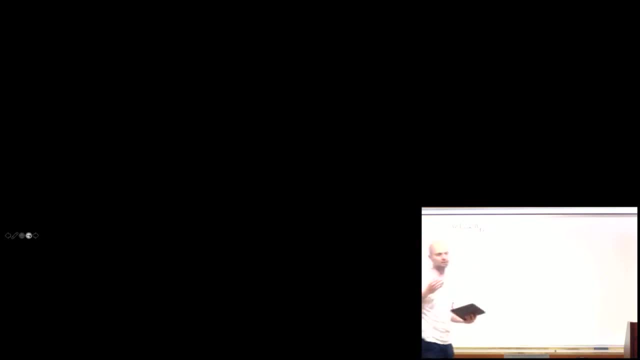 maybe linear feedback controller, k times x or k times x plus some offset k, or maybe a neural network pi theta. you want to find a parameter's theta. we can do the exact same thing And we can again do shooting or collocation on both cases. 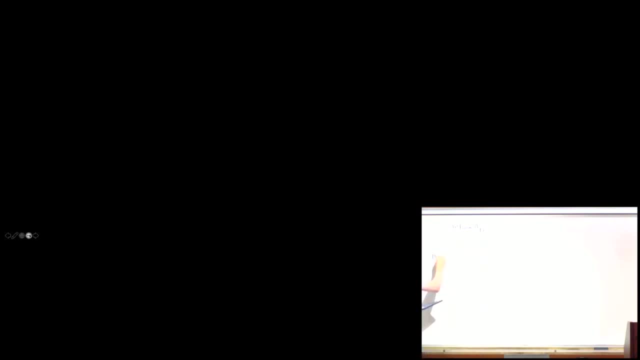 This can be done. so shooting would be min over theta, because now theta's the only thing we optimize over cost for x zero and taking action: u zero, at time zero. but u zero is not a variable right now, it's just pi theta of x zero plus. 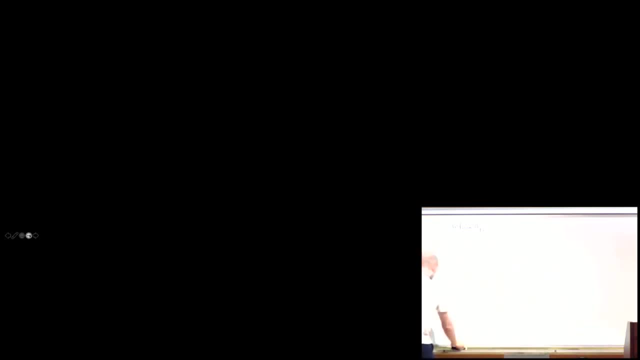 actually I'm gonna move this up to have a little more space. So min over theta c of x zero, pi theta x zero, plus same thing as over here, except that we replace the u one with pi theta of x one. 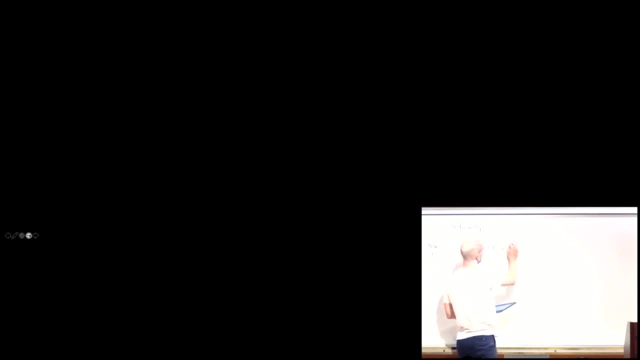 and we replace u zero by pi theta of x zero, so f of x zero comma, pi theta of x zero comma pi theta of x one plus another cost and so forth. Here I wrote three terms out of the many, many terms. Here I only wrote two. 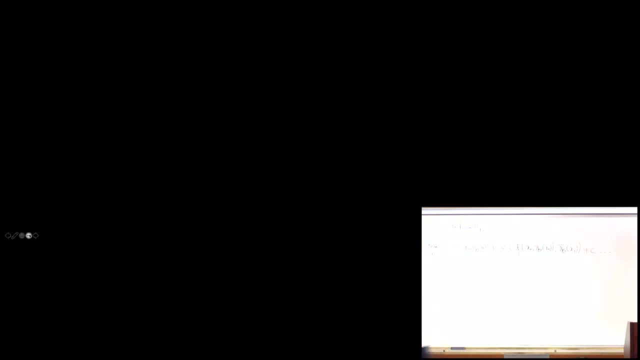 And we can do collocation. Now, actually, there's two ways to do collocation, So let me give you both. One way to do it is to say: I'm gonna do it exactly with this set of numbers, With this set of equations. 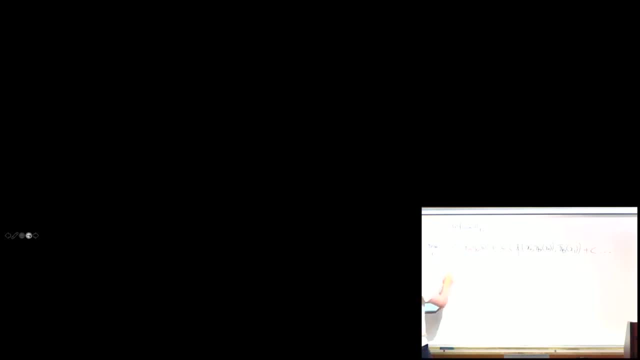 So I'm just gonna say: minimize over the axis zero through h and theta, sum of the costs, cost at each time for state at that time and control applied at that time. subject to x, t plus one, equals f of x t, comma, pi, theta of x t. 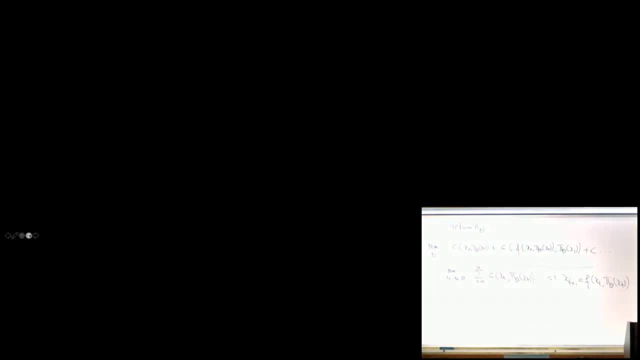 You can do it differently. You can say: why don't we collocate even more? That's fine too. You can say: why not just keep the u variables around, also Because maybe this pi theta is kind of constraining you. 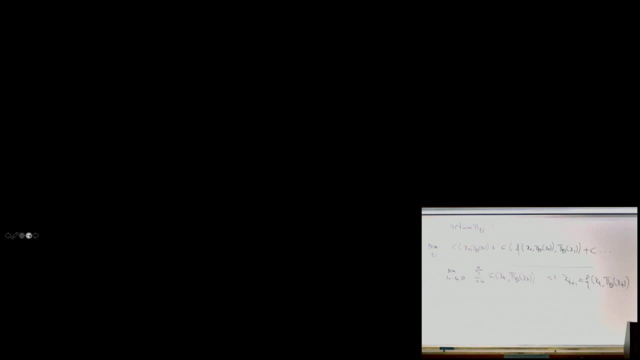 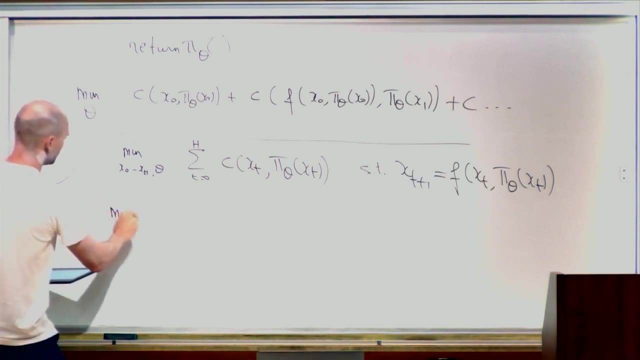 The function form of pi theta doesn't give you the flexibility you want and you wanna make your u something else. You wanna kinda make your optimization a little easier. when you start out You can say, well, minimize over x, t, x, zero through x h. 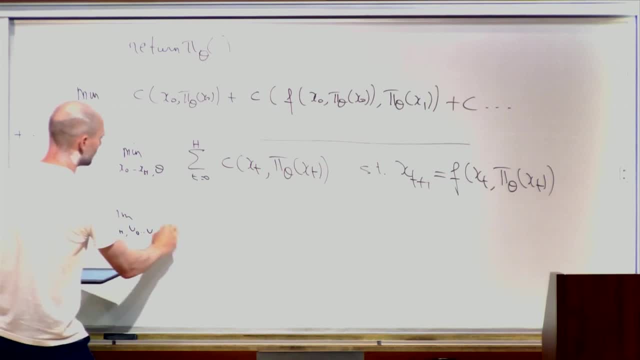 u zero through u h, m theta. same thing: t equals zero to h. but now the cost is in terms of x t and u t, and then the constraints are: x t plus one equals f of x t comma u t. 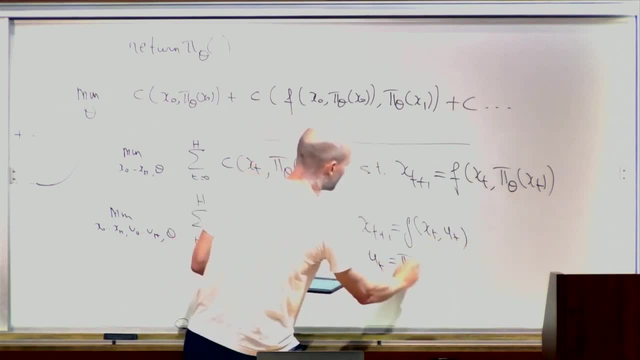 and u t has to be pi theta of x t. And so in this optimization, when you run it this way at times your controls that you optimize over your u t's will not satisfy this. Your penalty method will only at the end get dissatisfied. 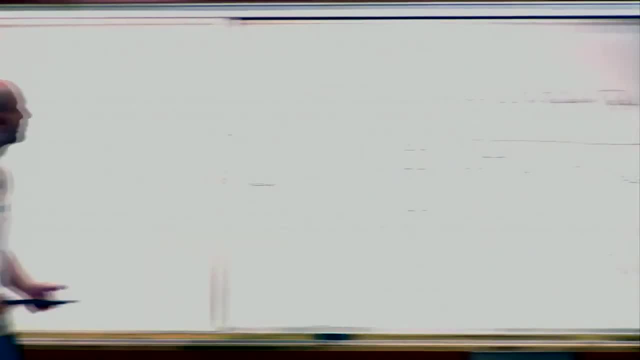 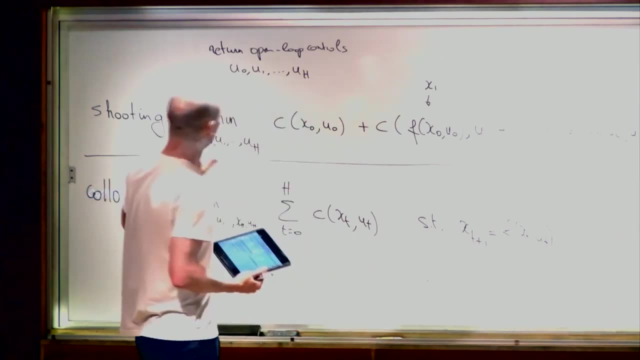 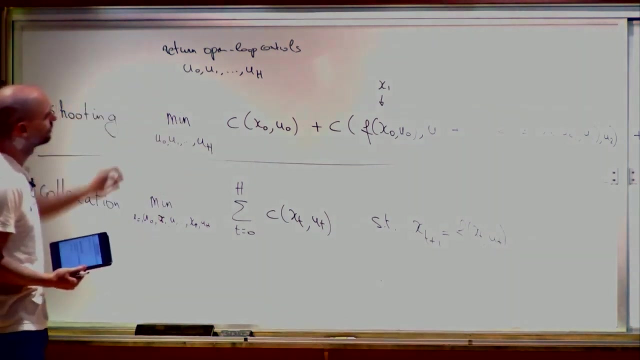 but it might give you more freedom in terms of initially finding what sequence of controls could be good. So these are four different formulations, and all are solving this. Well, that one's solving for feedback policies and this one is solving for open loop. 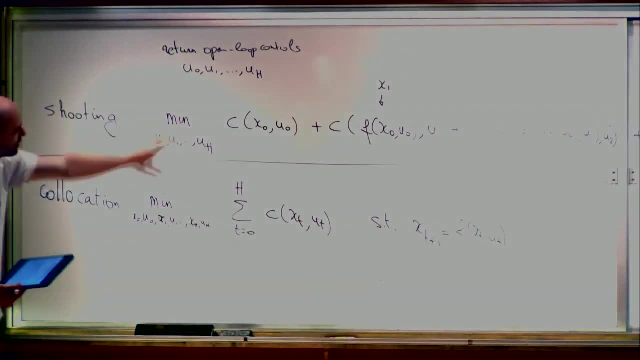 but ultimately, all three on the line on the right and solve the same problem. All two on the left solve the same problem. The difference is in condition and size of the variables that you're dealing with when you're running this. There's a third axis of choice. 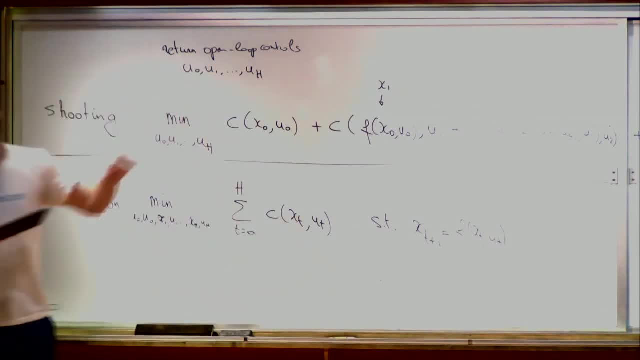 You might say: well, open loop controls seem a little fragile, Like I find open loop control and then I start executing, but a little bit of noise in the system and it will not be valid anymore. Well, what you can do on top of this. 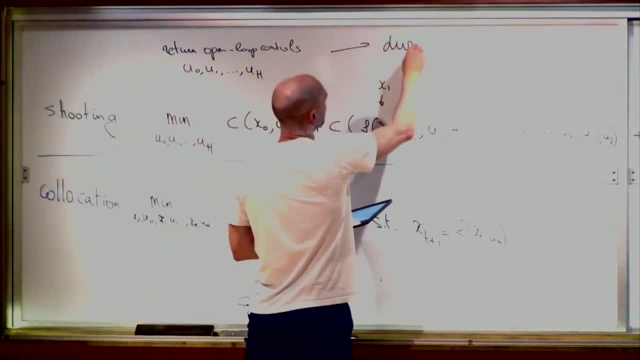 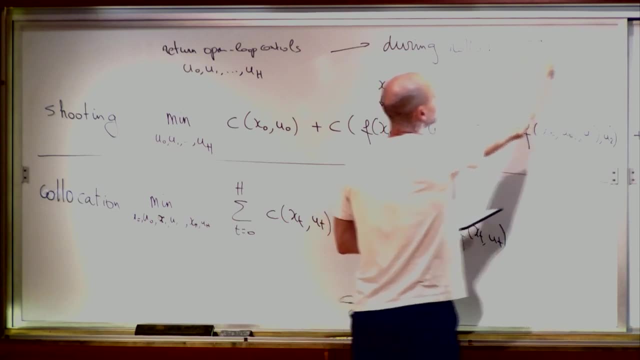 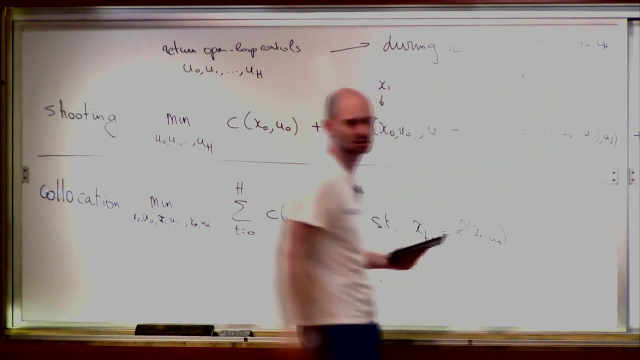 you can then during rollout just use u0 through- uh, that's naive thing. or you can do something called model predictive control, MPC. Let me spell it out: model predictive control- What does that mean? It means that after you took your first step, 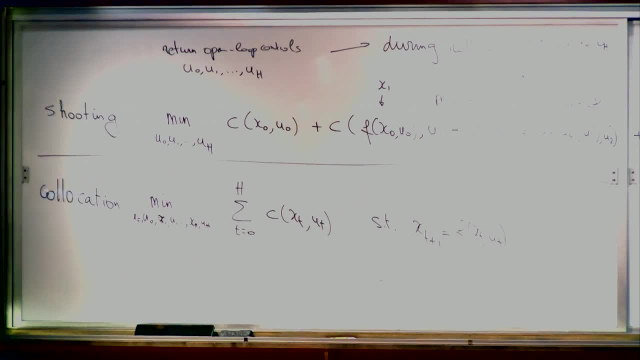 you just solve the optimization problem again from time one and then take another step and solve it again, again, again, And so that's the way to. even though you solve for open loop controls, you're still applying a feedback policies. After every step, you check what happened. 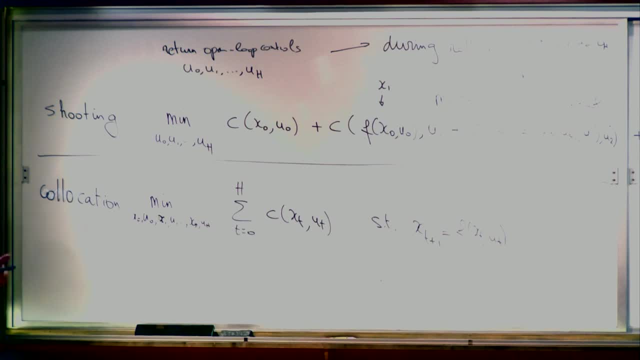 and find the outcome relative to where you landed. and that's exactly what it means to do: feedback control. It's just that it's not even in a parametric form. It's by you having to resolve every time. Now you can also do that here. 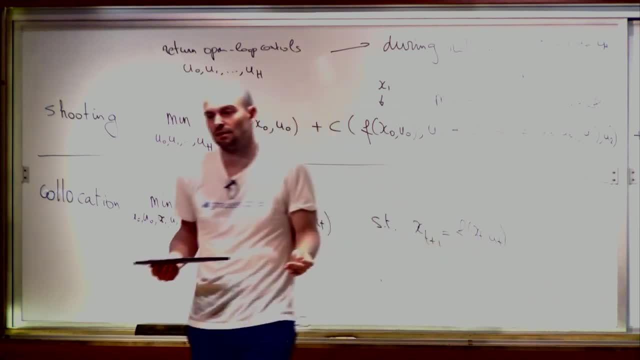 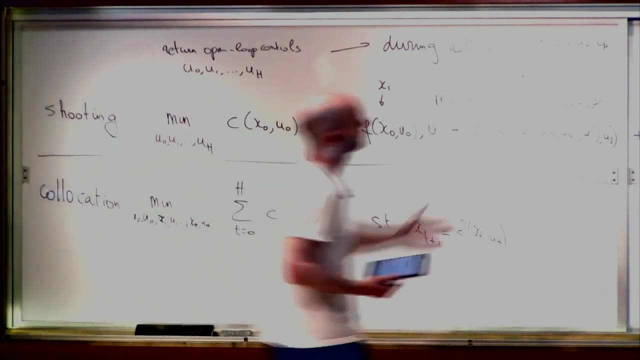 It could be that your pi theta is somewhat restrictive, that you feel like, okay, it's not as fine tuned to the situation as I want it to be, It's just more of a starting point and you can actually take a first step and resolve for the best pi theta. 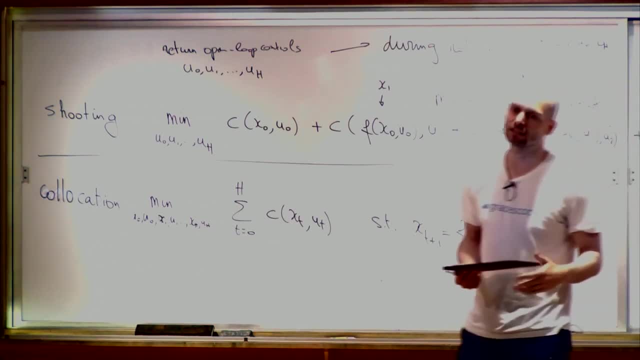 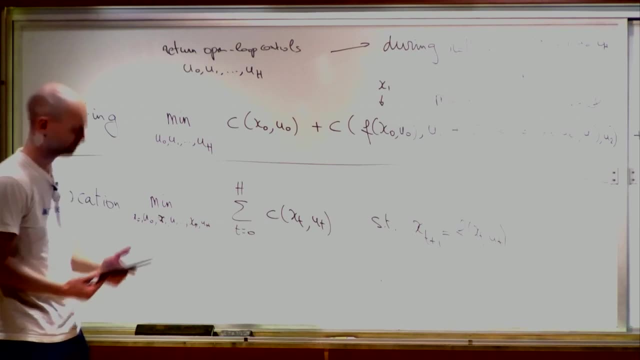 for the horizon that remains, and repeat, repeat, repeat. That's not done very often, In fact I would say it's rarely done, but in principle it's an option you have available to you if you wanna do it Now. what are some issues of this thing over here? 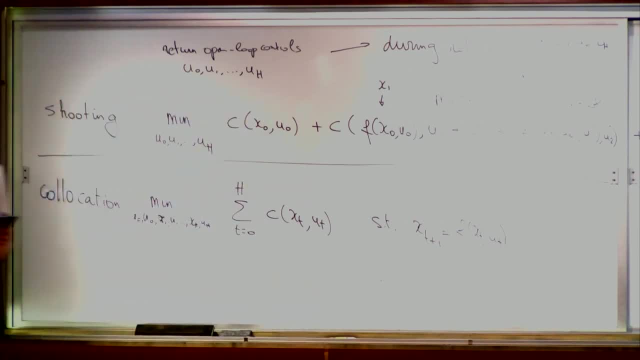 This thing when you are optimizing for these? u's, what really happens? Well, two things will happen. One is if you look at your derivatives, u zero appears in so many places. You see a lot of shared computation. If you wanna do something more efficient. 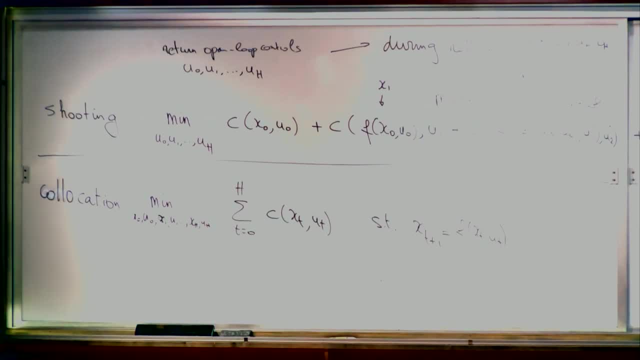 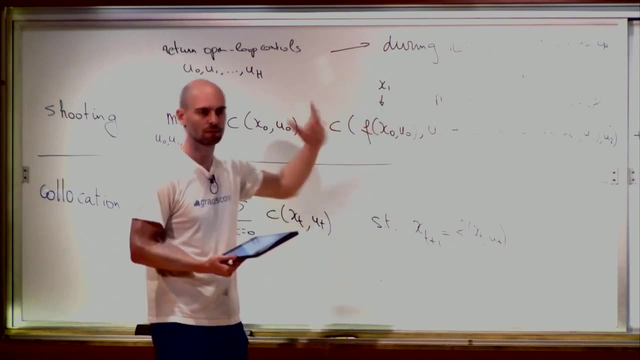 that could read every derivative independently. well, there's something called back-replication At the time I'll have a slide illustrating that, but the idea is that you'll do shared calculations, so anything that reappears as a component that you need to find derivatives. 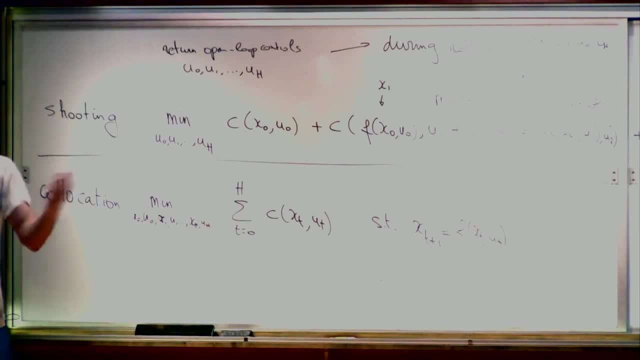 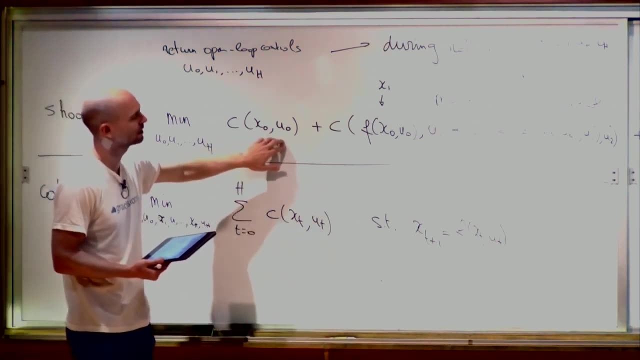 with respect to the? u entries, you'll do in a shared way, dynamic programming way to minimize computation cost. So that's one thing that you need to do here, Otherwise it gets super expensive very quickly. but if you set it up in some more intensive flow, 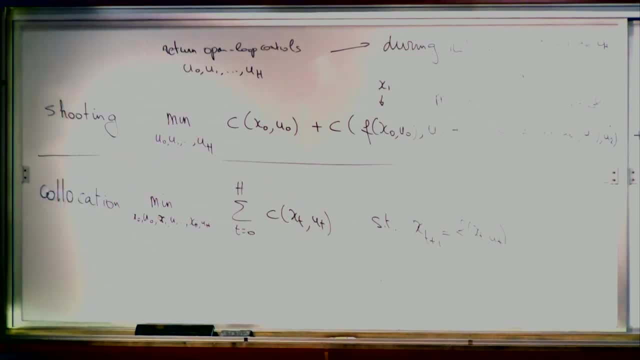 or any kind of automatic precision package. it'll automatically do that dynamic programming for you and it'll be very easy. But it is something that's important, Otherwise it won't work. At least computation will be too expensive. There's another thing that's tricky. 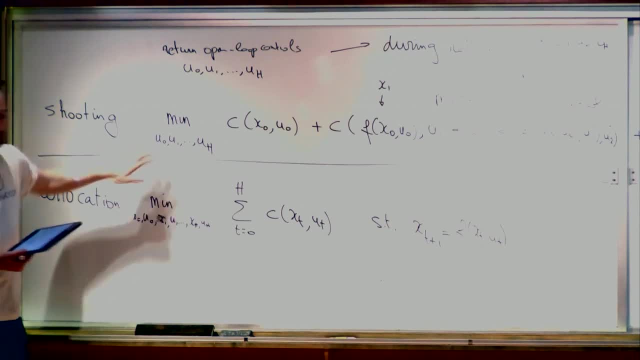 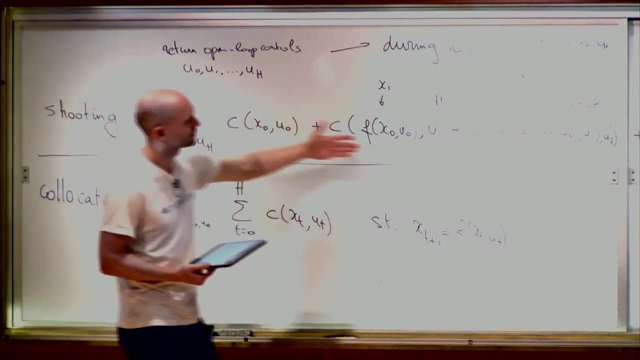 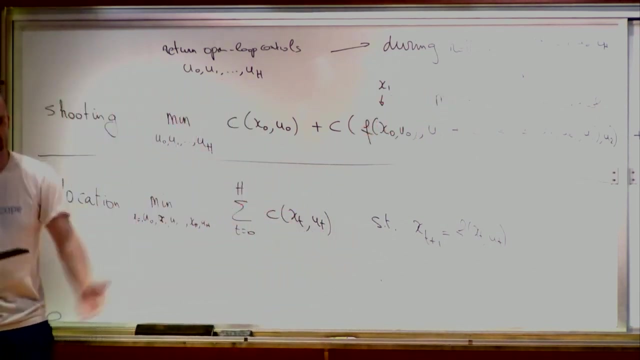 is that you find your current controls, as will happen in optimization. What will happen next? You'll essentially have to roll this out over time, do a back-replication backwards to find the derivatives, and then you can do your optimization step. 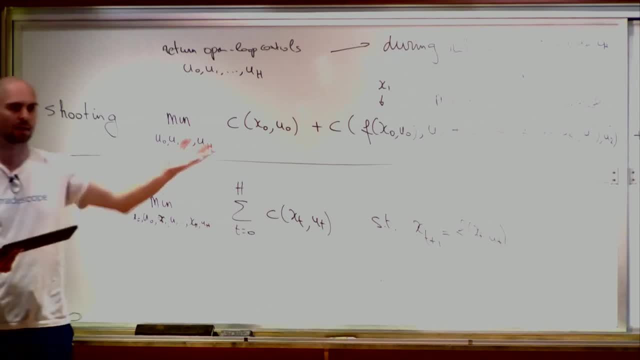 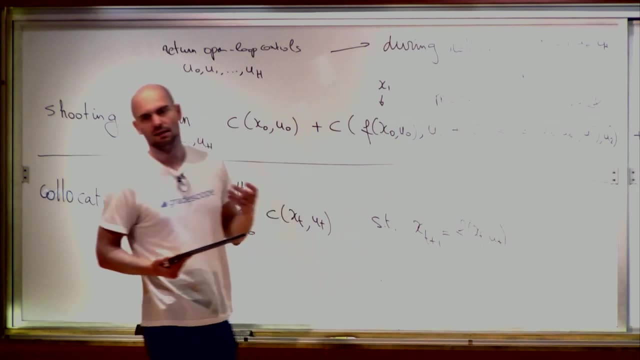 Or maybe Newton's step. you need also Hessian's. but it's a gradient method. just a back-replication down. you get your gradient, do an update. Tricky thing is that even during this rollout there could be even if there's no actual noise in the system. 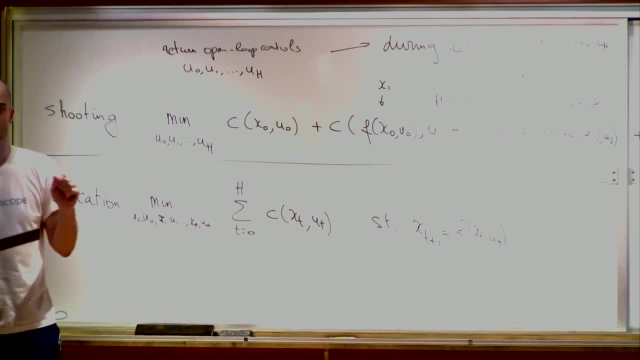 it could be numerical instabilities leading to small things going differently. and ultimately what happens? because this is all nonlinear functions, you get instability in your rollout, And so even your optimization actually doesn't work. What's the fix to that? The fix to that is to then. 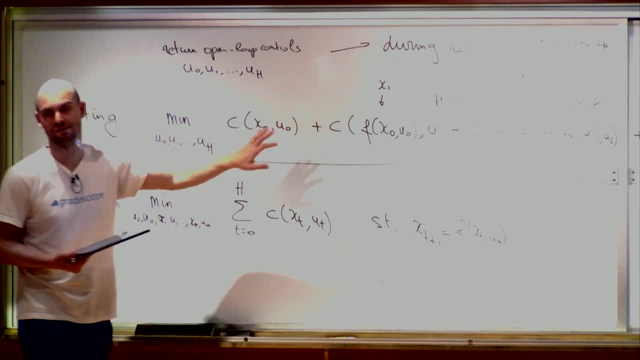 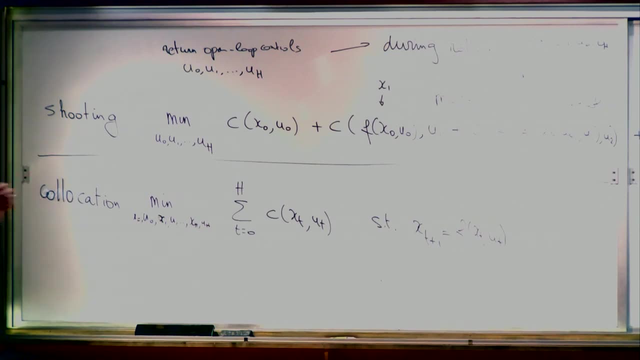 run MPC in the inner loop of your optimization. So this becomes very intense. but you would say I have a current U To roll it out because I want to find gradients. to find gradients I need to roll out and do a back-replication. 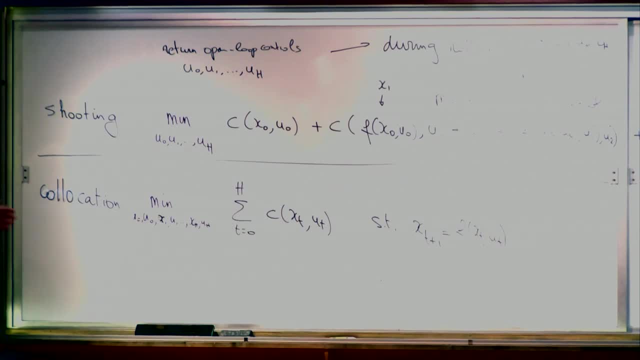 To roll it out. I can't just roll out the U that I currently have. I have to do MPC as I roll out. Once I've done that, I have a good rollout, then I can do back-replication through that rollout. 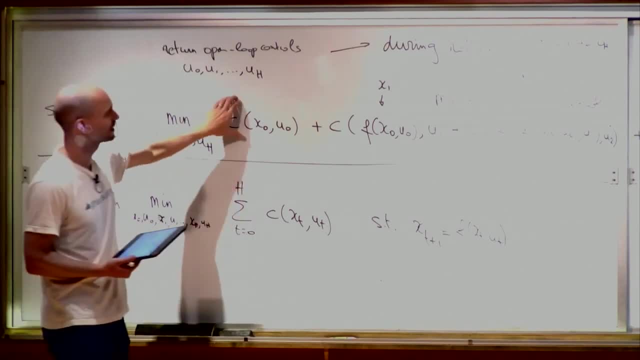 do an update and repeat, And so that's one way to make this stable, and without it, often it's just not gonna work. And so that's one way to make this stable, and without it often it's just not gonna work. 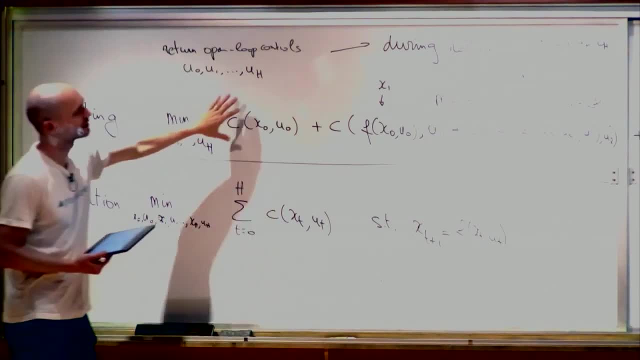 And so that's one way to make this stable, and without it often it's just not gonna work. If you have an unstable dynamical system, this formulation will not work unless you do something to take care of stabilization in the forward path. 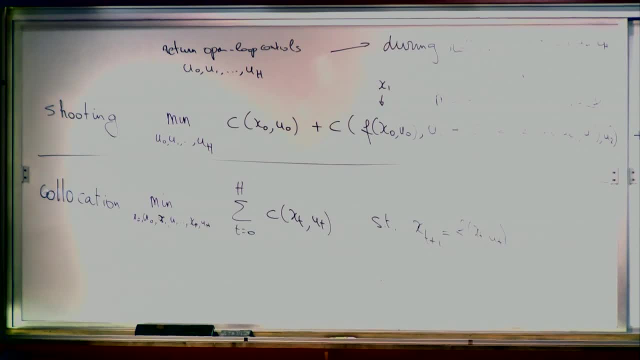 Let's see, Let's do a roundup of what's different between the different methods Shooting. you improve the control sequence over time. I said a lot of not-so-great things about it making it difficult, but actually one great thing about this or this. 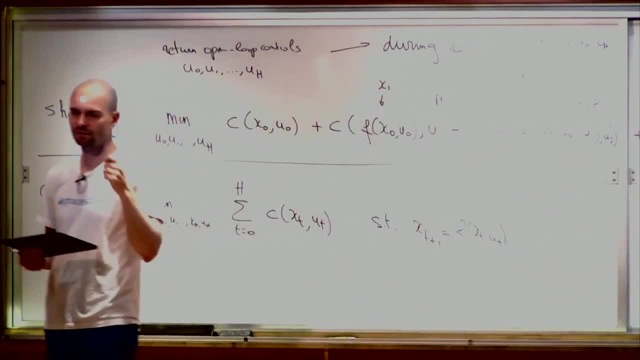 is that at all times you're feasible. As you're optimizing, you have a feasible solution, something you can actually use. You could use that sequence of controls or you could use that feedback policy you found so far, When you're in the bottom category, the collocation method. 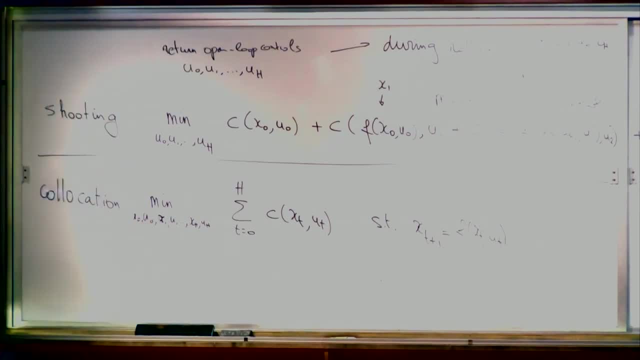 it might be that some of your controls are infeasible, are incompatible with things that you need to satisfy in your constraint set, and so you actually don't know how well you're doing. Like when you're running the bottom one, you'll have a score. 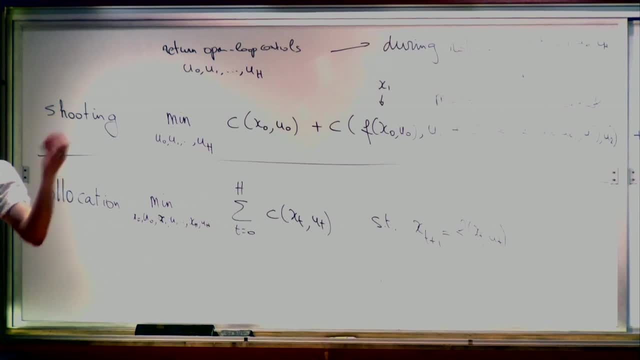 but that score will be a combination of cost as well as penalty from violating constraints. And well, if you violate the constraints, it's just a penalty in your optimization, but in the real world you don't know what's gonna happen. 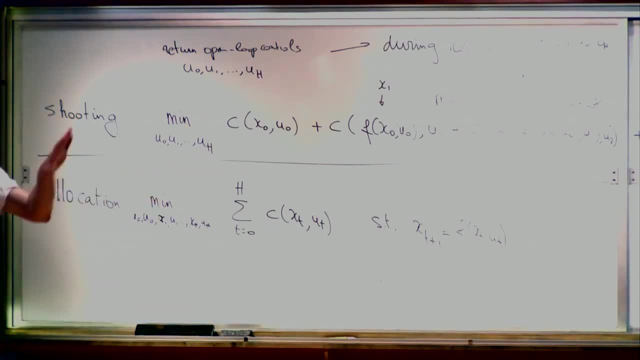 If you violate your dynamics somewhere, you say, well, yeah, in this step I'm just gonna violate the dynamics, it's fine and it's a small, it's just a penalty. But that penalty is not actually quantifying what's gonna happen when you take that control. 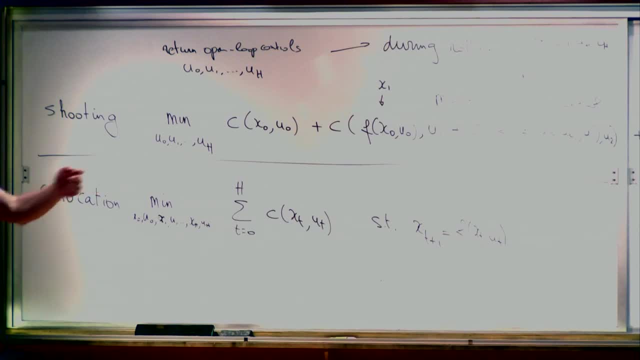 and propagate it forward in time And how this rollout's gonna play out. So you'll have no real notion of how well your current thing is doing. Only once all penalties have gone to zero will you know. oh, it's feasible and I'm gonna do exactly what's written down now. 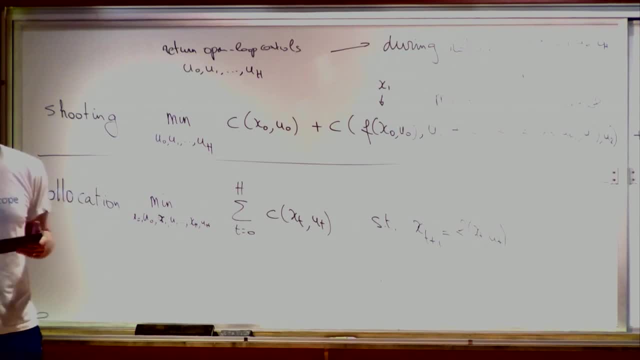 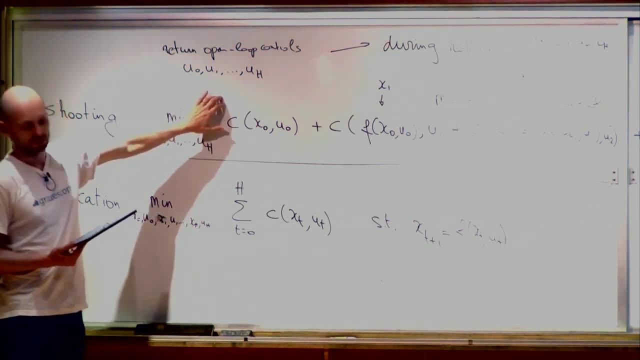 in the u's and the x's, But before that things could go completely differently and you wouldn't know it. This one, as I mentioned, is often very poorly conditioned and that's a bit of a downside of using that method. 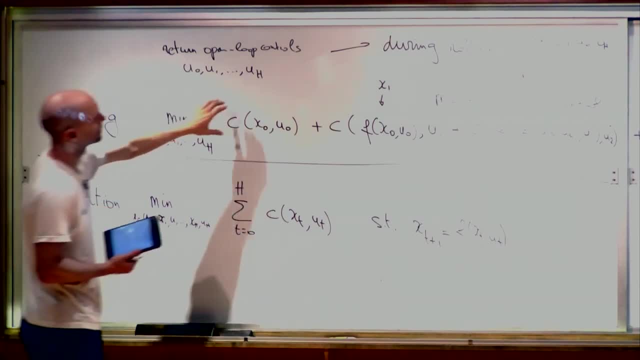 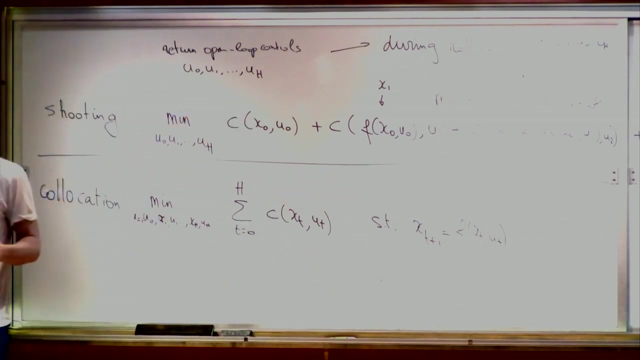 You really need to be very careful when you optimize this objective to deal with the poor conditioning because of different u's having such different influence on what happens. Another downside of this one is that, both this one and the one over there, it's not so clear how to initialize. 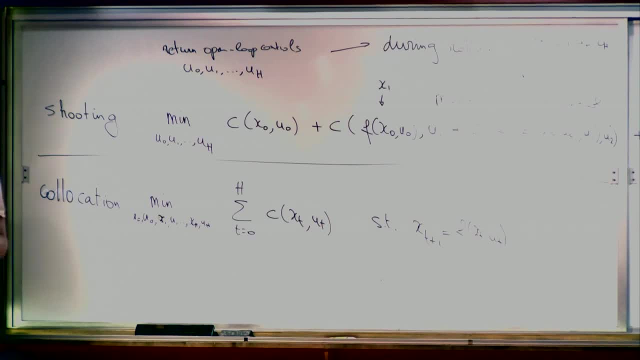 Imagine you want a car to go from point A to point B. Well, what are the exact controls you need to apply? Maybe you can try to think where it's very hard, But that's all you get. to initialize here is the u's or some policy. 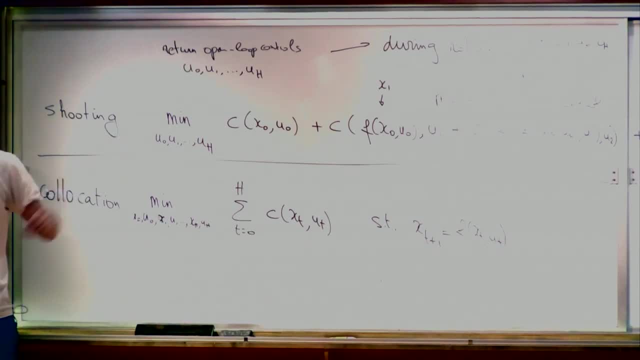 Here you get to initialize the x's. If I want my car to go from point A to point B and it's an empty space, I can just draw a straight line and say, well, probably the car cannot follow that straight line. 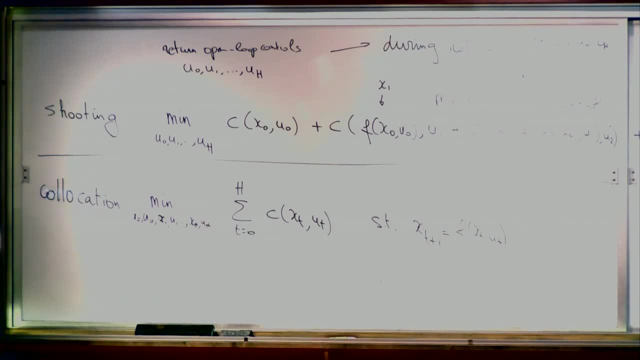 but it might be able to follow something relatively close to that and that might be a pretty decent initialization for the solution I'm trying to find. And so, because you have access to initialization of the x's, you have any intuition of what the solution would look like. 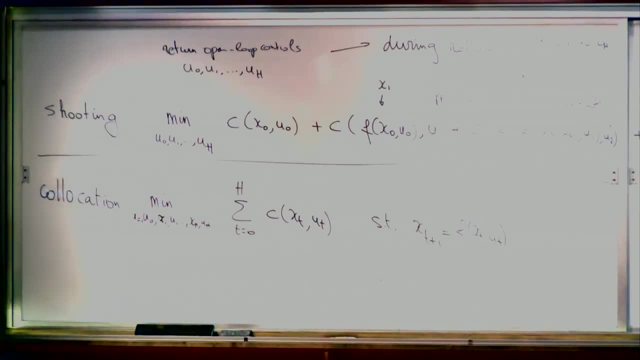 you can actually put it in an initialization and often solve a problem that maybe we don't know. but you can actually put it in an initialization and often solve a problem that maybe we don't know, maybe with a shooting method. 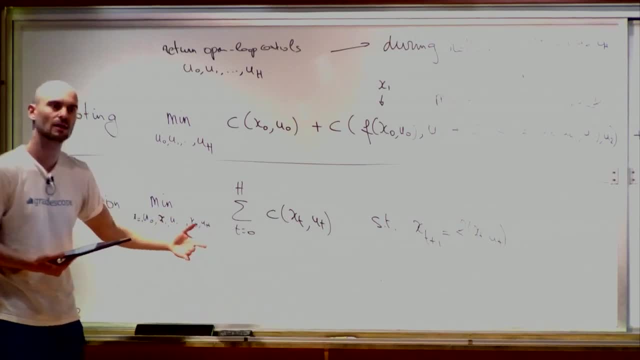 because an elderly nonlinear problem might never find a solution. but here you have a lot of influence on how you set up the problem when you start out, so you might have enough information to find a solution. Another upside of this one is it makes the commutation stable. 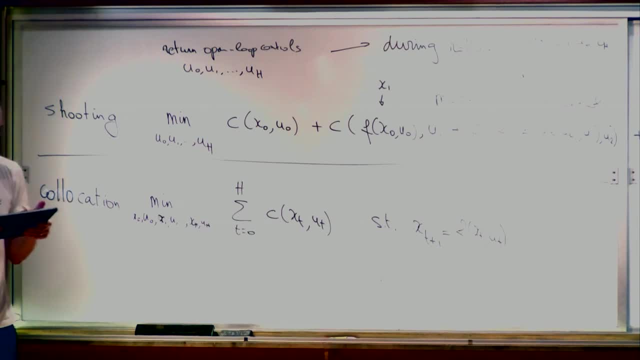 by having a decoupling through the x's. The main downside of this one here is that it might converge to a local optimum of the surrogate function, and that is not actually feasible. So you might end up with non-zero penalties and there's no way to improve. 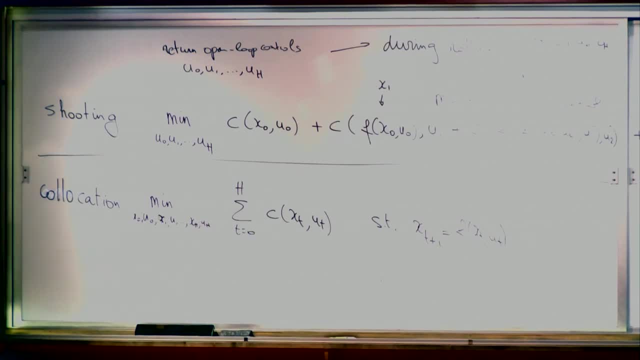 and that's where you're at, and you just now don't know what to do. You could try those sequence of controls and see what happens, but you actually don't know, based on just the objective, that that's gonna be any good. 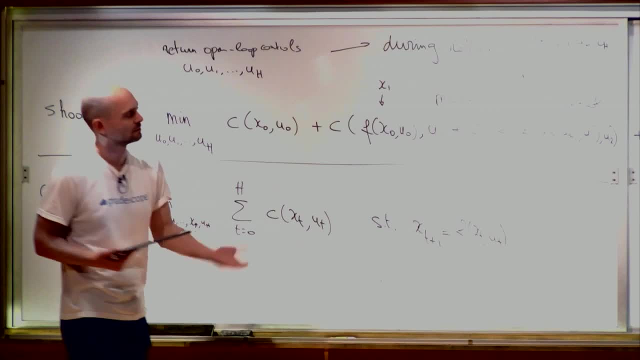 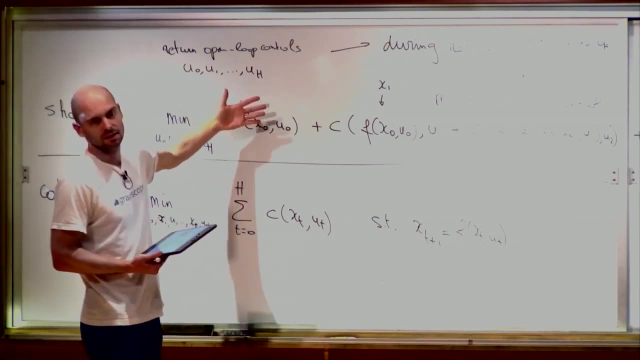 And so you might get stuck in kind of a weird local optimum where you don't have any way to get out and maybe you need to reinitialize and try again, Whereas here, if you are in a local optimum, you still know what is going to happen. 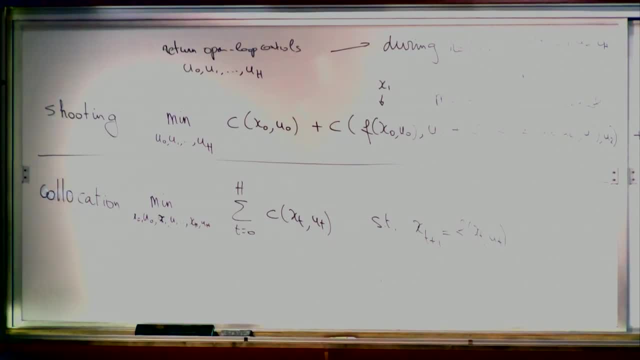 because you know what the rollout is giving you. Now, of course, in this one, once you're in such a local optimum, you can do a rollout and see what happens, but it doesn't, I think, give you anything to improve. 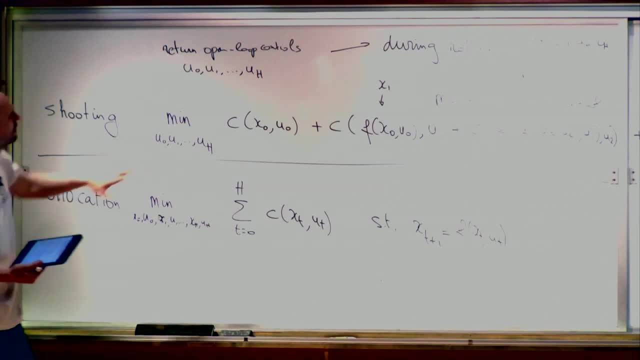 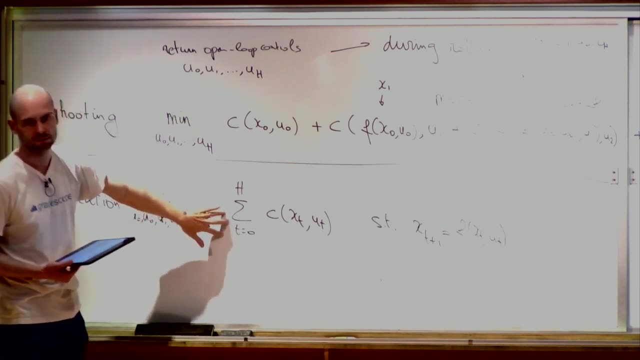 So another thing to point out is that the NPC, while probably most critical- if you use this formulation, you can also use it here just as well- right In the collocation method, you apply your first control, you re-solve, repeat it. 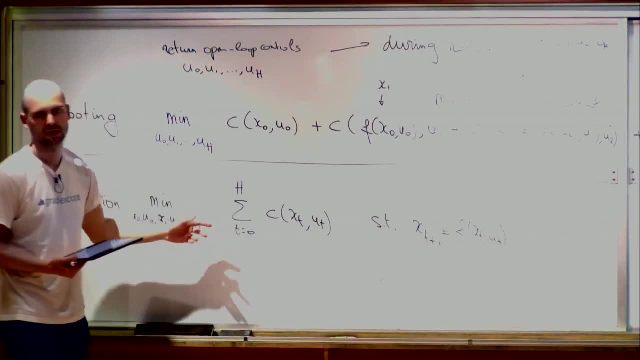 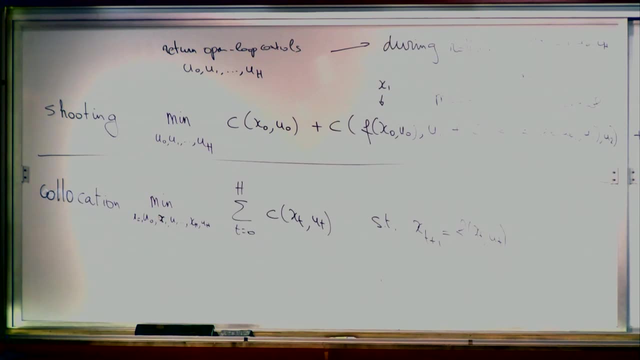 In fact you often have to, because if there's noise in the execution again the original sequence of controls will not be good. Question you might have is: how about iterative LQR? That's another method we saw to solve these kinds of problems. 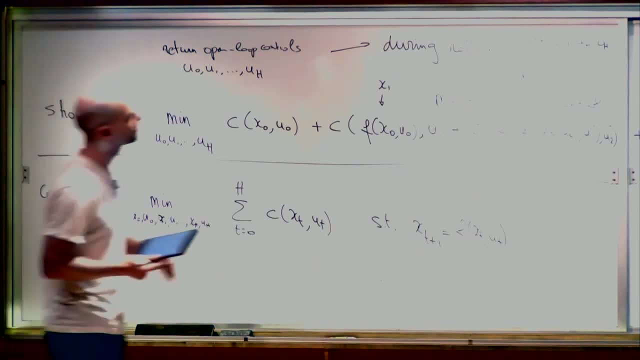 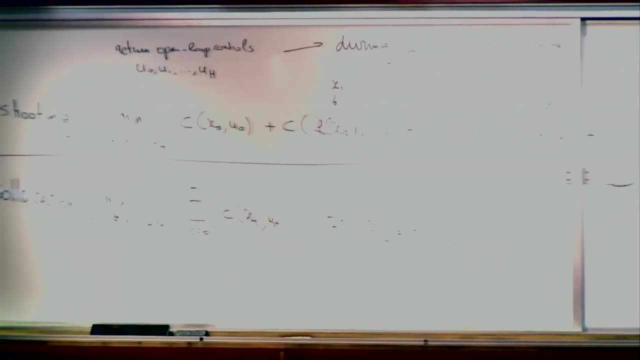 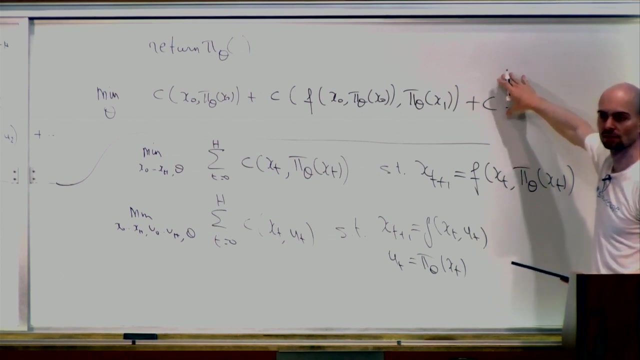 Where does that fall? Well, that falls over here. You're returning a sequence of linear feedback controllers, So returning a policy. We do it with a shooting method in LQR because you kind of roll out the current policy, see what happens, back-rubricate through all of that. 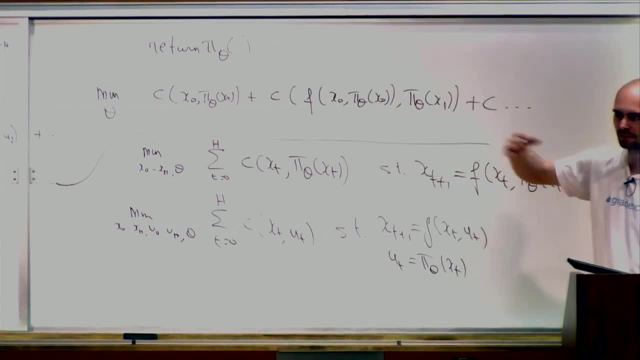 in a specific way, back-rubricating with value iteration, but it's a back-rubrication through everything to find an update and repeat. So iterative LQR falls here. It's kind of a you think of it as applying Newton's method. 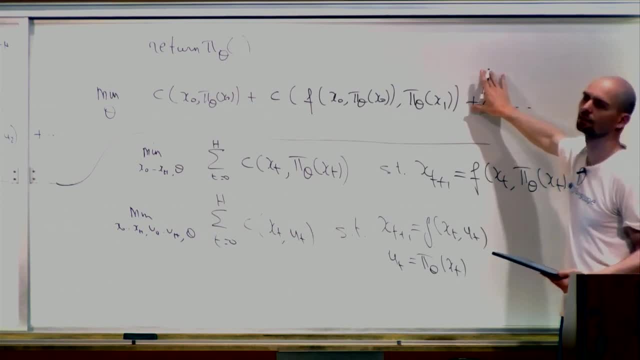 If you were to apply Newton's method here, you'd see that essentially it's gonna be or Gauss-Newton method. it's gonna be equivalent to LQR. it's just that LQR is structured in a way that it understands every part of the structure. 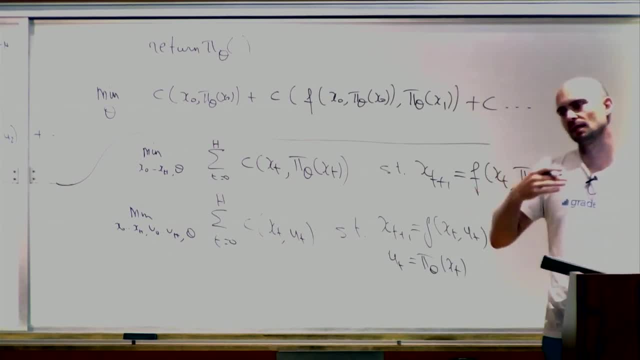 of the problem, and so it takes advantage of that in a way that if you just ran a black box Newton method, it probably would not be nearly as efficient in this spot for the same problem as the iterative LQR. Now, if you want more than a linear feedback controller, 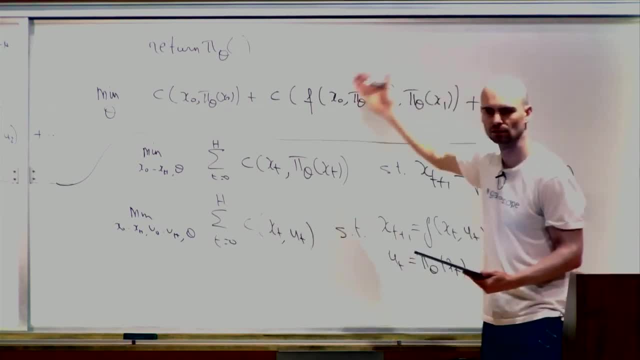 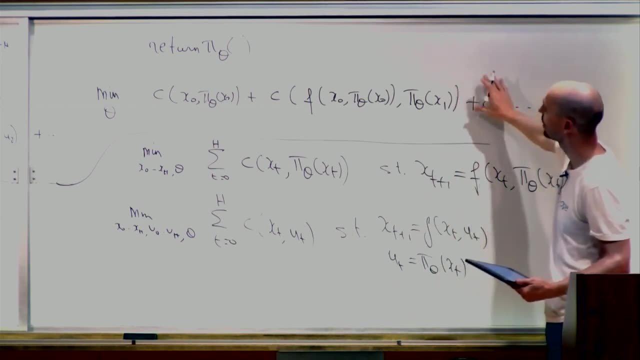 it gets trickier because LQR will not give you that. If you want a pi theta, that's a neural net, then you might still need to resort to just running Newton method on something like this, Or some people will run LQR first. 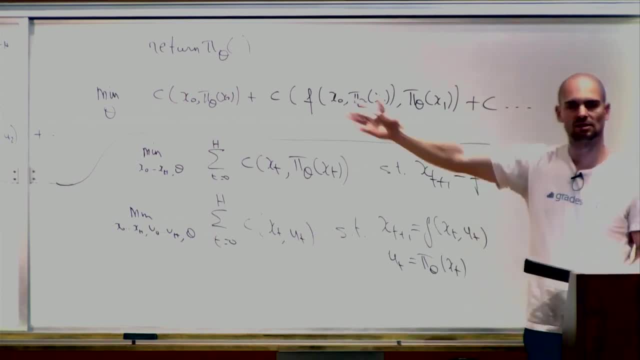 and then behaviorally clone it, say: okay, I now know my sequence of linear feedback controllers. now I'm gonna train a policy to be equivalent to those feedback controllers and find that policy that way. So let me show you. let's see. 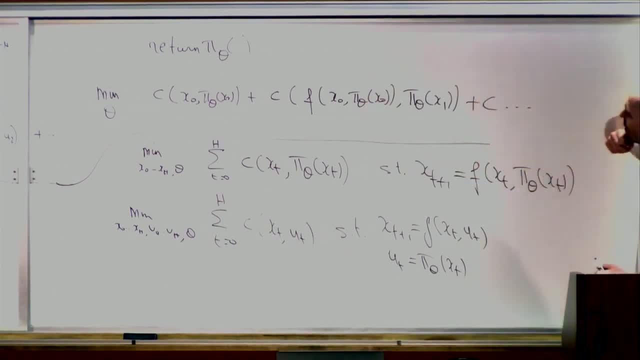 actually any questions about this breakdown. I realize it's a lot and it's kind of not always clear which option to choose, but that's just the reality of the situation, and what I mostly want is to make you aware that there is all these formulations. 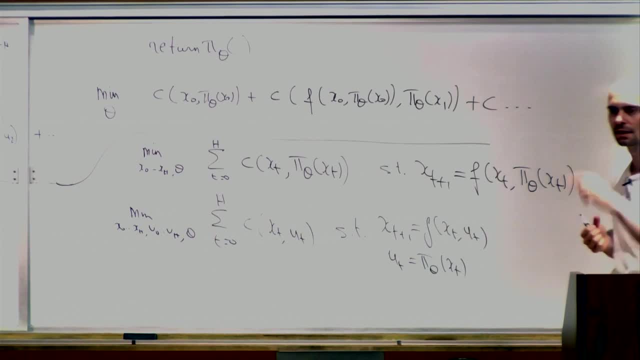 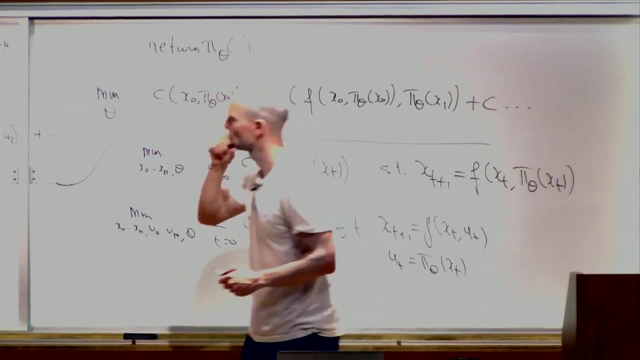 and you need to often carefully think for your problem which one you want to apply. yes, Can you limit how often the constituents are violated on the bottom left? one Like, let's say, I only want, oh, 5% of the time. 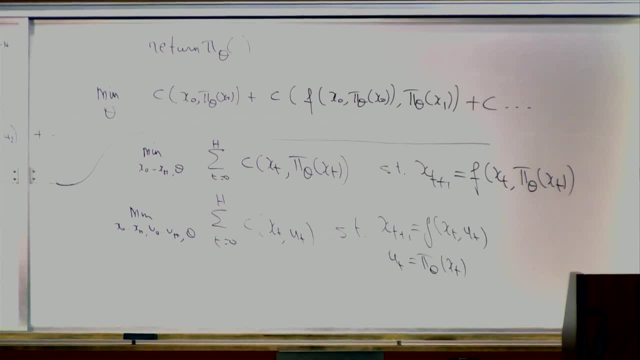 I don't care if it violates. So in your penalty method you could stop early if you want to, and then that's what you could have. You could- I mean you could- have an outer loop that says: if less than 5% is violated, I'm just gonna. 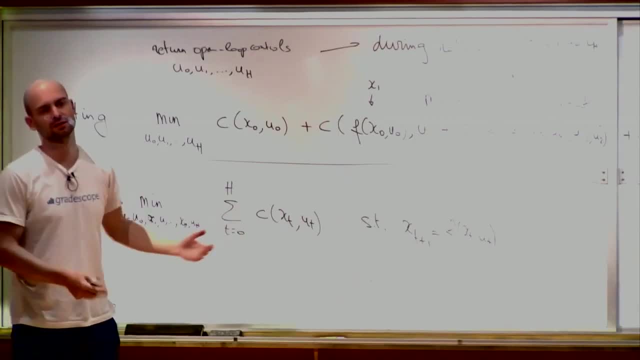 I'm just gonna run it and I'm gonna run an NPC mode anyway, and I hope it's good enough because the small violations won't affect me too much And that's a totally reasonable thing to do, Yes, When you're doing shooting. 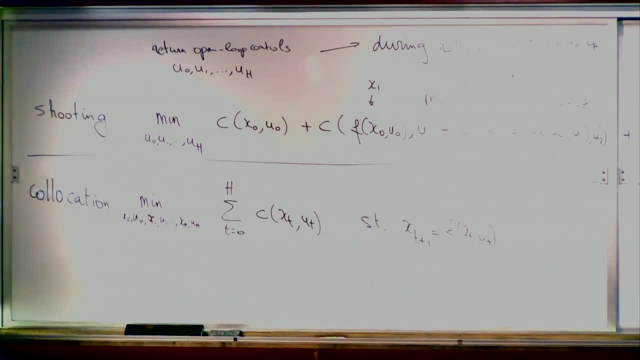 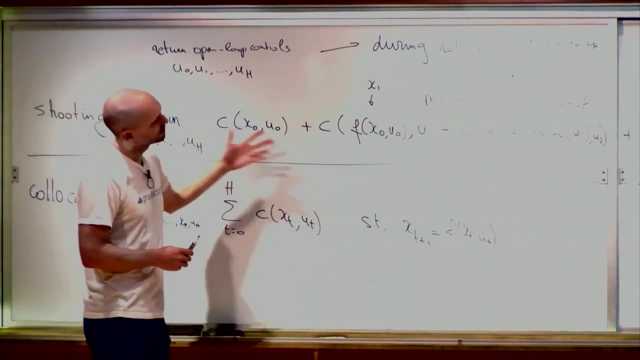 and you're calculating the forward task. do you actually have to physically execute that on the robot or is it just? That's a good question. So what I described here was assuming you have access to the real dynamics and you run it in simulation. 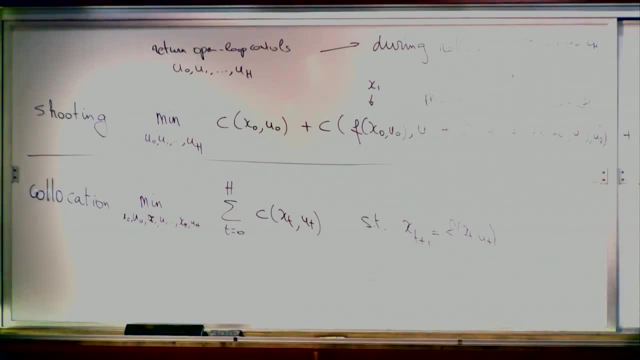 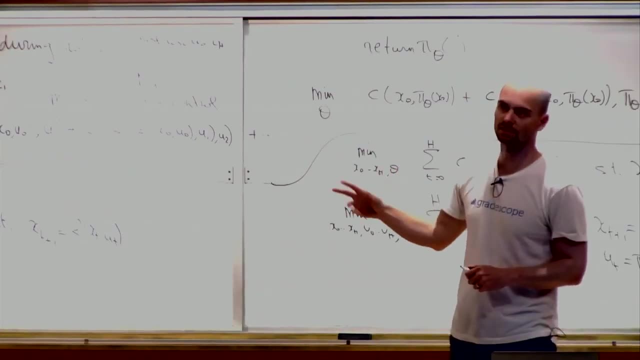 In practice. that's not always the case, but often you'll build a model that hopefully is close, and so when you actually roll out on the real robot, you'll see discrepancies and you'll definitely need NPC or a feedback policy to be able to succeed. 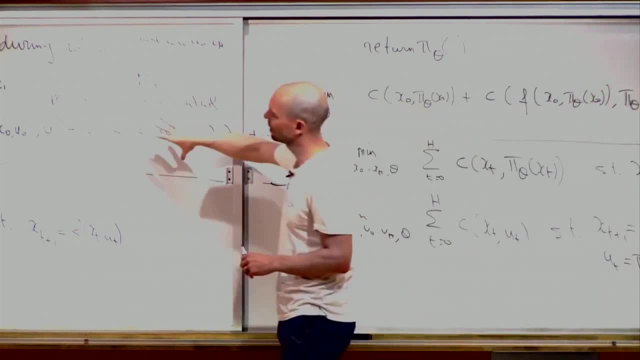 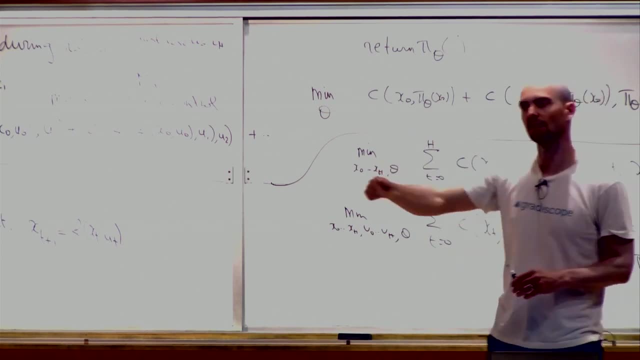 There's also the notion that you could, in principle, optimize for a while in simulation. then you do a rollout on the real robot and then you adjust your model F based on what you saw in that rollout, and at that point you'd be doing model-based RL. 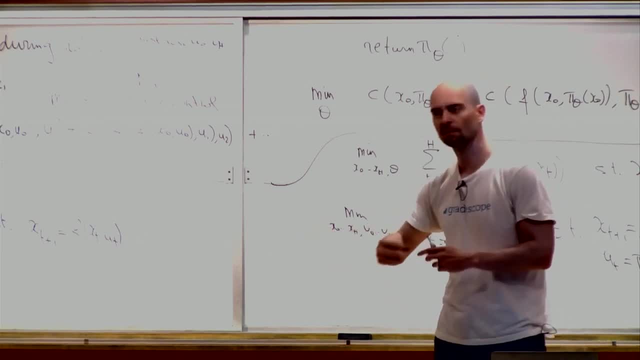 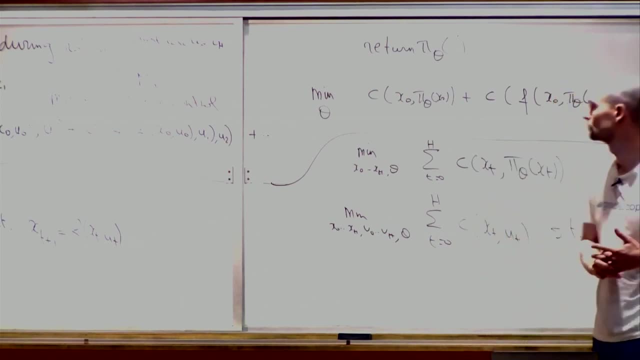 in some sense. but you adjust the model F and then optimize again against a new model and repeat: Yes, That's a small point, that the initial condition cannot be an optimization variable given. Yeah, correct, So we should start. yeah, good point. 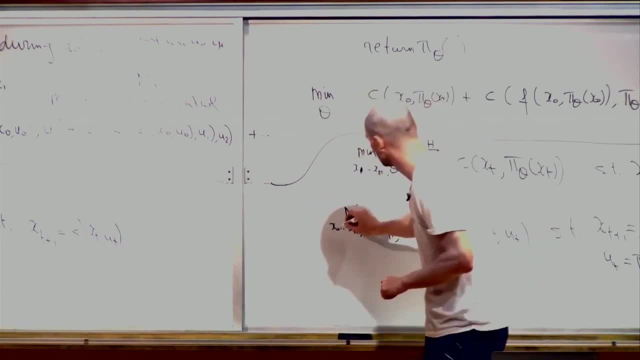 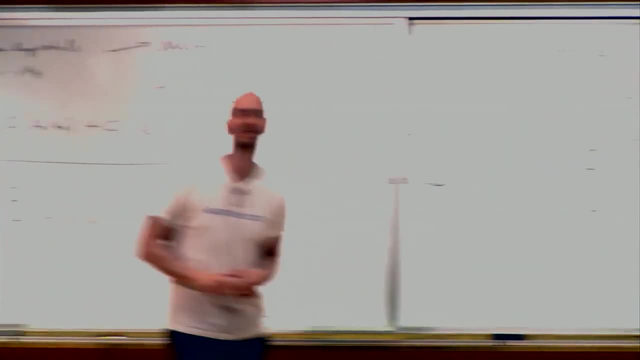 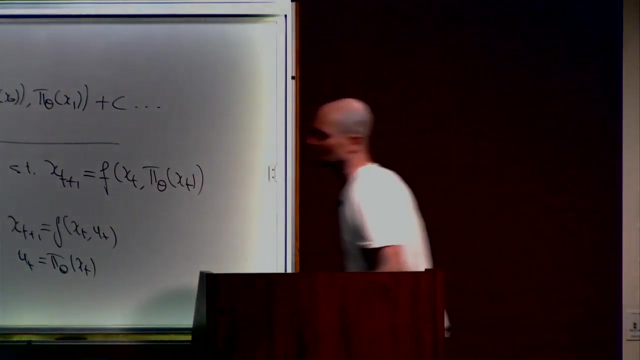 We should start in our optimization over X one, because X zero. we don't get to choose Absolutely right And the same here, Thanks, Okay, so let's recap this into the slides and then also look at a nice demo of a collocation method. 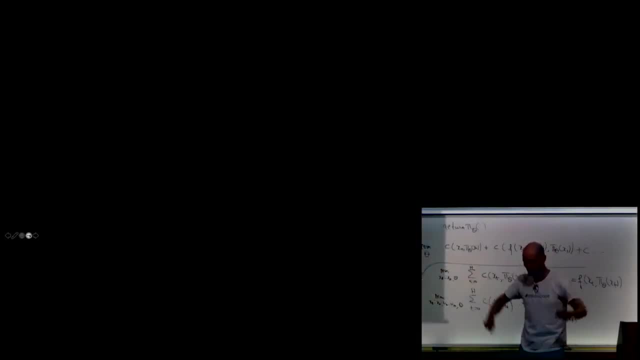 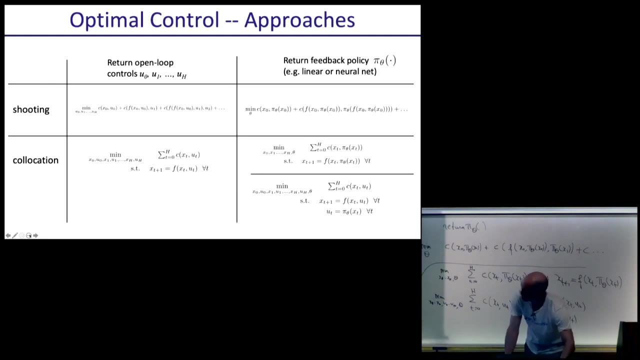 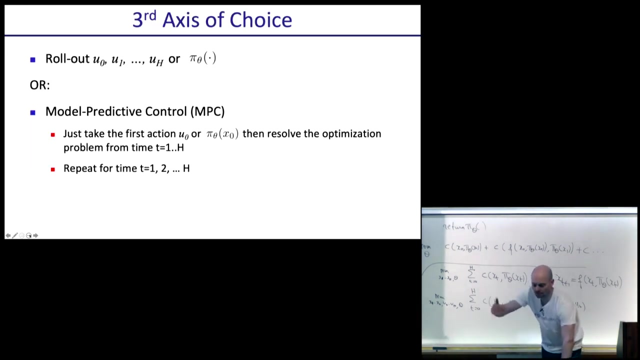 that has the exact behavior I described, just like make a car, follow a, find a path. So this is a table we ooh, wow, okay, This is a table we had on the board. The third axis of choice was whether to do NPC during. 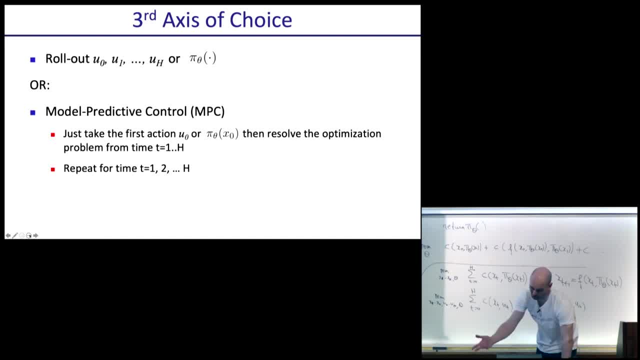 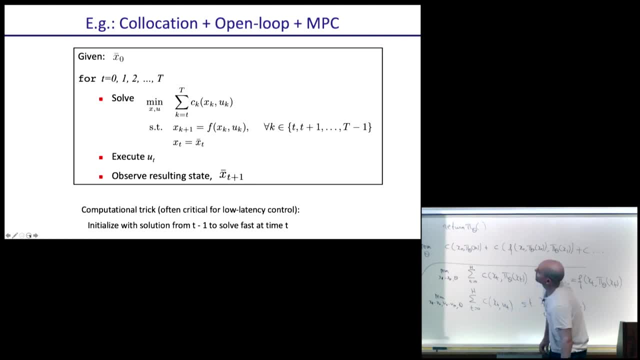 rollout or not, and when you optimize over just the use, you often will have to do it even during your optimization. Here's a specific incarnation of an algorithm. This is collocation plus open loop plus NPC. That's what's set up over here. 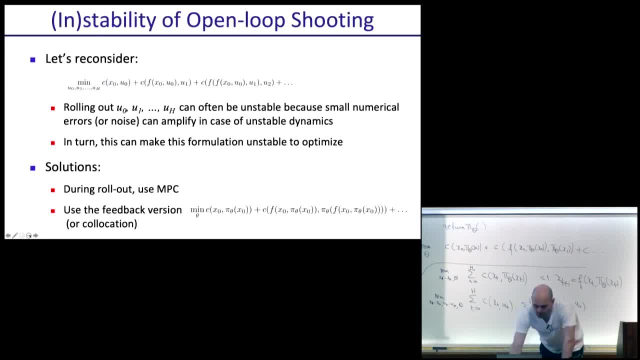 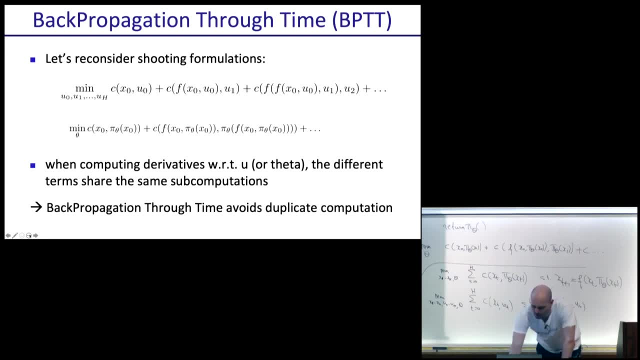 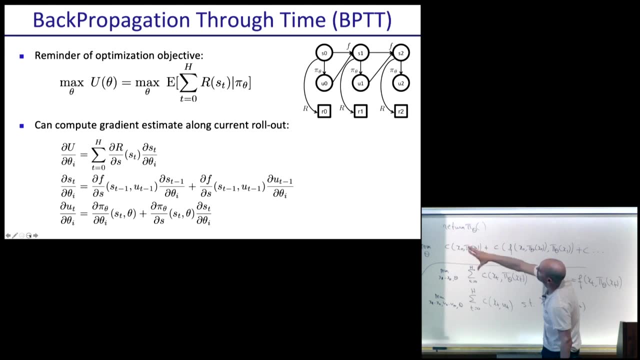 but you can do other things, of course. We've discussed the instability of open loop shooting. We discussed back variation through time being important to avoid duplicate computation. This is what it looks like in terms of equations. You would do a forward pass of your controls applied. 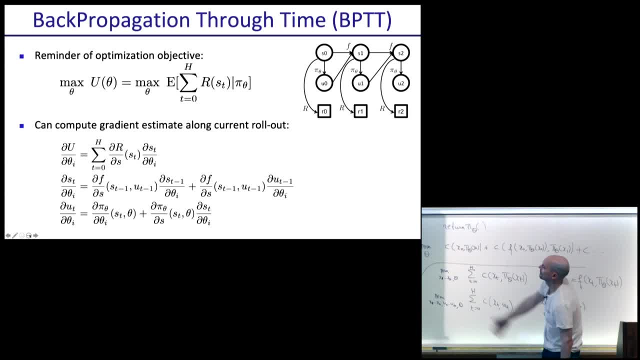 or your policy applied, and then you do, you'd have essentially these derivatives, which would be a backward chain of derivative calculations, to get out all your gradients, gradient entries that you need, And so it's not particularly expensive, It's just linear in the length of your sequence. 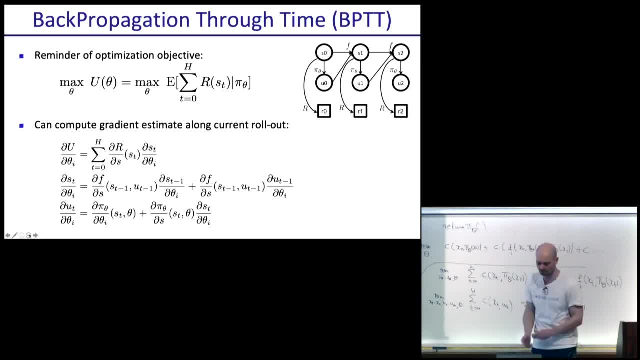 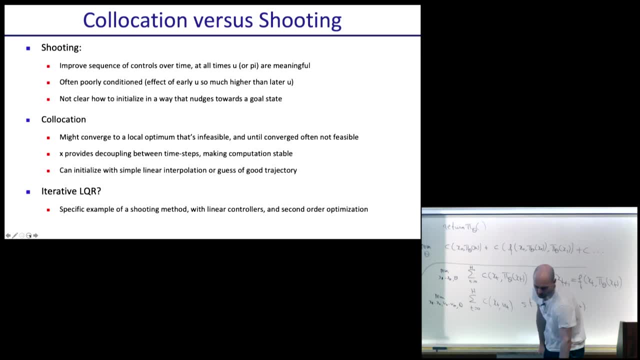 whereas if you do it super naively, you get something exponential in the length of your sequence. Then we talked about pros and cons of you know shooting and collocation and how iterative LQR fits in. Now look at something that I still find pretty magical. 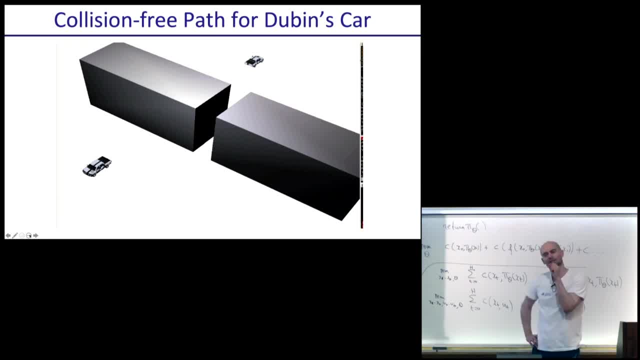 Here we're gonna do a collocation for finding a path for the car to go from bottom left to top right. then there's an obstacle. So the cost here is you have high cost if you're in collision with the obstacle and the dynamics is that you need to satisfy. 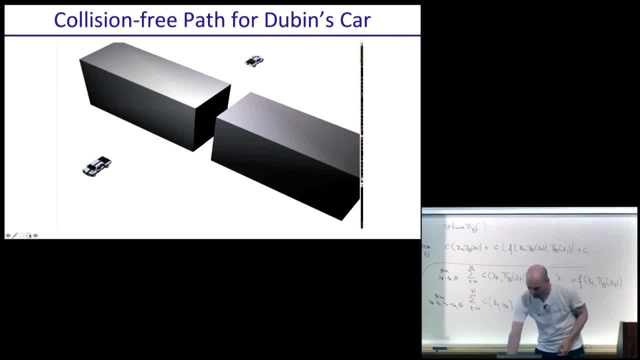 the dynamics of the car. If we run collocation we get to initialize. this is a linear interpolation between: so we kind of get a good hint at what we should have. It's gonna ride through the obstacle, but then there's cost associated with that. 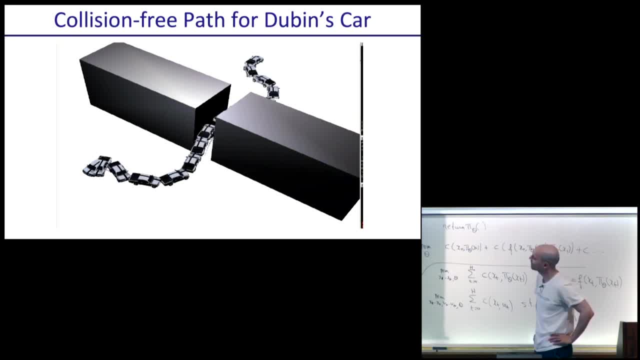 and there's a penalty for violating the dynamics, and over time it bends this path into a path the car can actually follow And this actually works surprisingly well in many, many domains where you can just watch it again. you can just bend your solution.